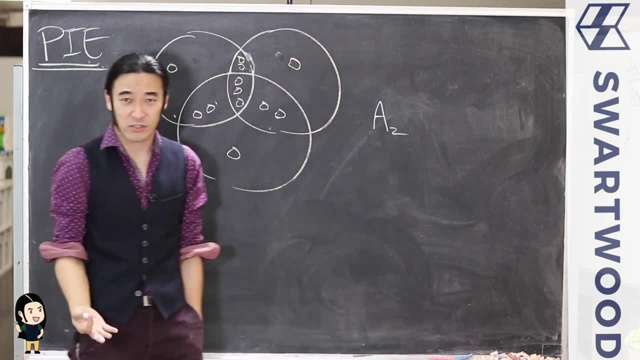 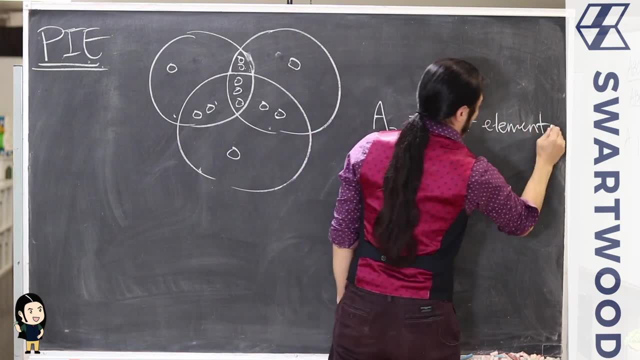 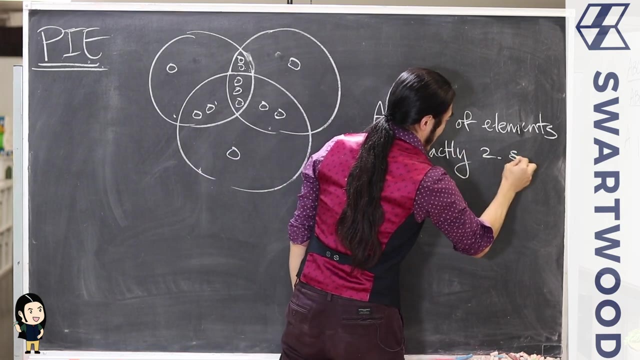 I'm going to call it, for example, like A2.. That's going to be my notation, So something like this: A2, it's going to be the number of elements in exactly two sets. So a lot of textbooks that talk about this. 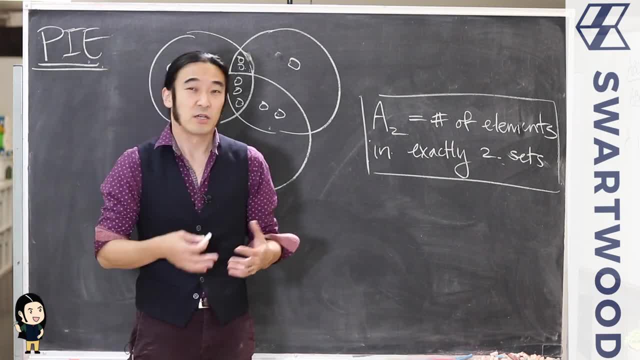 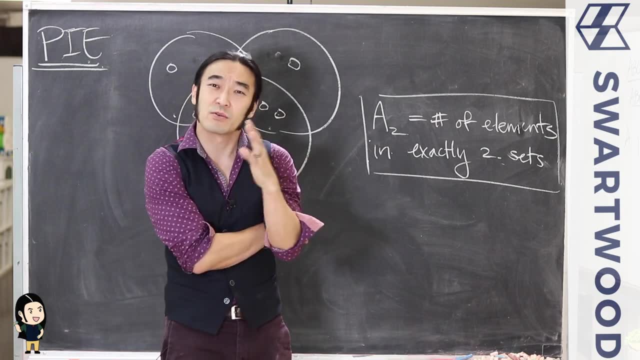 or they deal with this, generally talk about this in terms of properties. So it starts to become more abstracting. You think of properties, et cetera, et cetera. But you can think of it this way: Being or having a certain property. 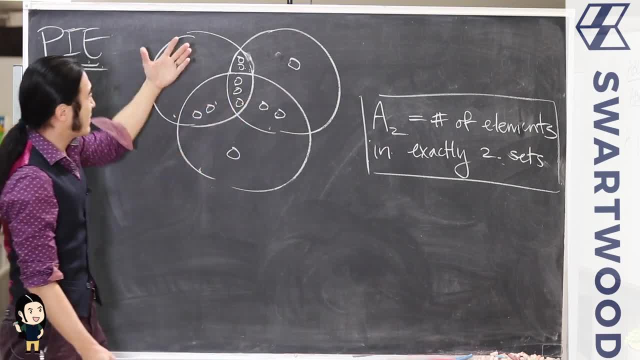 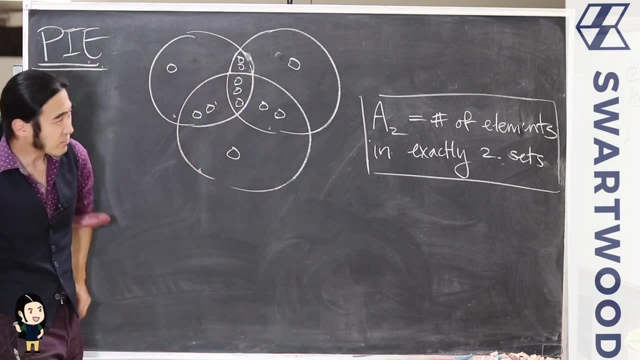 is basically equivalent to being in a set, So this could be like property one, property two, property three. So I'm just going to do this in terms of sets. No big deal, All right. So we need a little bit more notation too. 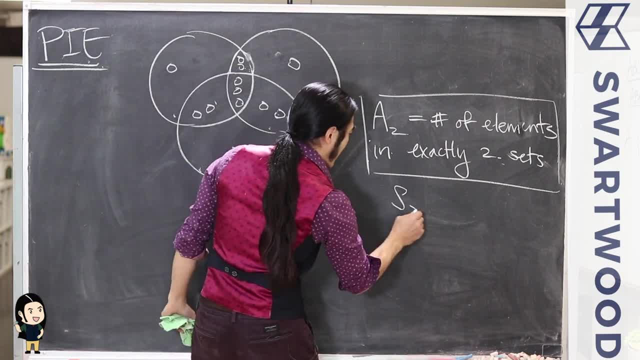 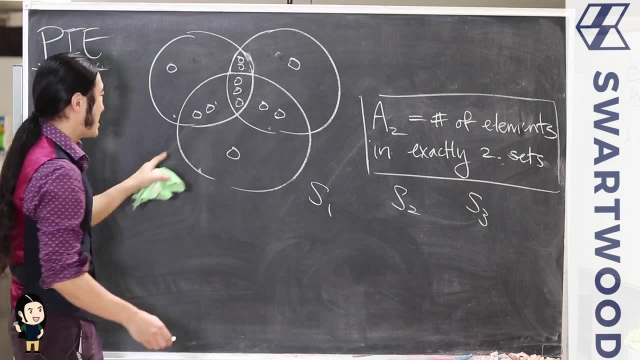 So I'm going to start using notation like this: S1, S2,, S3.. And let me show you why. So do you remember the regular principle of inclusion and exclusion for three sets? It kind of looked like this: The magnitude of A plus the magnitude of B. 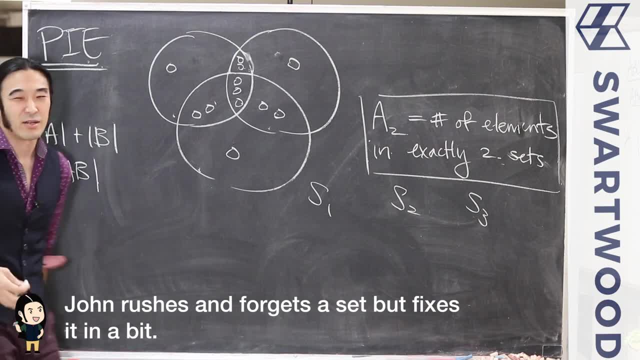 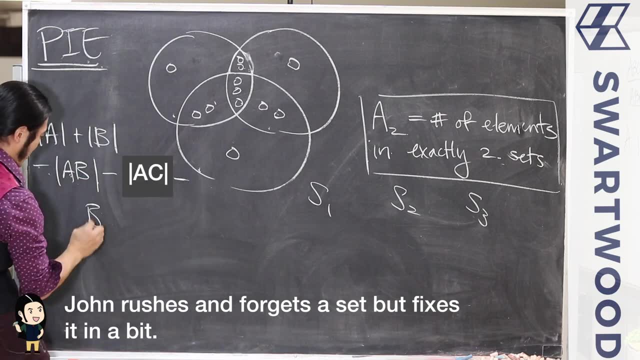 minus the magnitude of the. So when I say magnitude I really mean the size of the set. It's much shorthand: The intersection minus this intersection minus this intersection Right Plus this guy. Now I'm doing this pretty quickly, but I'm assuming you're comfortable with that previous video. 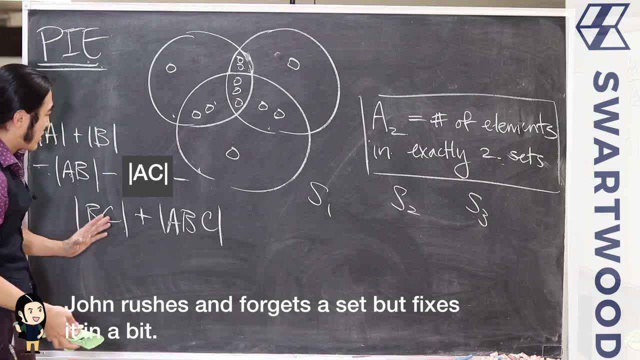 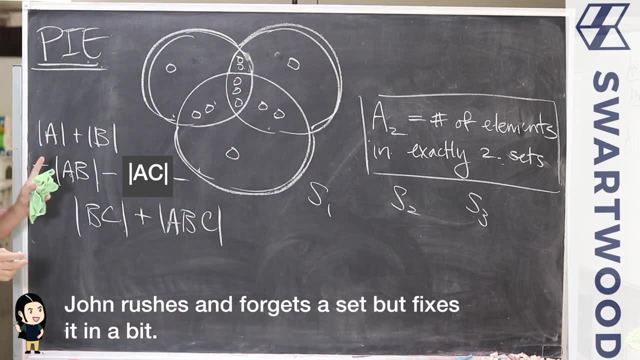 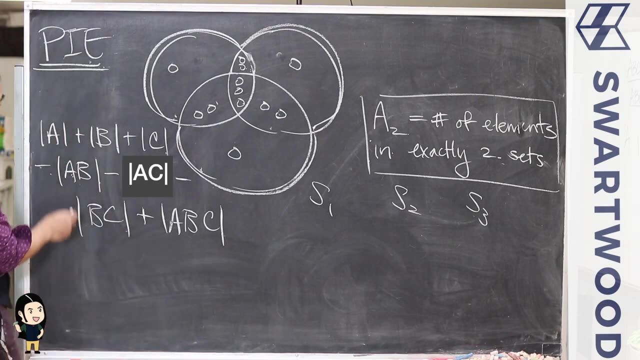 OK, So this thing right here was figuring out or computed all the guys that are in there, Right, OK, But the way we did it was we first. Oh, I'm on crack, There we go. OK, All right, So let's redo that. 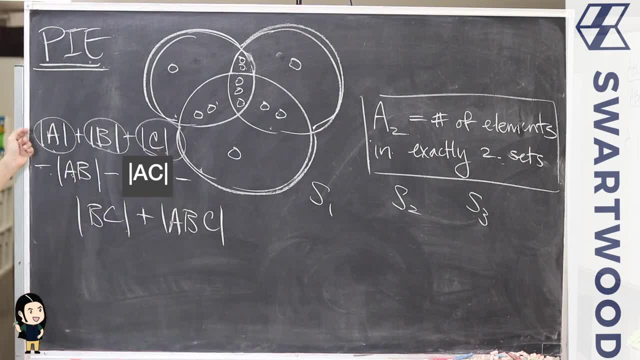 So notice here we added up the number of guys in each set Right. So A plus B plus C, We'll call this S1.. So this entire sum OK. And then notice here we added up well, excluding the negative sign. 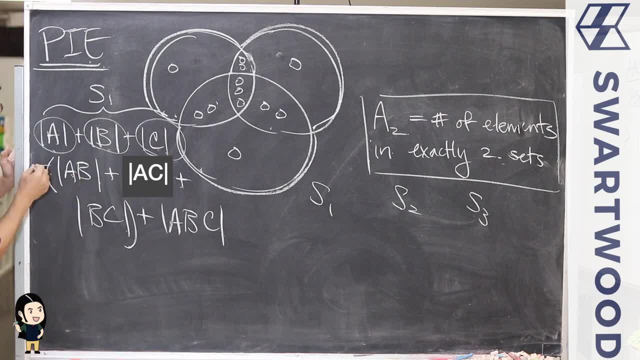 Let's write it like this, Right? So we subtract this guy and this guy and that guy, So we're subtracting the sum of all the double intersections, so we'll call that S2.. OK, And then here there's only one guy. 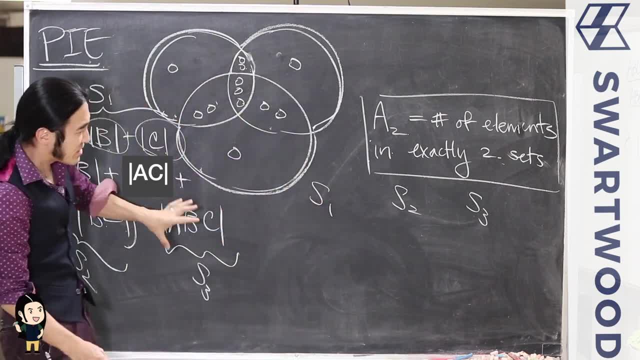 but you can imagine, if there were more triple intersections we'd sum them all up With this sort of notation. it's going to be much more efficient, especially for the formula that comes with this guy, rather than writing them all out, OK. 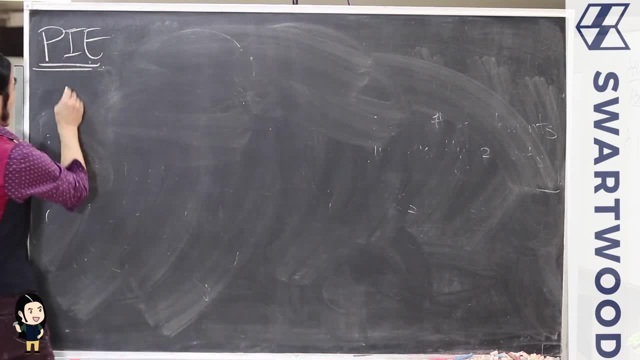 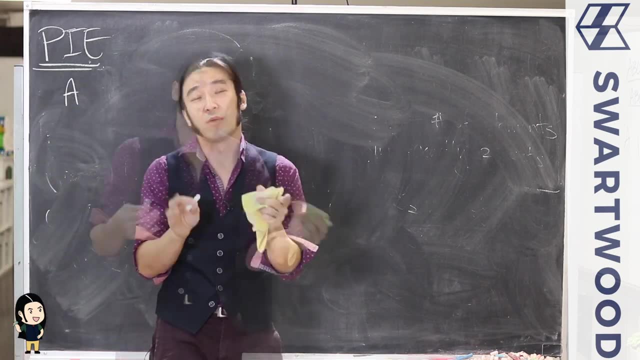 What we want is we want something like this. So, in general, if we have like a bunch of sets right, some of them intersecting, some of them not, blah blah blah, You want a number of guys in the union of all those sets. 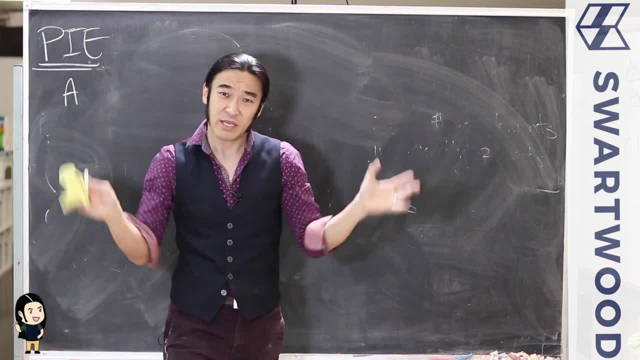 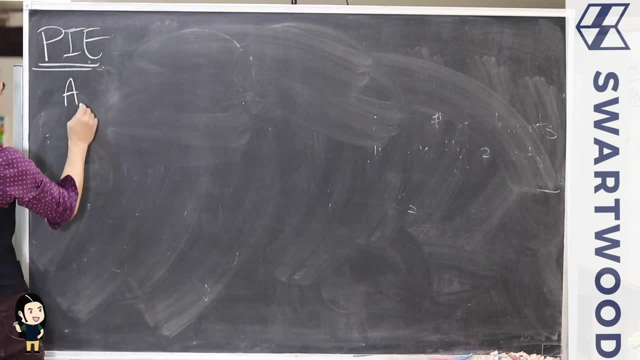 You'd use regular old pi and there's nothing wrong with that. So let's say, you have that big union, right, And now you want to know the number of guys where each guy's in exactly two sets. OK, So for example, 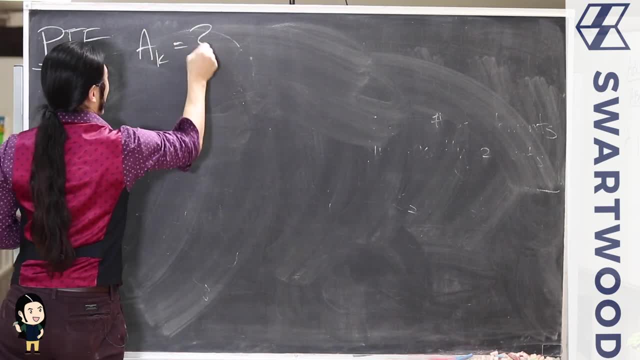 A2.. OK, Now, of course, in general, we're going to go for a formula for AK And you can look up the formula and use it and apply it. That's great, But the point of this is to basically give you. 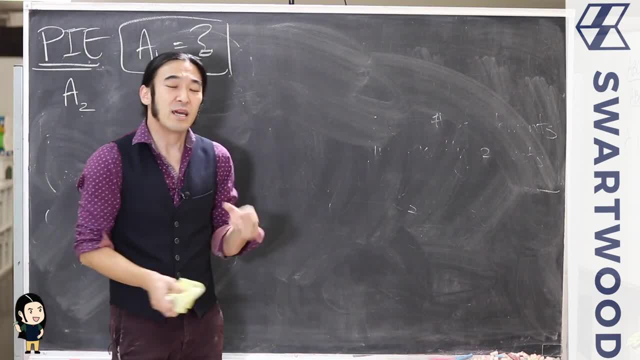 the intuition behind this guy, the proof of this guy, like where it comes from right, And I think what's going to be a little different here is we're going to talk about like motivation. So if you're just sitting around on your own, 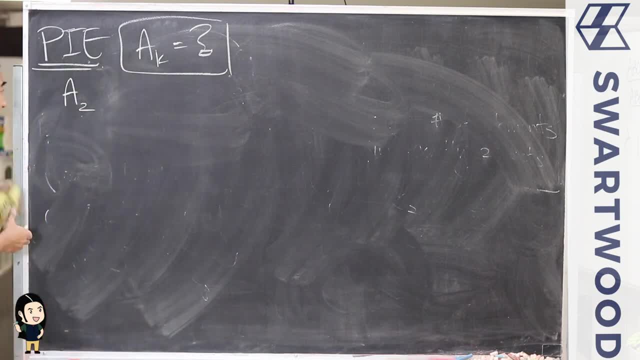 like: how could you come up with this? OK, So again, you might want to try it on your own. come up with your own way of doing it. I just wanted to share this because we had a request and I think it's kind of. 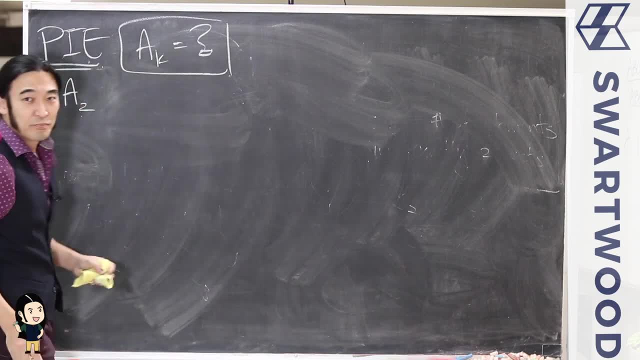 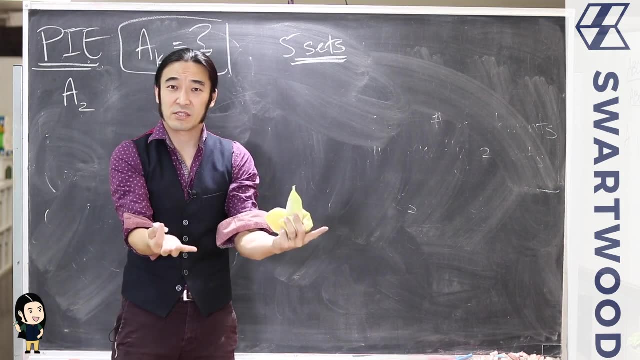 you know interesting to talk about. So let's try it with this though: Let's say you have five sets. OK, And we're looking at the union of five sets. OK. And let's say, aside from that, we have 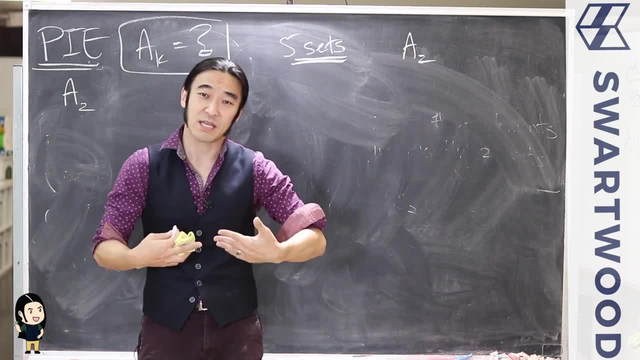 well, we want to look at a two, which is the number of elements that are in exactly two sets. OK, So again, it doesn't have to be the same two sets. So if we had five guys that look like this: 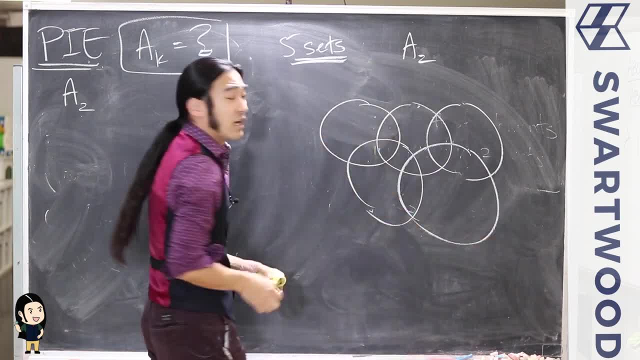 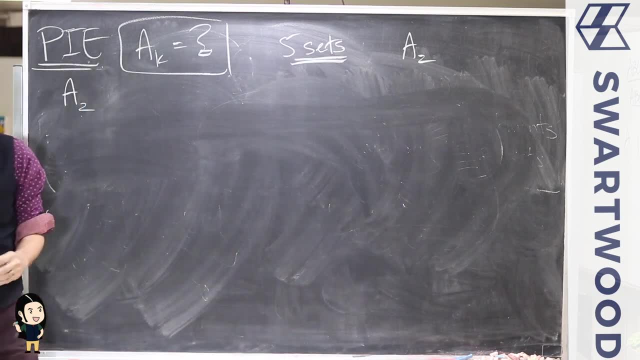 one, two, maybe three here, four and like five. right, We want the guys that are staying here exactly in two sets, exactly in two sets, All right. So let's try this intuitively Well, first, 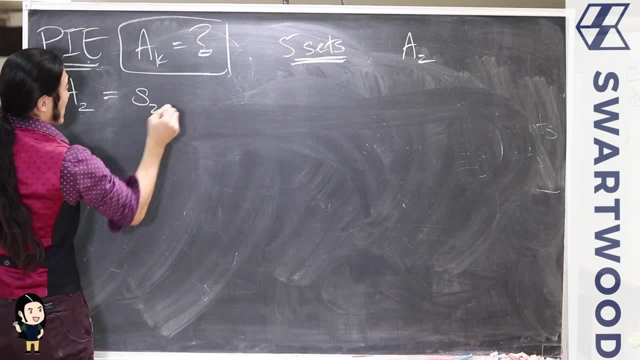 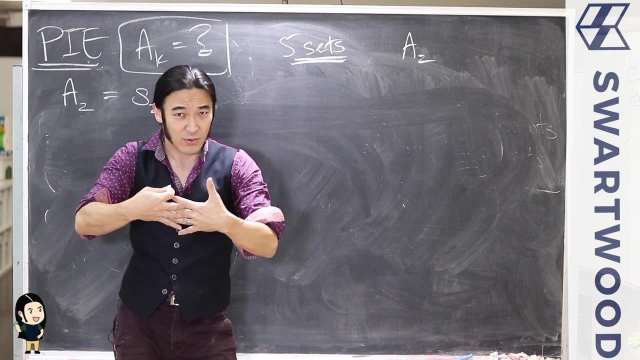 my gut instinct would be like we do with the general principle of exclusion. Let's just sum up all the double intersections. We're not going to start with S1, because we're looking for guys that are exactly an intersection of two sets right. 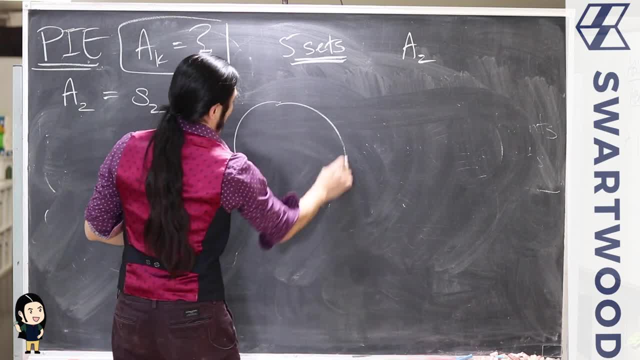 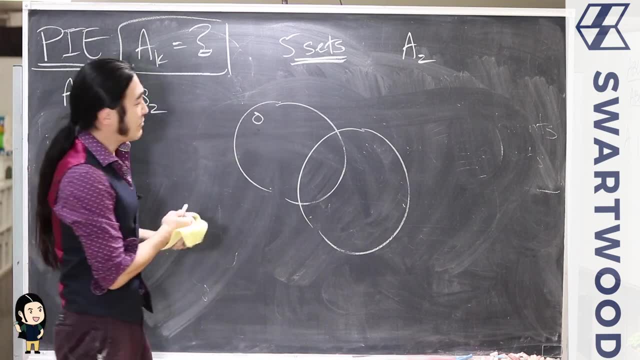 So there's no point in counting guys that are just in, you know, like like here, Right? So we're going to ignore that. So we're going to ignore where we count guys that are in one set, OK, Plus. 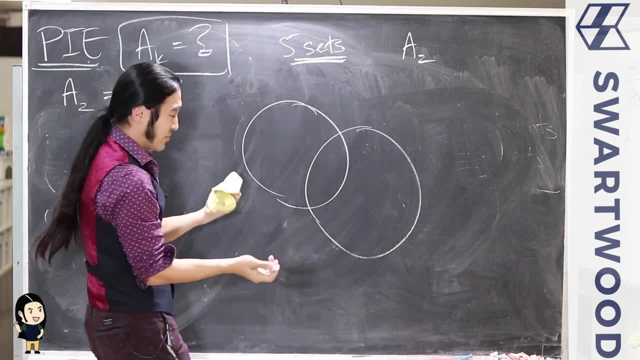 it adds a little bit more complexity because technically, when you do S1, if you have a guy- I don't know why I just erased it right there- right, Then you're going to count him once for this set, right? 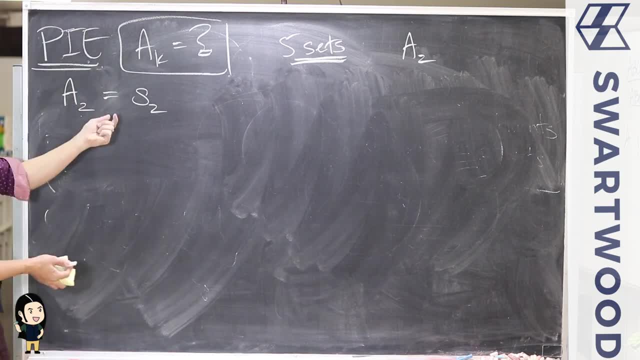 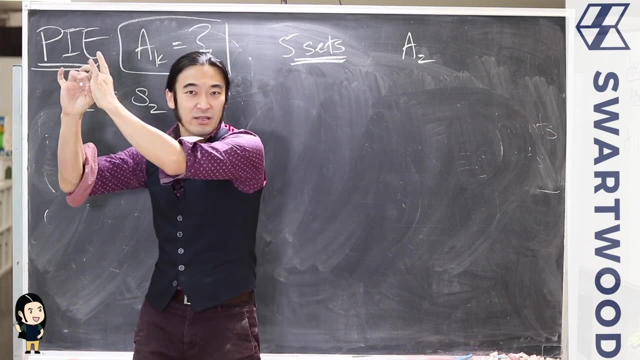 So I think it's just much simpler if we start off by just looking at the guys that are literally in the intersection of two sets And if that's all you had, if you just had like something like this and maybe over here. 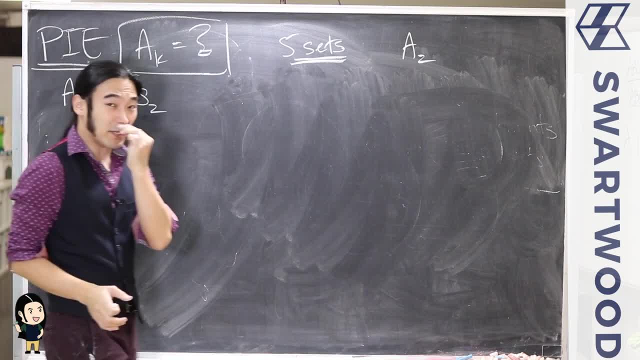 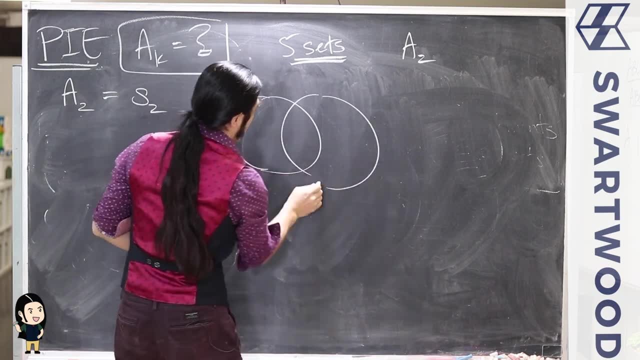 something like that, something like that. you can just compute this number and you'd be done. The problem is is that if you have guys that are in triple intersections then, like we saw before, elements here are totally fine, But guys that are in 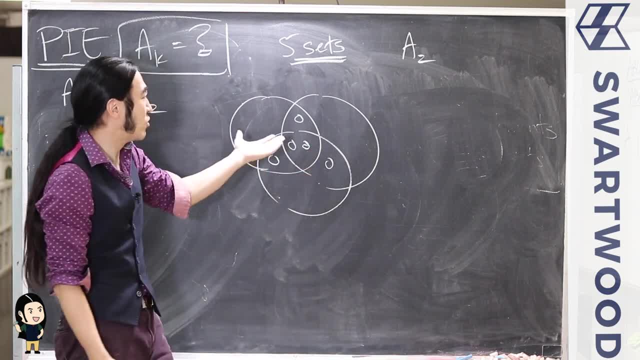 the triple intersection, they're going to be over-counted. The other thing is that we don't want to count guys in the triple intersection. Remember that We want them to be exactly in two sets, But anything in the triple intersection would be exactly. 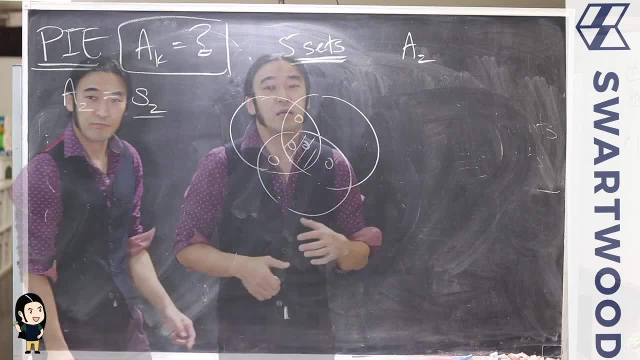 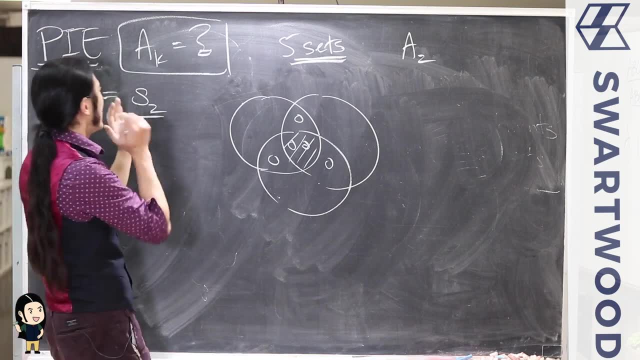 in three, right. But at this point it might be a little confusing because you might be thinking: doesn't this count the number of guys that are in double intersections? Yeah, it does. But remember this is literally: you take any intersection. 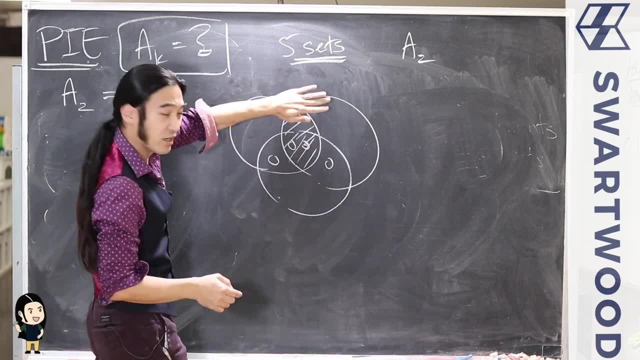 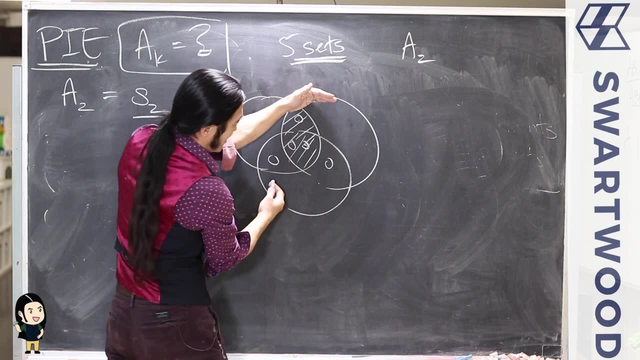 between two guys, which includes all of this region, So everything in here, And you literally add them up. So for this and this, you would count one, two, three. But then for this and this, you would count one, two. 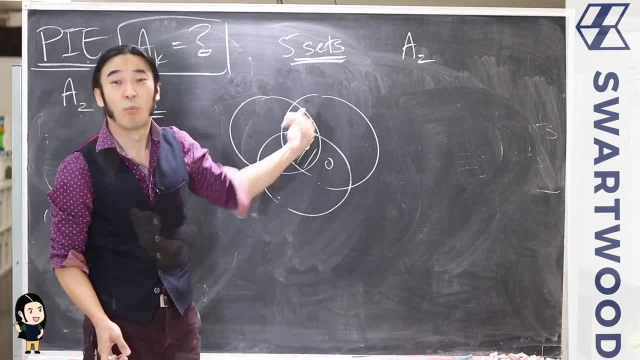 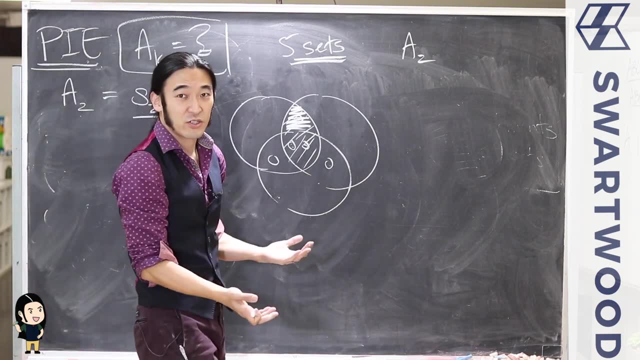 three. So it doesn't give you exactly the number in double intersections, It just gives you double intersections or more. It doesn't give you the guys that are just purely in double intersections like this. It gives you guys that are in any sort of double intersection. 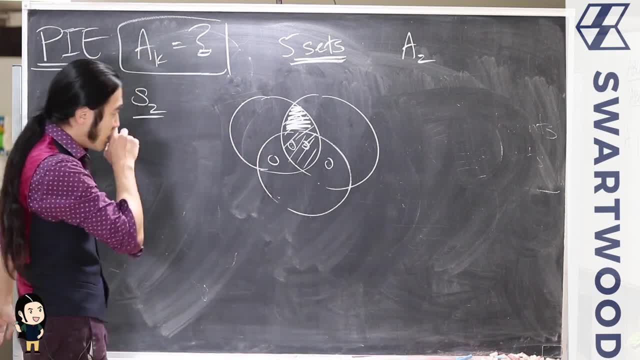 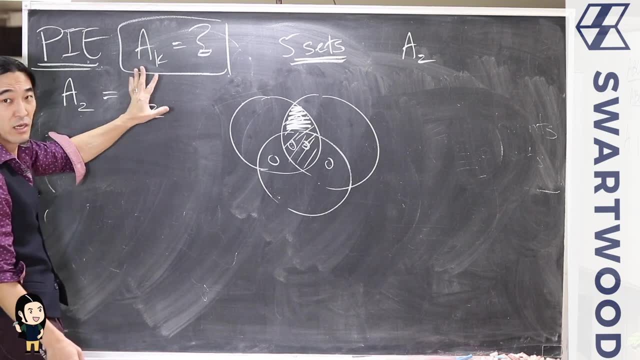 whether that includes guys that are also in triple intersections, quadruple intersections, quintuple, et cetera, et cetera. So counting guys like this, which are definitely in here, are not so good, So we want to fix it. 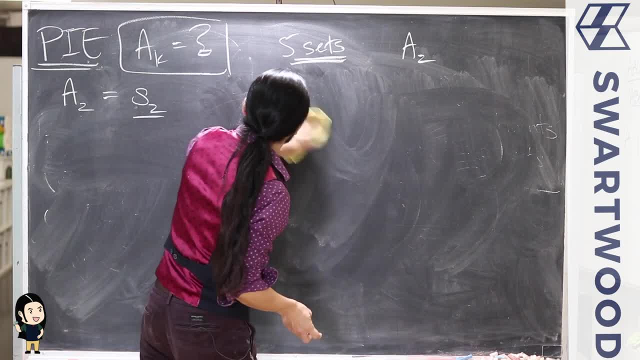 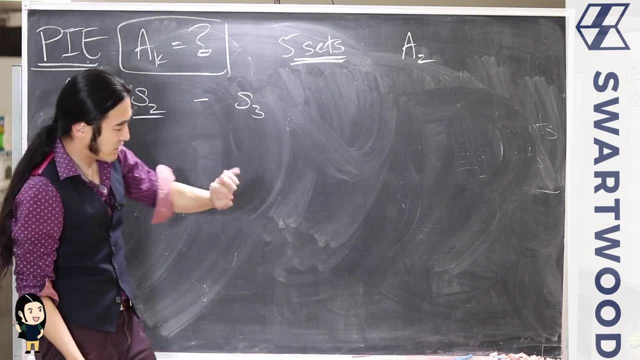 right. So I think one natural thing to do would, be kind of like before, take out all the guys that are in triple intersections, So this guy counts guys that are in triple intersections or possibly higher intersections, And if you count, compute this guy. 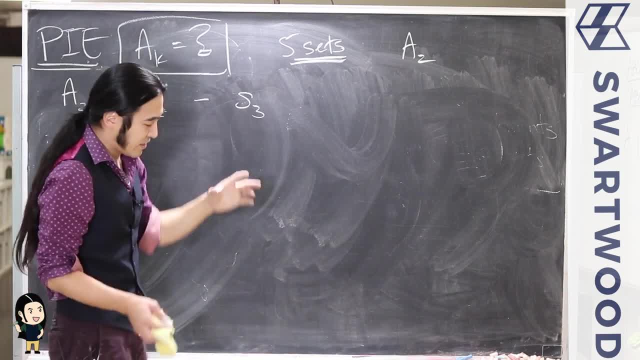 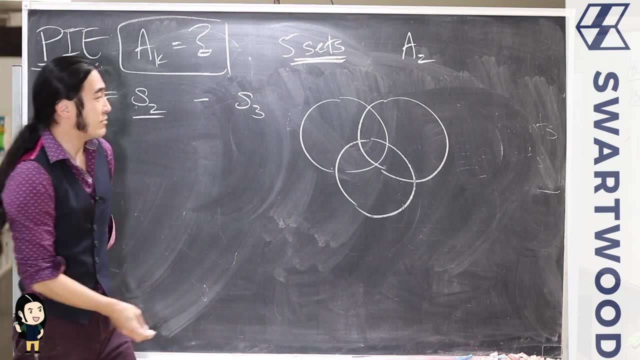 you take this guy, subtract out this guy, then you're removing, at least in this case, all the guys that are in issue. Okay, All right. So let's see. So, for example, if we had one here and two there, 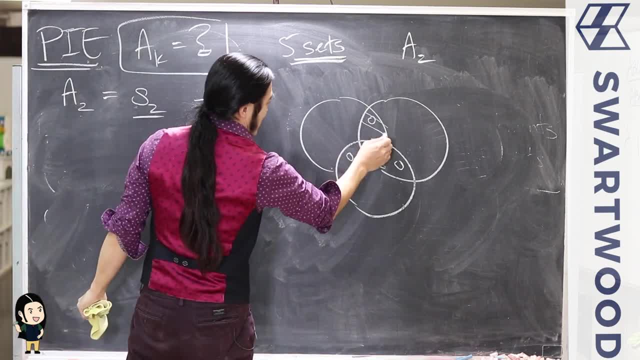 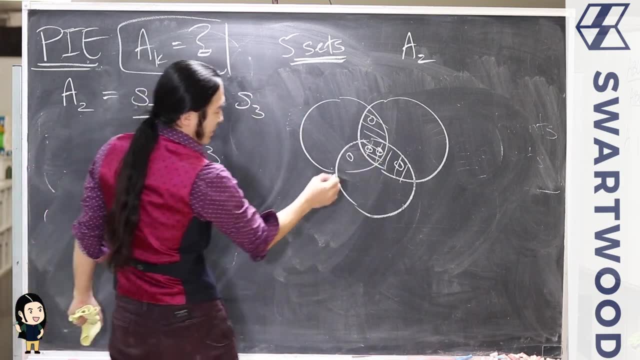 what does this guy count? This guy counts, say, this intersection one time, So to count three, And then it would count this one. So it would count three, And then it would count this one. Okay, Which would count three. 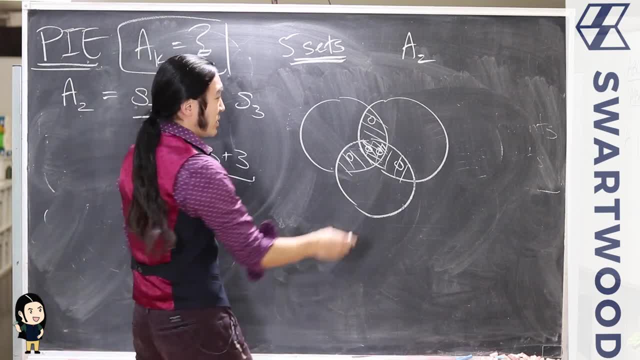 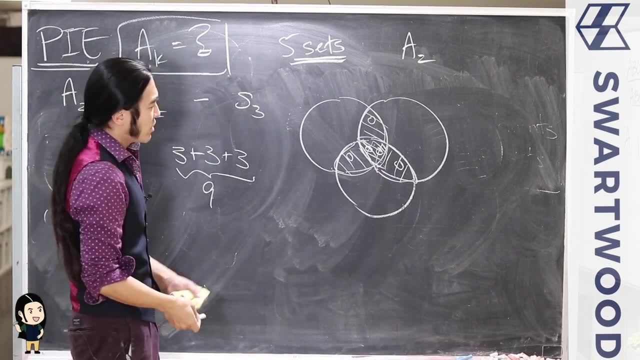 And we'd have nine. Okay, It's clearly not what we want, because we know that we want this, this and this And that's going to be three, Okay. So I think if we subtracted this off, we'd be in a better place. 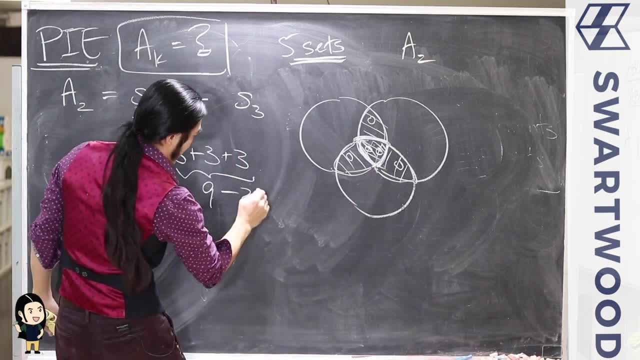 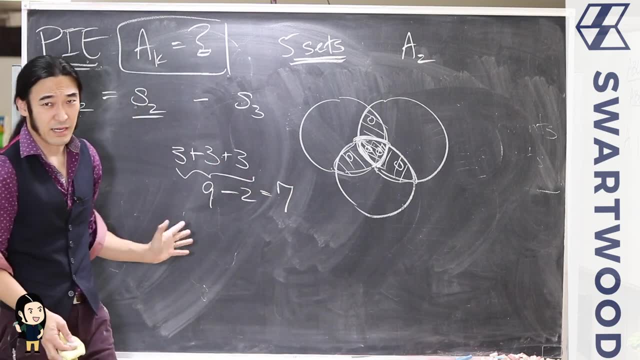 So we subtract the guys in the triple intersections, So we subtract off two Right, And then we've gotten almost what we want. Well, at least better Seven's closer to three than nine is Okay. So what was the problem here? 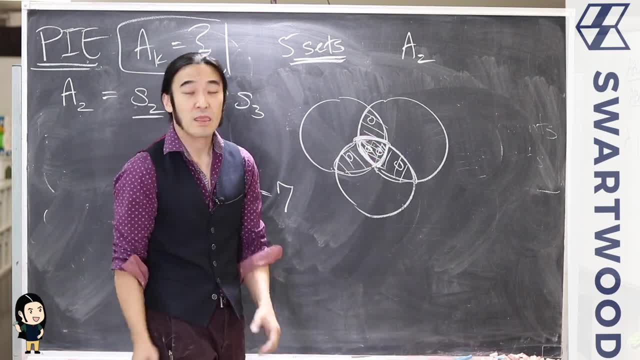 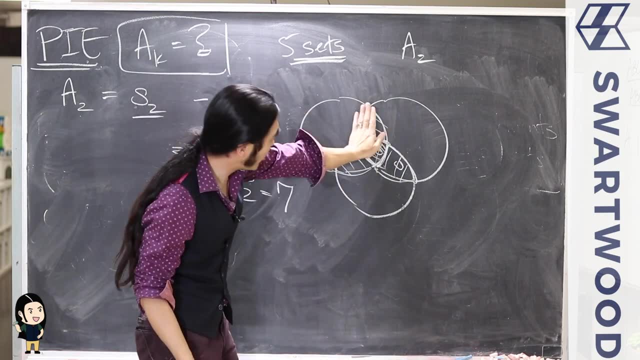 Remember, there are two issues going on. Number one: you don't want guys in the triple intersection to count. But number two: every time you were adding up the double intersections, you counted this guy. You didn't count him just once. 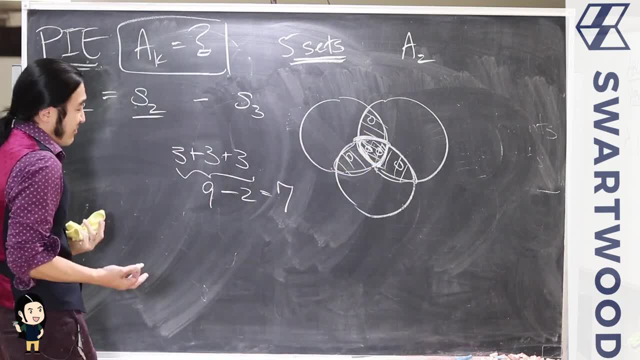 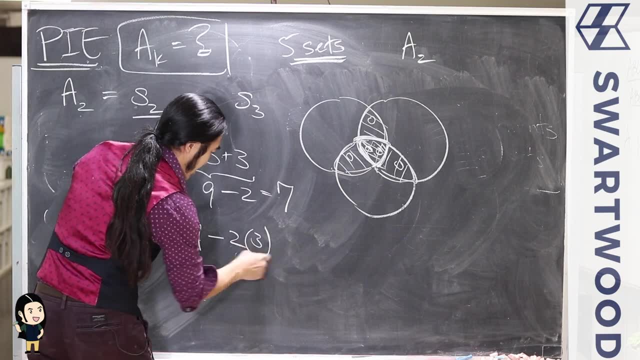 You counted him one, two, three times. Okay, If we take that nine and we subtract off this overcount of two, but how many times did we overcount this guy Three times? So then that would be nine minus six, That is three. 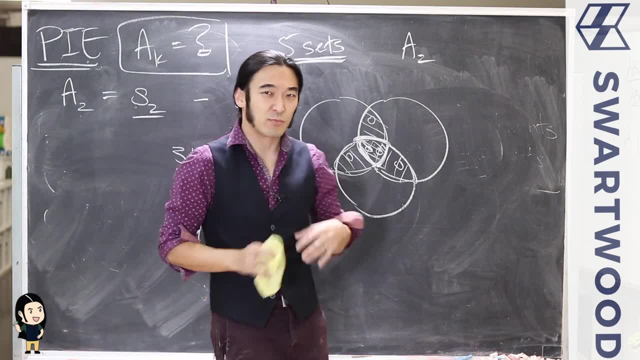 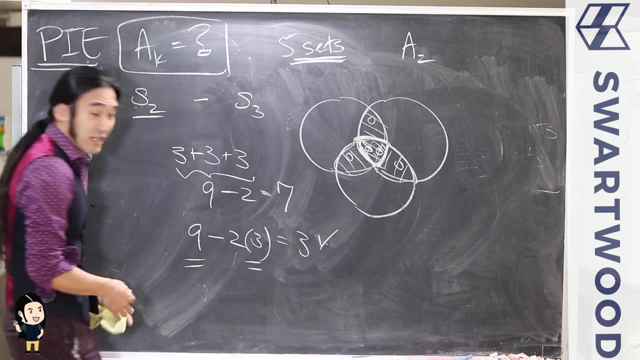 That is what we want. So that's roughly the idea. So you're playing with this and you're like, okay, I get it. You take the double intersection type guys that sum S2,, you subtract off S3, at least in this simple case. 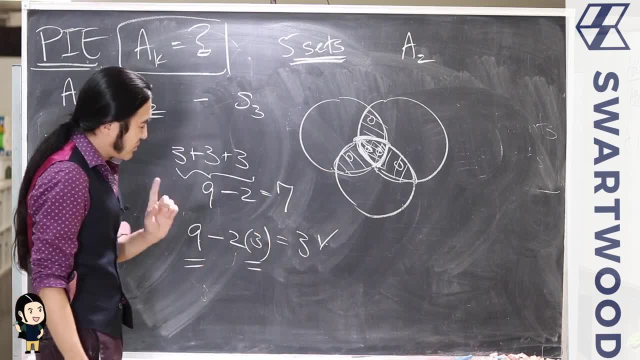 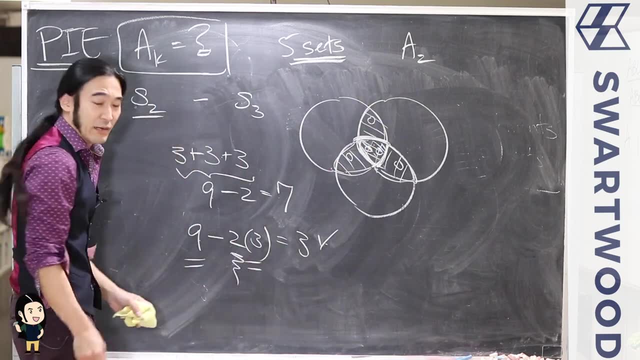 and we can kind of see the pattern's got the right idea. There are two problems with this Number one is: every time you're counting this, you're counting this too many times, So we've got to have some factor in front to compensate. 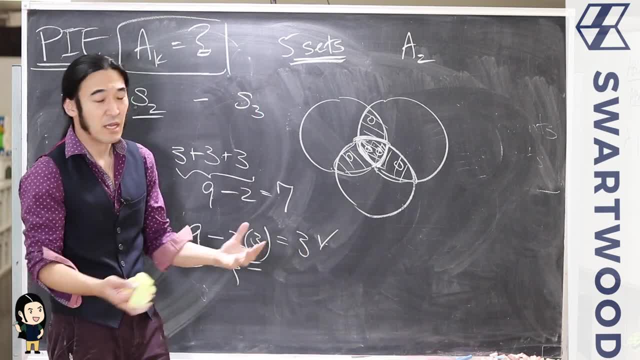 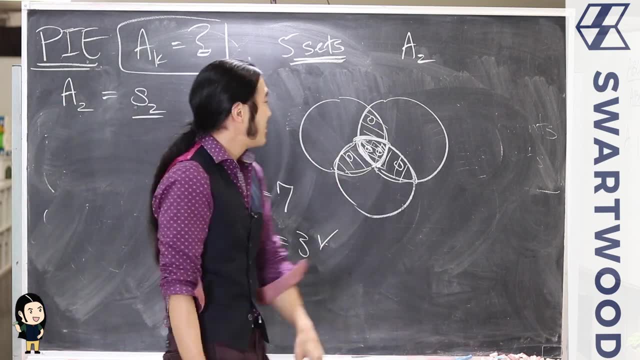 In this case it's not that bad. It might get slightly more complicated with more sets right. The other issue that we're kind of forgetting here is what if there was a quadruple intersection Right, Just like when you're doing regular pi? 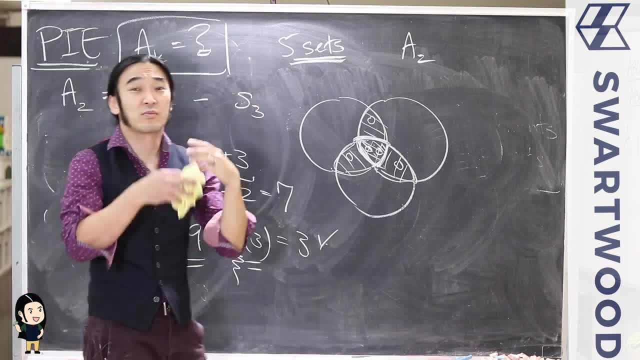 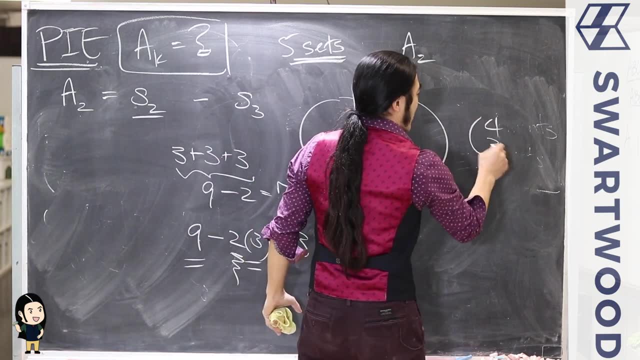 then it's kind of like we're kind of overestimating the number of triples in a way, right, Because with every quadruple you have a bunch of triples that would come from that quadruple. When four sets intersect, right, you'd have four sets out there. 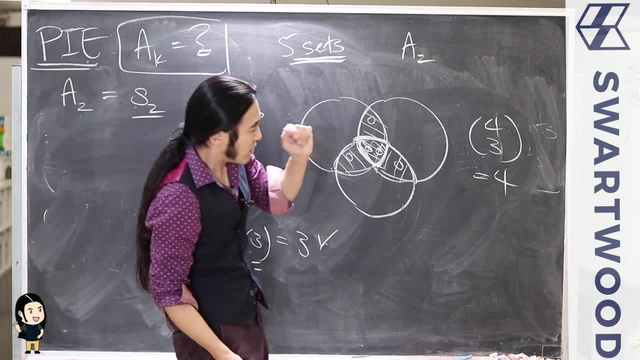 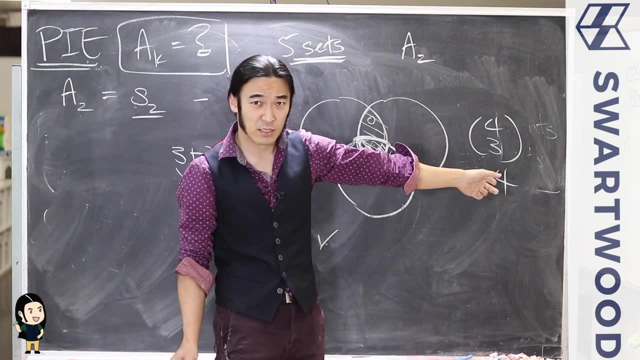 There are four. choose three or four ways to count triplets. So when you have a quadruple intersection, any element in the quadruple intersection is effectively counted. if you count by triplets four times, Okay, Don't worry about that, We'll go through it. 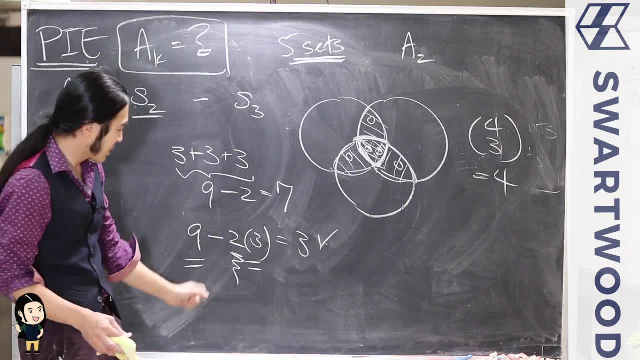 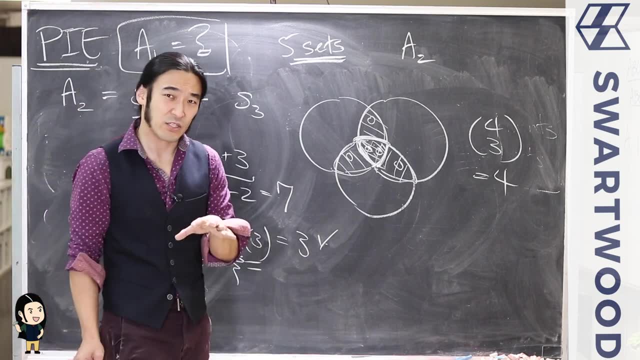 more slowly. I just want to outline this idea. You've got two issues going on. Number one: we want to correct S2 by taking out S3, but we're kind of overcounting, so we need to fix that. The second issue is: 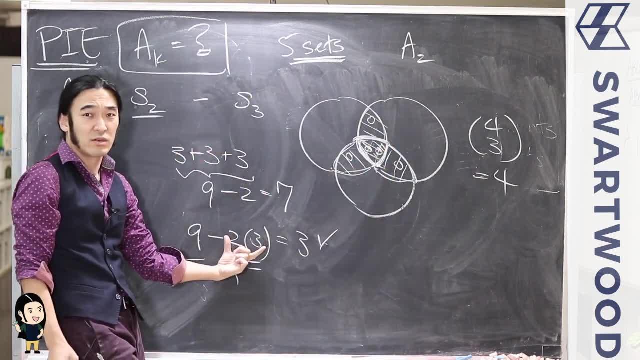 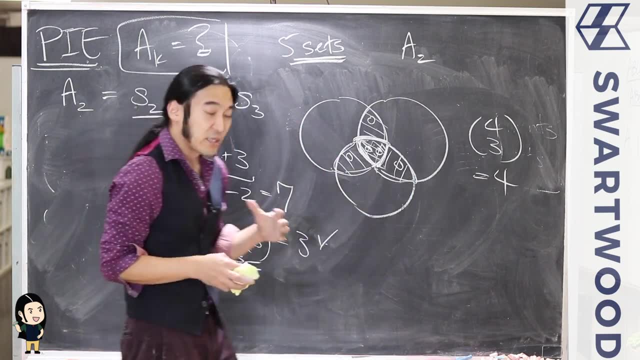 if you had greater intersections, then maybe this estimate is also sort of overdoing it, right? So we compensate by adding back. You subtract from pi, You subtract, You add, You subtract, You add. Okay, We can keep progressing forward like this. 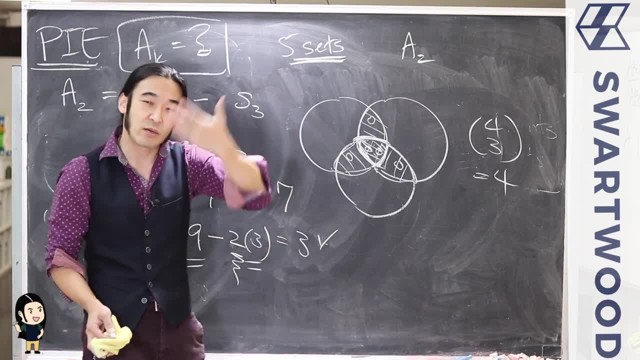 but it gets kind of tricky. The other thing is sometimes what people do when they prove this stuff is they start with the formula. You start with the formula and then you try to prove why it's true, And that's okay, It's not too bad. 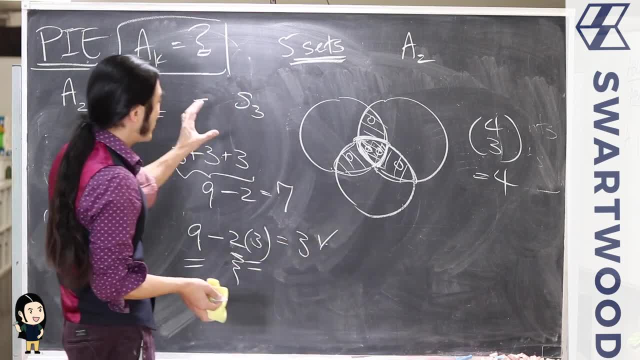 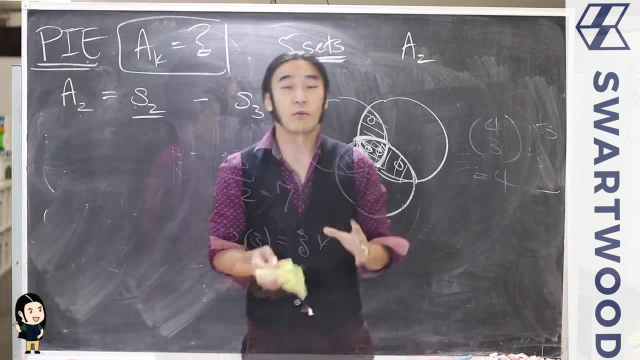 But the thing is, I think, at least for me- the idea would be like: where would you come up with this to begin with? I personally think that's more important. I mean, it's great to prove it once you have it. 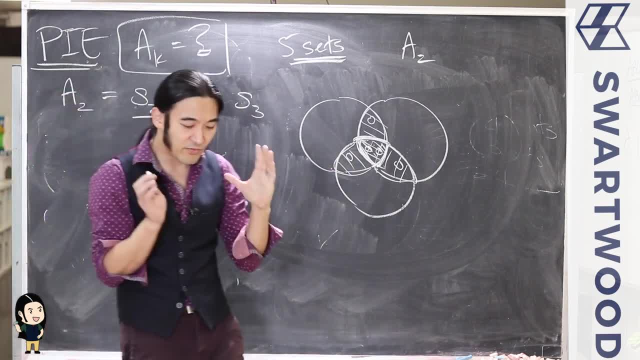 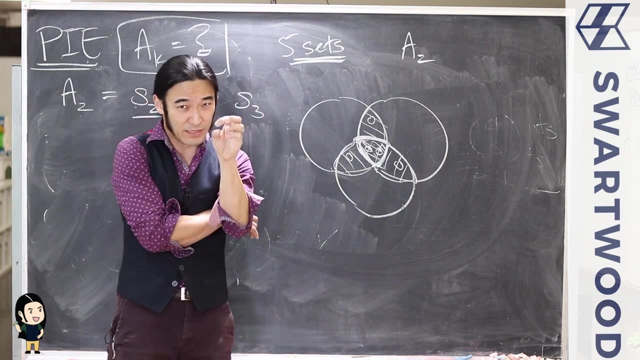 and that's super significant and it's completely the same thing with this understanding, but I just want to focus on what we're counting, Okay, So if we have a guy that's only in a double intersection, like an individual element, that's only in. 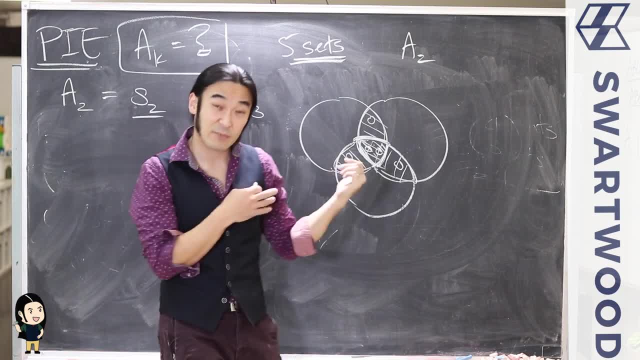 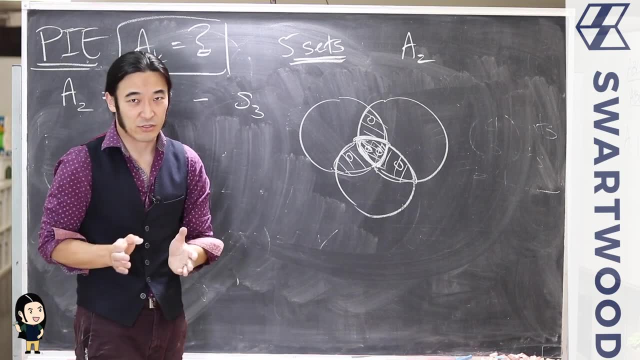 a double intersection. he's counted here, He's just fine. The problem arises when, for example, in the previous case, you've got a guy that's in a triple intersection and because of that he appears in multiple double intersections. 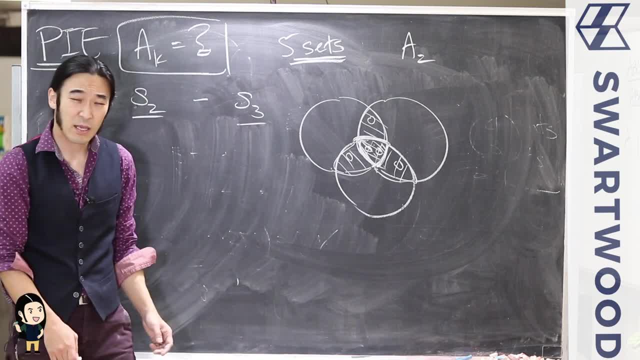 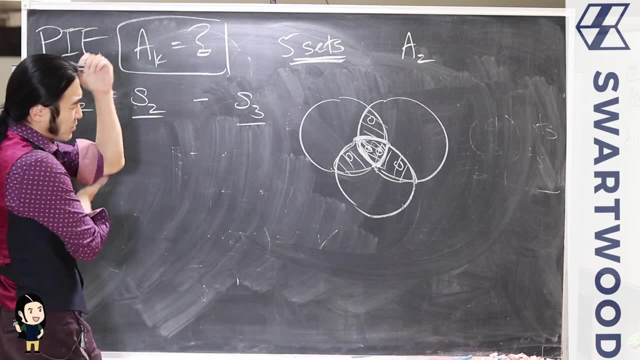 right. So that's why we're going to try to adjust by taking out that triple right. But like you saw here, pi is counted multiple times. Does everybody see that? Okay, So what's a way of sort of fixing this? 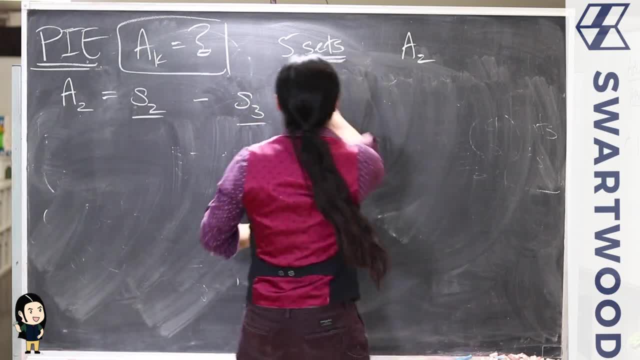 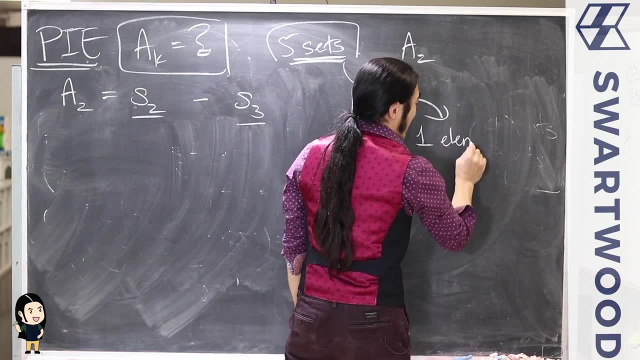 Why don't we visualize it like this: Take any element, Actually, first, let's do it five sets, okay, And do you agree? we're going to pick out one element. So we saw that in the proof of pi, right? 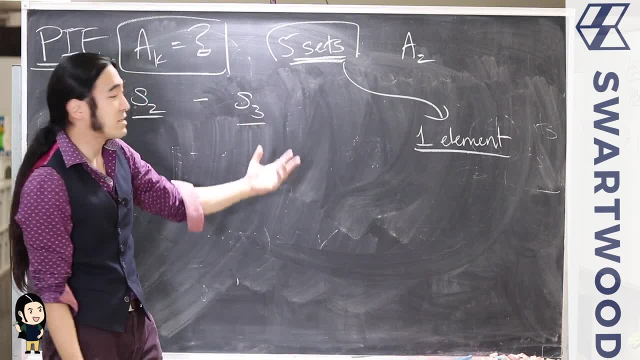 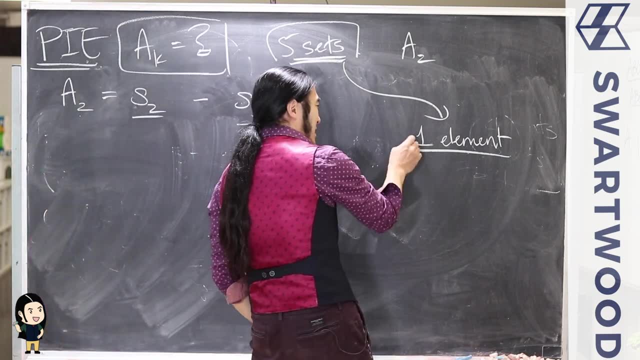 You can focus on one element to make the argument simpler. So we're going to think about what's happening with one element. Now we need to place him somewhere. But just to make a point, let's make this guy in the intersection of four sets exactly. 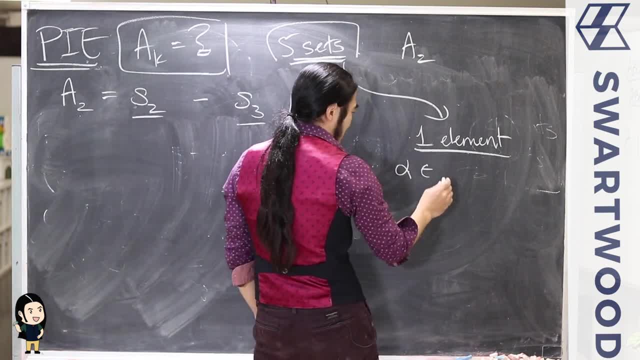 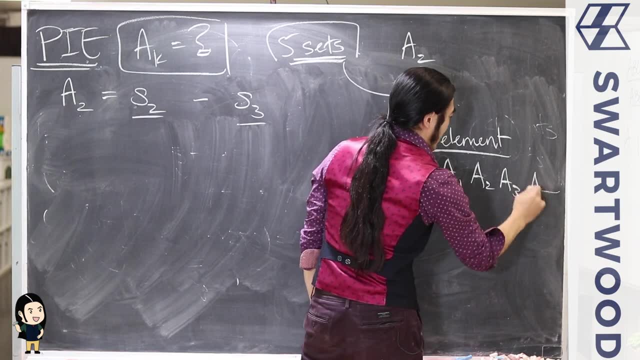 So let's make this one element. Let's call it alpha, Let's say it's in the intersection. Well, let's do this. Let's say there's a1,, a2,, a3,, a4, and a5 will be the final guy. 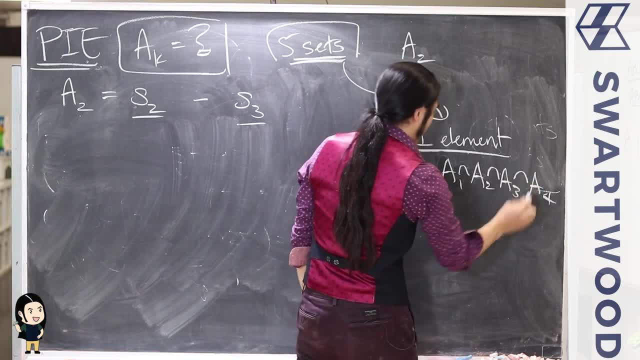 but we won't use a5.. We won't even go all the way up. Just trying to make a point. Okay, So let's say alpha is in the intersection of four of those guys. So alpha sits exactly in four of those guys. 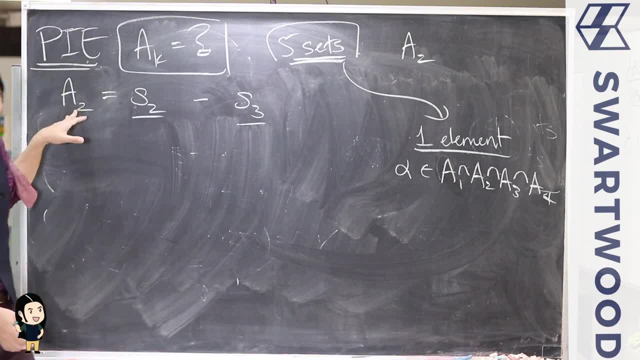 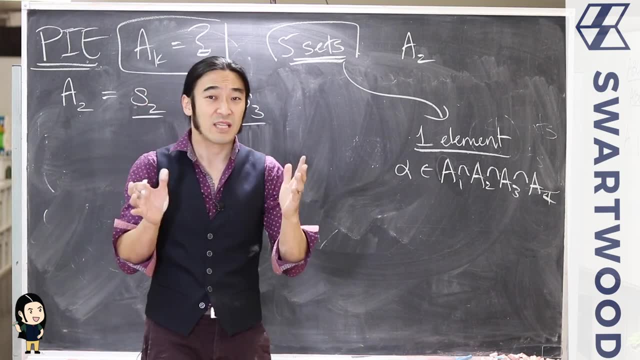 Okay. So now the first thing: if you're looking for a number of guys that are exactly in two sets, would alpha belong there? And the answer is no right. So you're looking for guys that are exactly in the intersection of two sets. 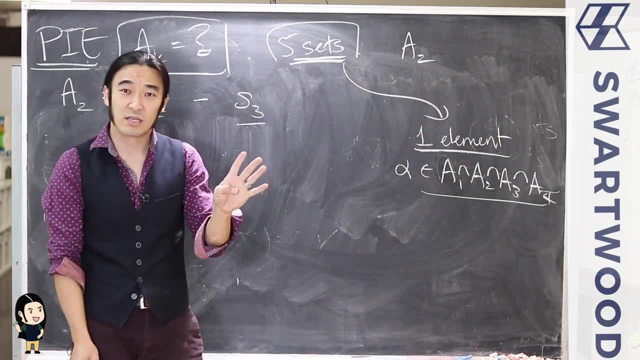 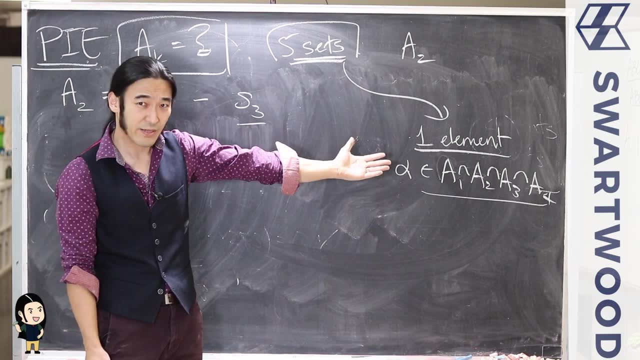 But this guy, alpha, he sits in the intersection of four guys. So if we're counting this right, alpha should not appear in this answer because he doesn't belong to just two sets, He belongs to four. Does that make sense? So guys that are legal. 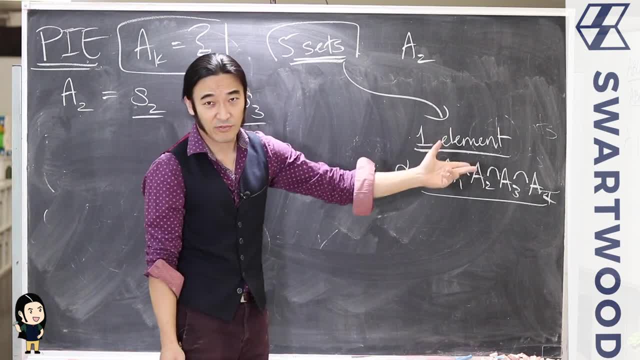 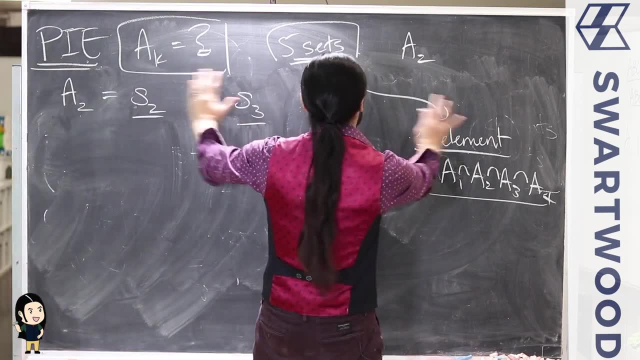 over here would be guys that are just in alpha1 and alpha2, or say alpha3 and alpha4 or alpha1, but not alpha1, 2, 3, and 4.. So what we're gonna hope to do is over here. 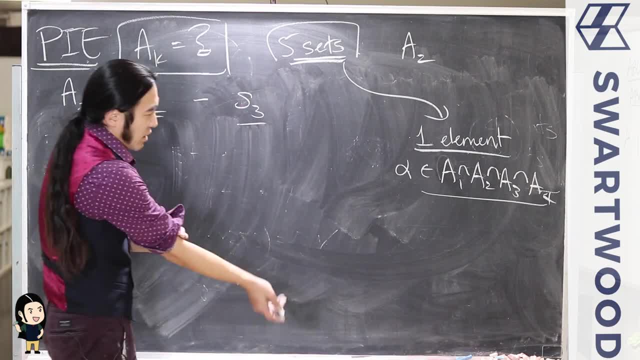 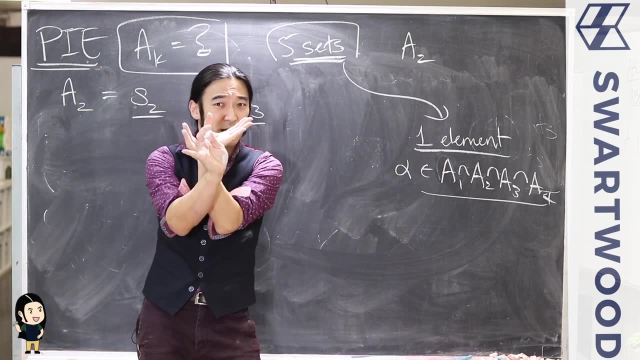 we're gonna set it up so you don't see alpha. You count them literally zero times. Okay, All right. So what's one way of doing this? We got this element alpha, and since we're always talking about intersections of two sets- 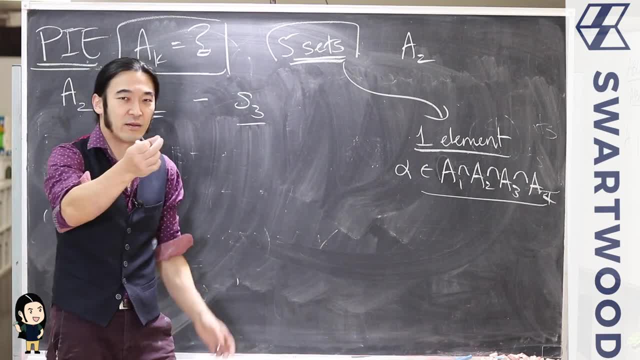 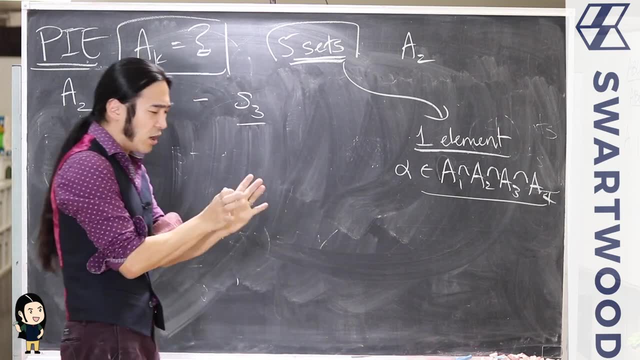 right. I think a key idea that's intuitive, at least to me, is before we look at an element and we're just looking at how many times to count it. But now let's look at an element that has two different double intersections. he can kind of sit in. 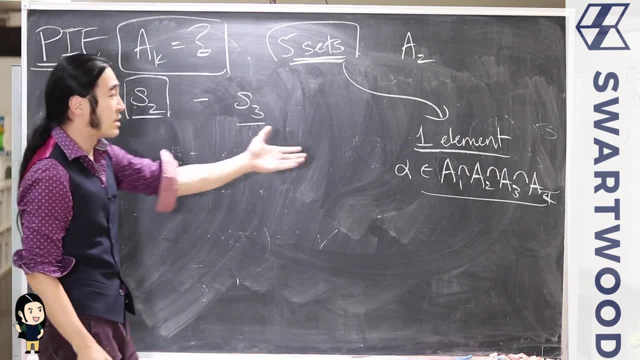 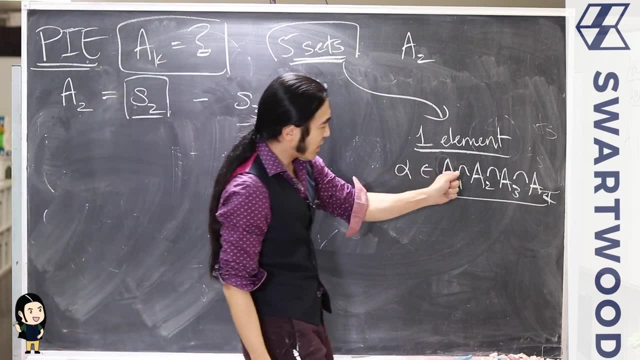 Okay, All right. Well, wherever alpha is, S2 would definitely count all the double intersections he could sit in. But now here's the thing: How many double intersections does he sit in? Well, if you have four guys, 1,. 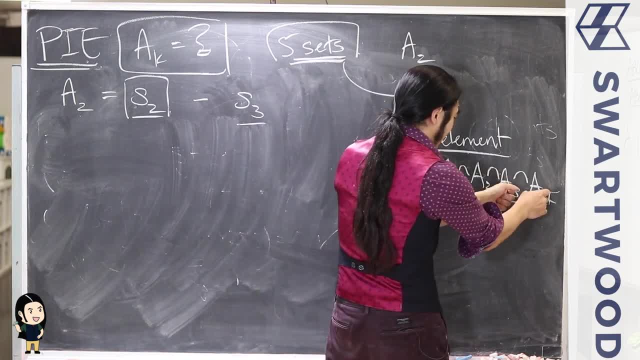 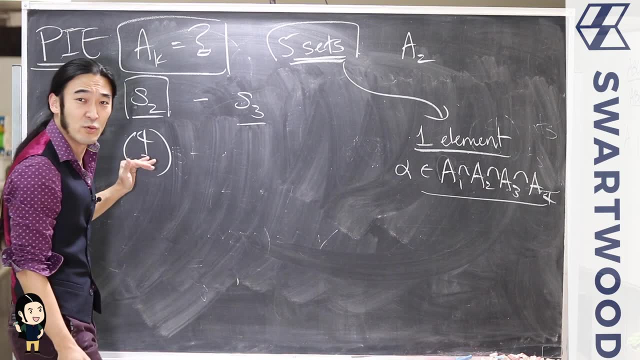 2, 3, 4, right. he sits in the intersection of a1, a2, right a3, a4, a1.. So basically any pair from here works, but you know how, if you're looking at one of these pairs, 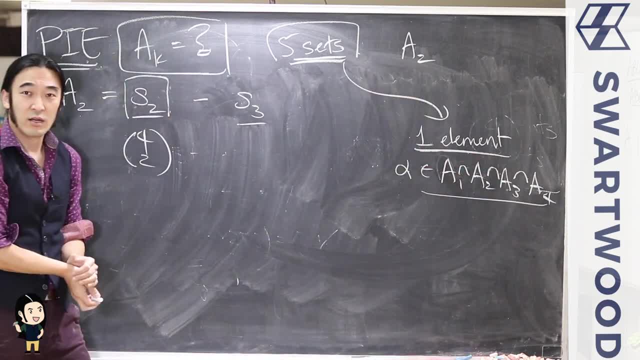 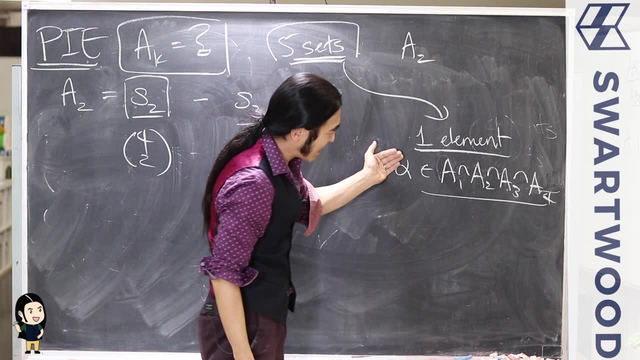 like a1,, a2, alpha definitely sits in there. It would be counted once over here. Right, Because this guy literally counts all these double intersections, everybody in there actually. But how many times is alpha counted in this guy? He's counted once. 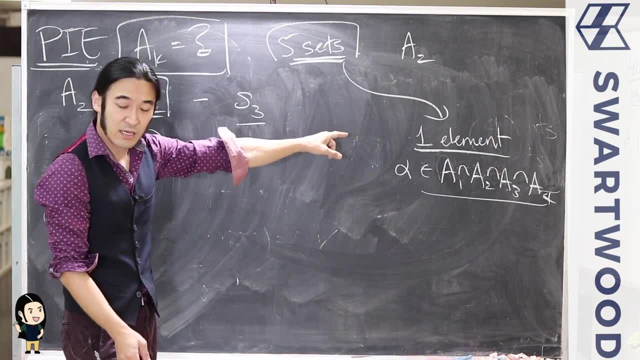 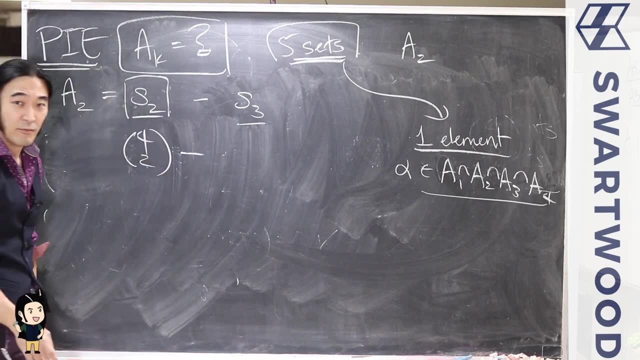 He's counted once for here, once for here, et cetera, et cetera. So it looks like you're going to have four. choose two double intersections. that alpha sits in and each time he's counted once. So this is the number. 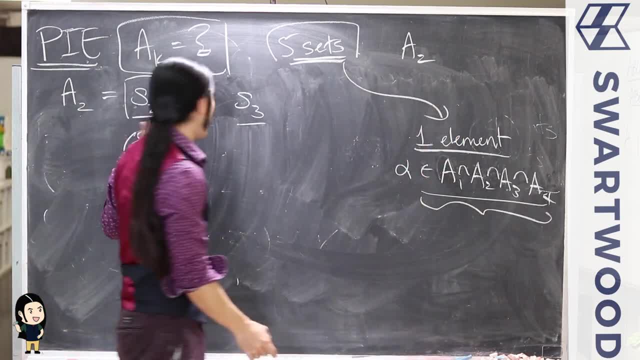 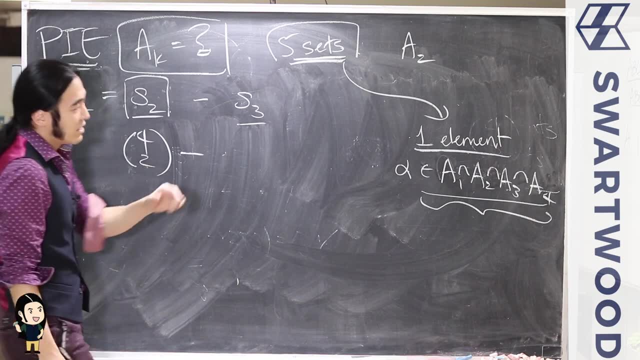 of intersections. So let's think about it this way: First, let's start off with a similar idea that I think is very natural. What we did was we saw how many double intersections alpha sat in right. Okay. Now think about this. 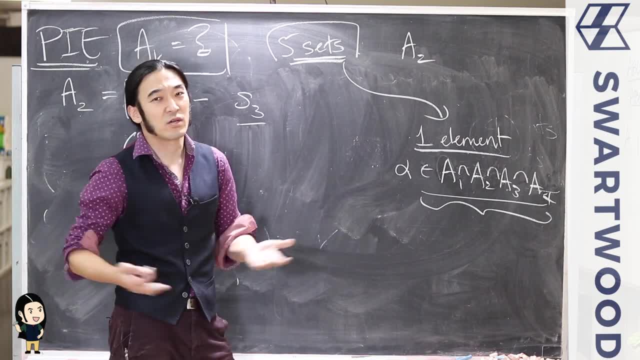 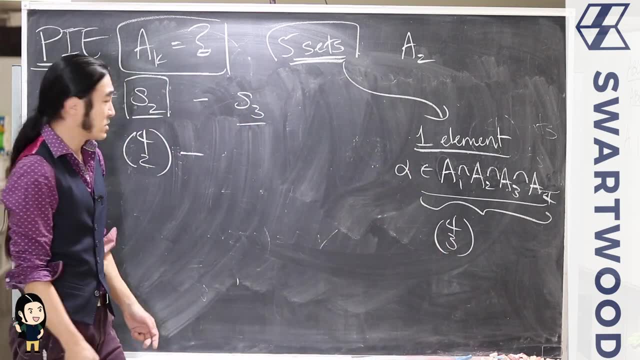 Since alpha sits in four sets right First, how many triple intersections are there period? So if you look at this, it looks like: well, I think there's four. choose three triple intersections. So I'm going to put that over here. 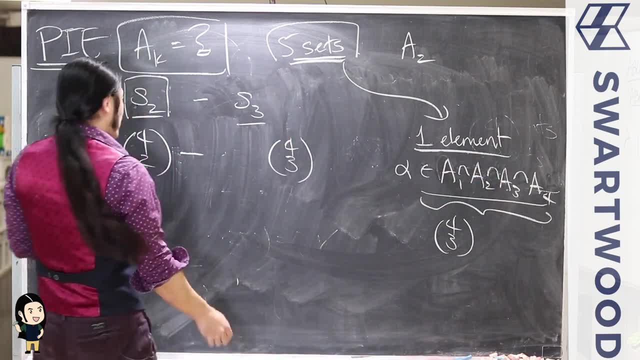 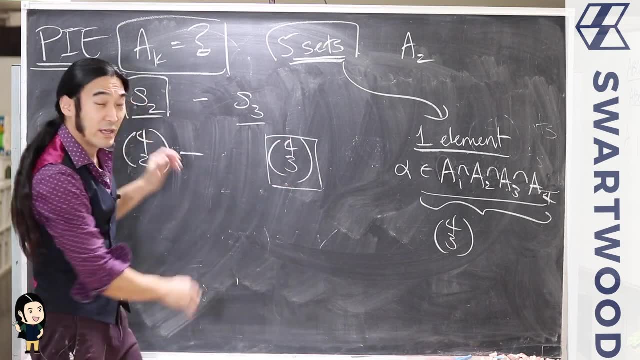 Does everybody see that There are four triple intersections? that alpha sits in, So right there. Okay, Now, I know right now it's a little deceptive. We're just going with this general theme and then we'll clean it up, Okay. 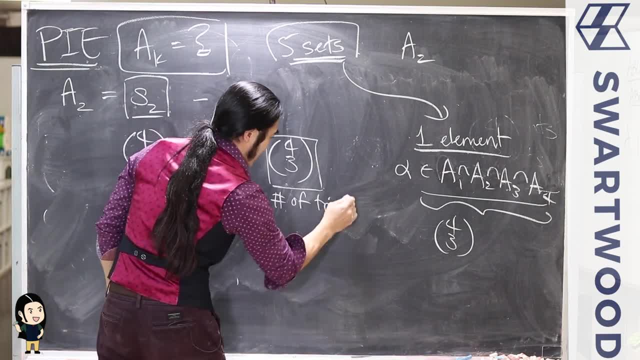 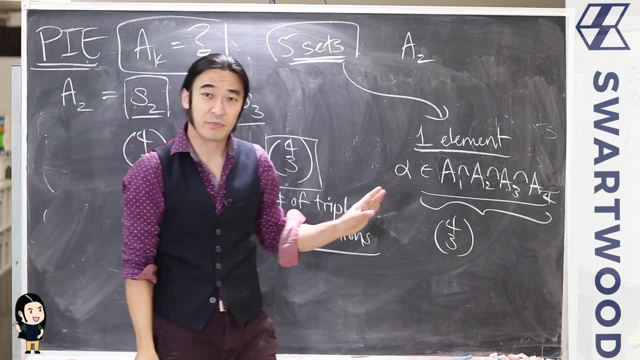 But the story's not done, because when we look in here, this is the number of triple intersections that alpha sits in, right, Okay, What we've counted here is the number of triples that alpha sits in, But that's not what I want. 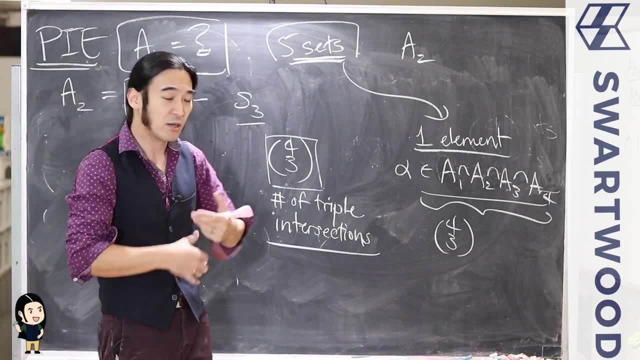 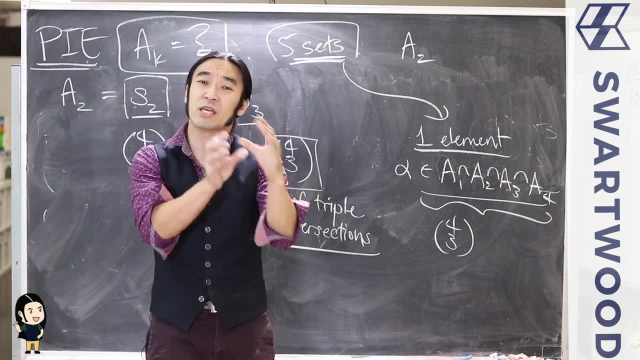 What I want to do is basically count the number of double intersections. alpha sits in: Okay, Well, there are four, choose three. There are four triple intersections, But for each triple intersection, how many pairs can you pick out? Well, in a triple intersection, 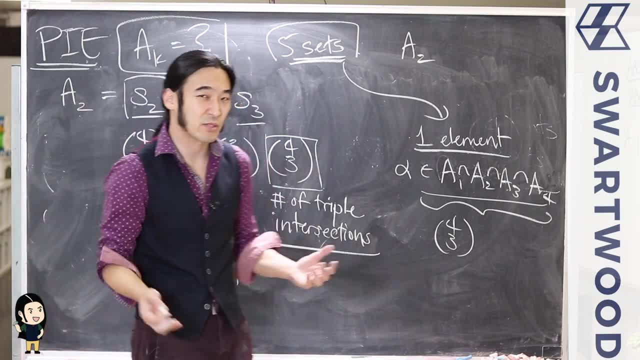 there are three guys right And you're going to pick out two. Does everybody see that? All right, So what's our game plan? So how would you come up with this crud? It's going to be like this. The idea is: 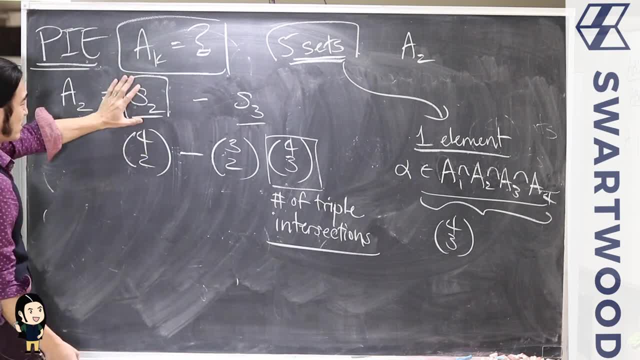 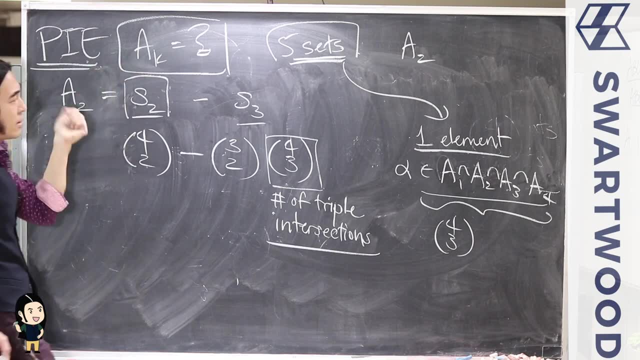 we are basically trying to count everything in terms of pairs. So intersecting pairs like this, There are only four. choose two pairs, right? That alpha sits in. So that's what we counted in here. Okay, What about in here? Well, in here. 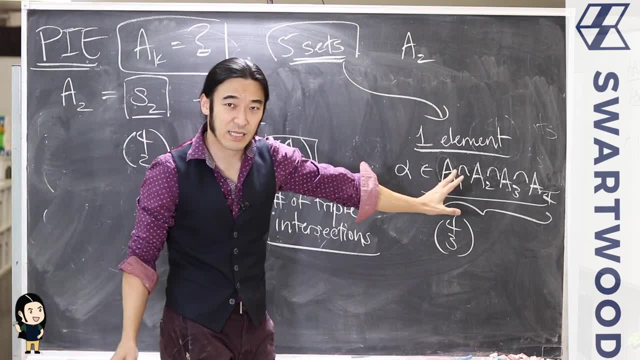 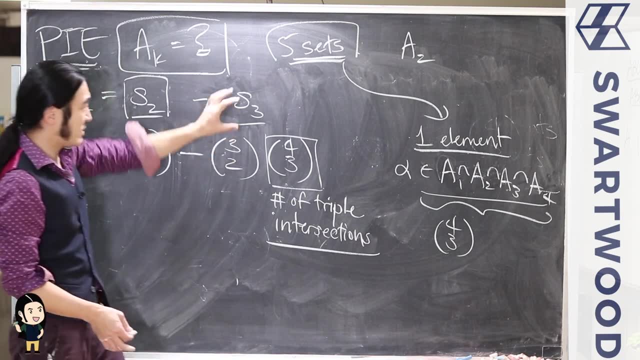 all the. this guy adds up all the triple intersections, Not just the ones containing alpha. But if we're focusing on alpha, right In this sum you will see four. choose three triple intersections that you're going to be counting here, right? 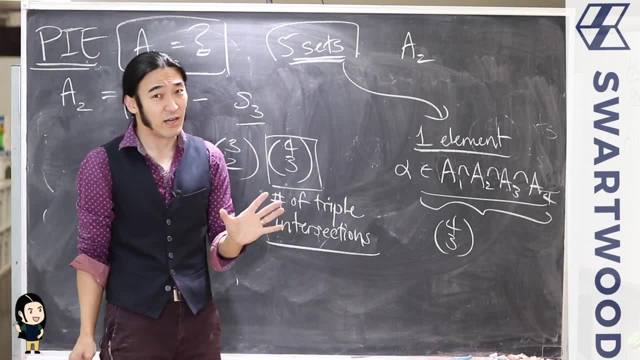 And for each triple intersection you're counting alpha once because it's sitting in that triple intersection. Okay, That's totally fine. So really, what we're doing here is we're making use of this. How alpha belongs in there, We're arguing by pairs. 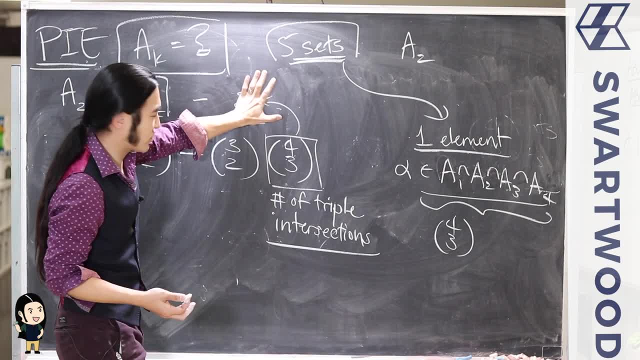 So really, what I want to do is I want to say, okay, there are this many triple intersections that are counted for here, But what I really want to do is count the number of pairs. So for every triple intersection you have three. choose two pairs. 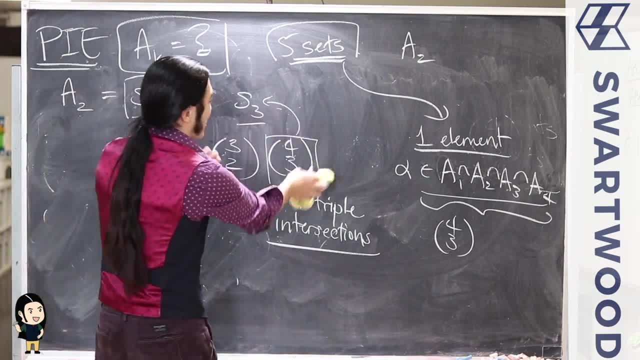 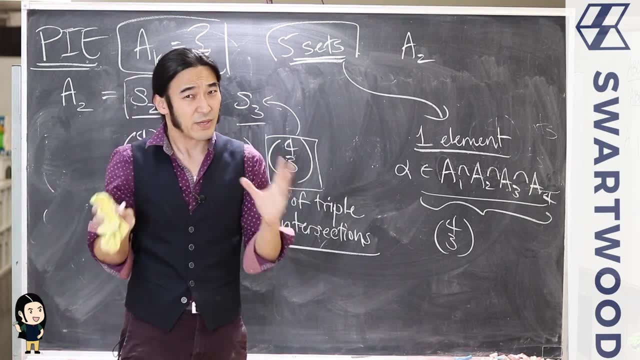 Does that make sense? Okay, Then we're basically recounting all the pairs again, But we're doing it from the point of view of triple intersections. So you take a triple intersection and count all the pairs from there. Okay, Does everybody see the big idea? 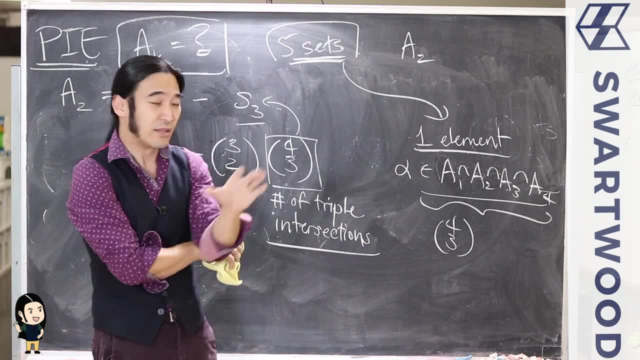 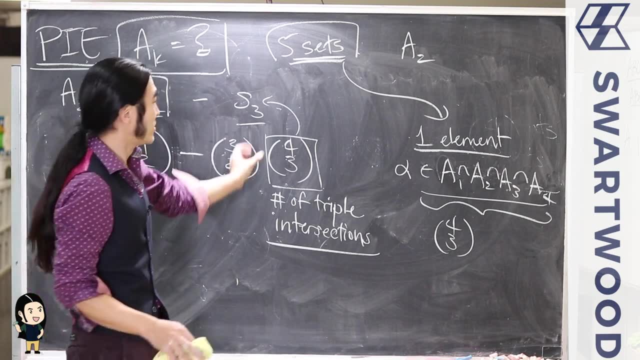 Sorry, I don't want to beat this to death, But I'm really saying it because I think once you have that big idea, then the rest of it is very mechanical. So you're counting out pairs period. Here you're counting out pairs, but in a different way. 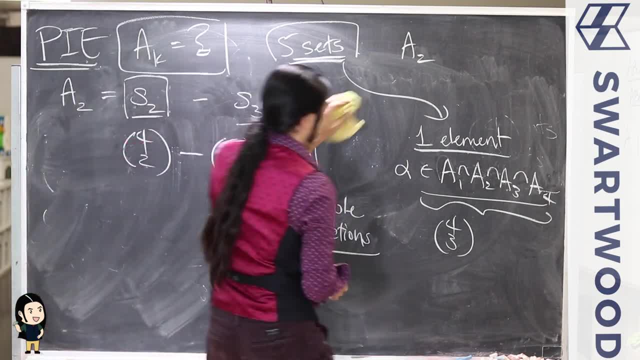 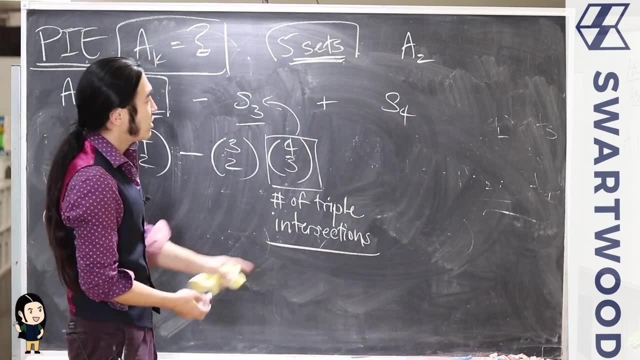 First you look at the number of triples and then the pairs that belong to those triples. Then you know, over here we're going to run it all the way Because you know in general inclusion exclusion We might be over counting Right. So now we're going to look. 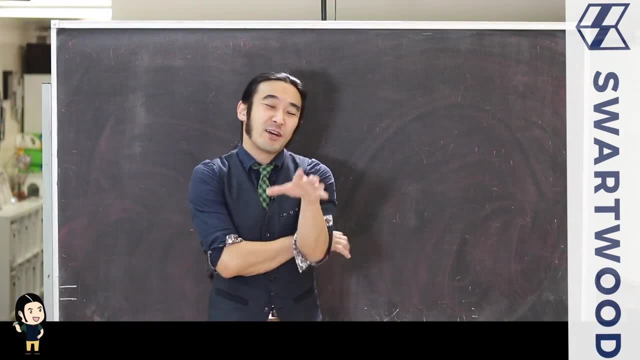 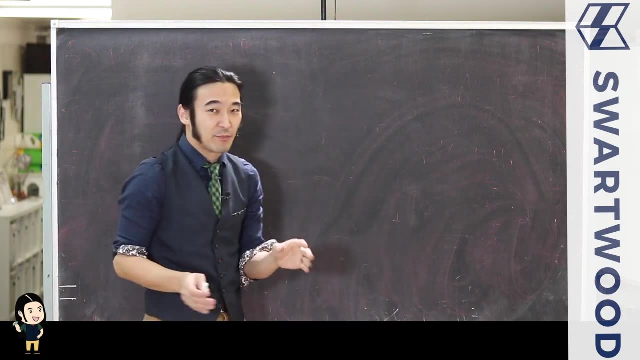 at all the quadruple intersections. Hi guys, You might be wondering about the costume change. Sorry, but the camera actually ran out, So it ran out of charge last time. This time we're a little bit better prepared, so I'm going to go ahead. 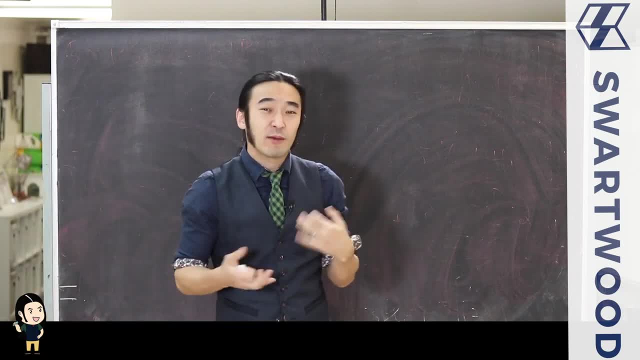 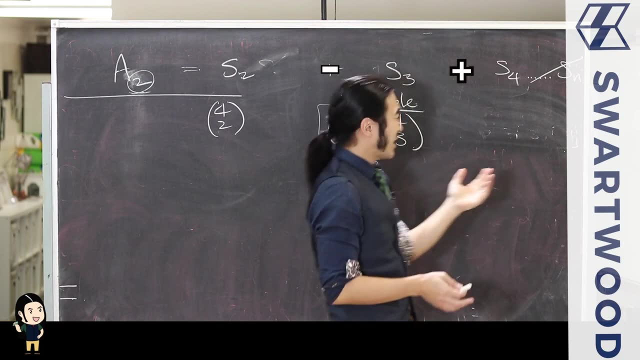 and finish. Okay, So let's think about what's the inspiration. How would you come up with this? Okay, So our idea was this: It isn't just that you're looking at double intersections and triple and quadruple. Then it'd be like where? 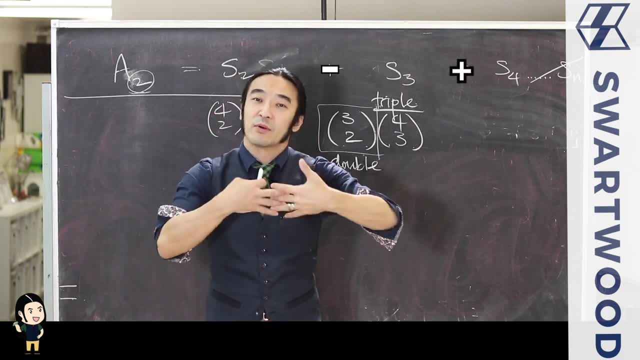 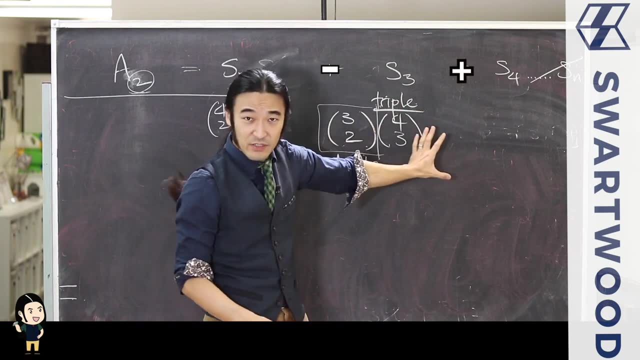 did these coefficients come from? It's? you want to visualize it like you're actually counting all the double intersections Just different ways? Here, just straight up, It's going to be the right number, Right. Then here do it in terms of triples and the doubles. 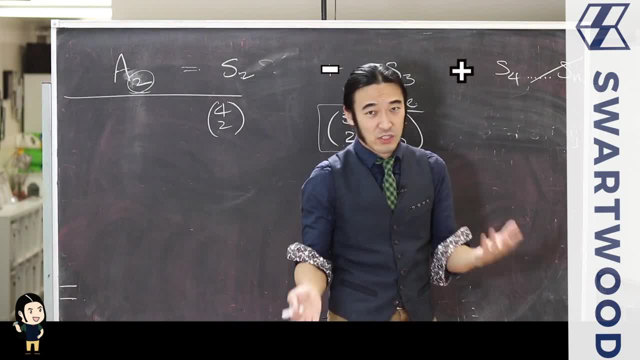 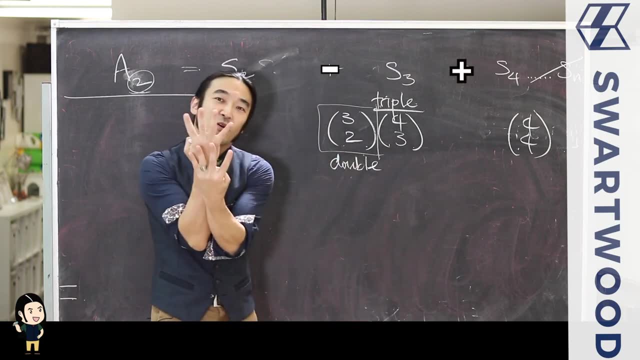 you get from the triples and that will be over counting. Okay, And we're going to make an adjustment or we're going to check that when we do all this, it's going to be: how many quadruple intersections are you sitting in? Just one. 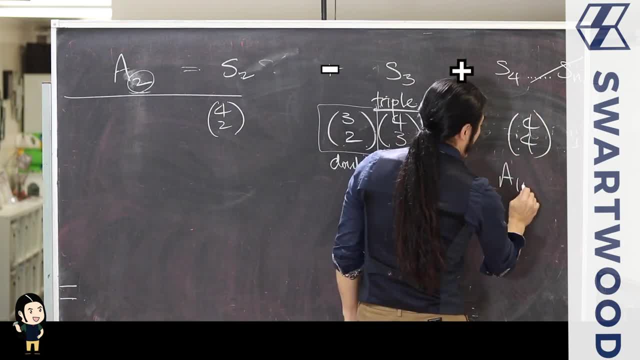 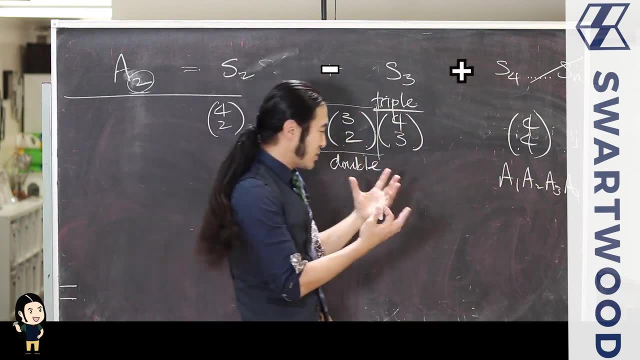 Because you have to choose all four of those sets, Right? So it's going to be four. choose four, one because, remember, these are literally all the sets that alpha sits in. But then for every quadruple intersection, again the same procedure. How many double? 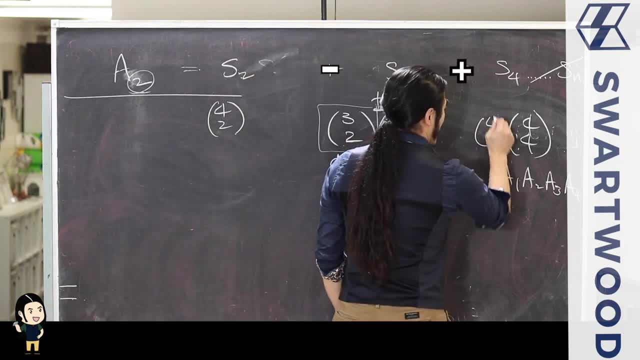 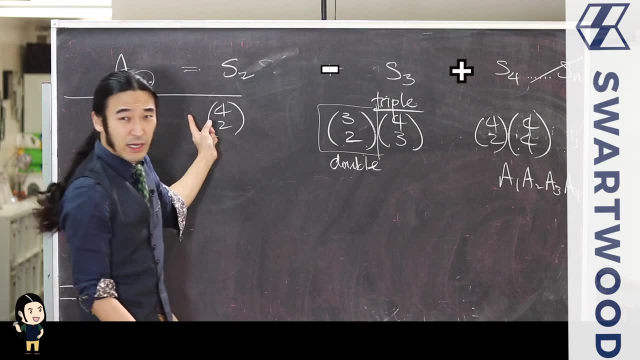 intersections. is alpha going to sit in? Well, that's going to be four, choose two. Now you might be like: well, this is kind of lame, because here you counted it right, Here you over counted, and here you kind of counted it right, because you end up getting the 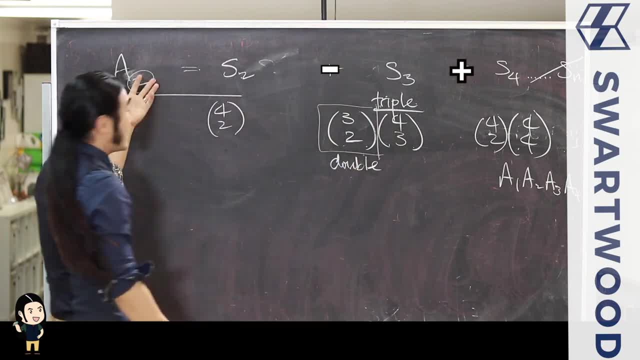 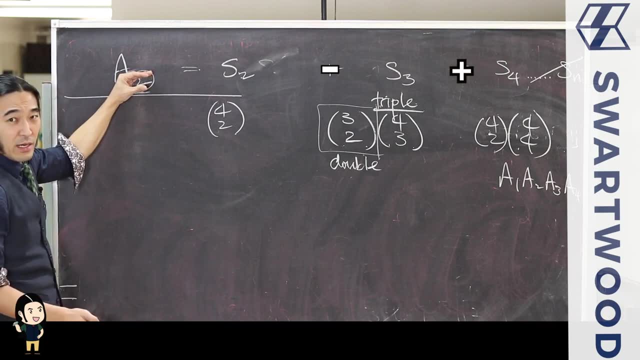 same number, Right. So the procedure remains the same. Right now it's double intersections, but it could have been triple, quadruple, quintuple, whatever, Okay. But the idea is, whatever your target number is right, we're going to count those sorts of intersections. 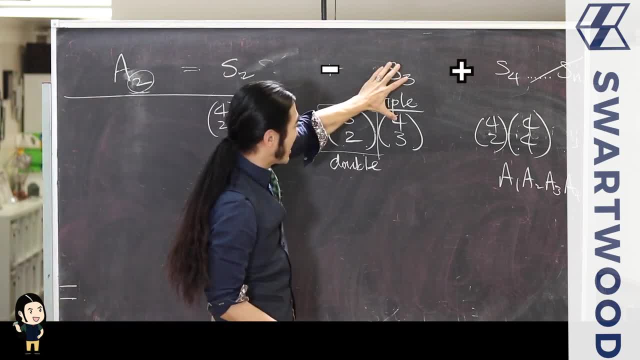 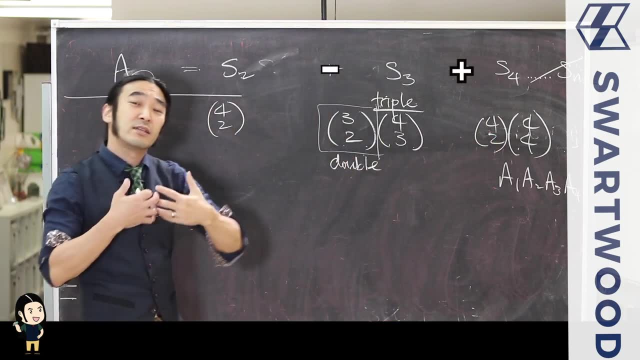 And we're going to do it just first, straight up. We're going to take bigger collections and then generate from them, and then bigger groups over here and generate from that. Okay, So it's just in this case, to be concrete, we're counting the number of. 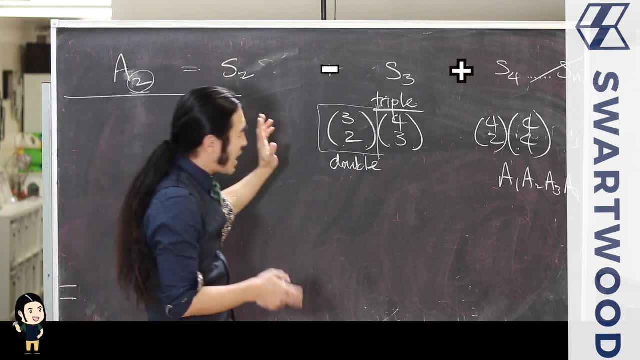 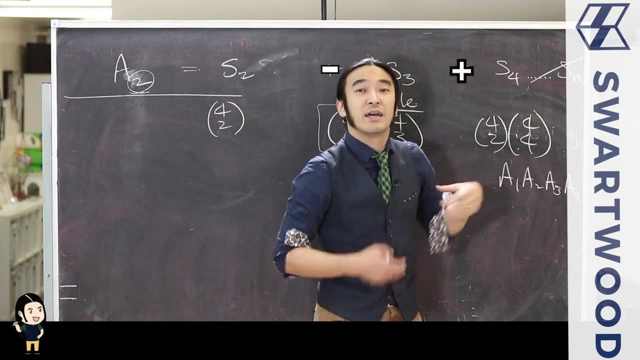 double intersections. that alpha sits in. We're doing it straight up. then we're kind of doing a sloppy. we're doing first two triples you can get from the possible guys and the doubles generated from them, and then the quadruples and the doubles generated from them, et cetera. 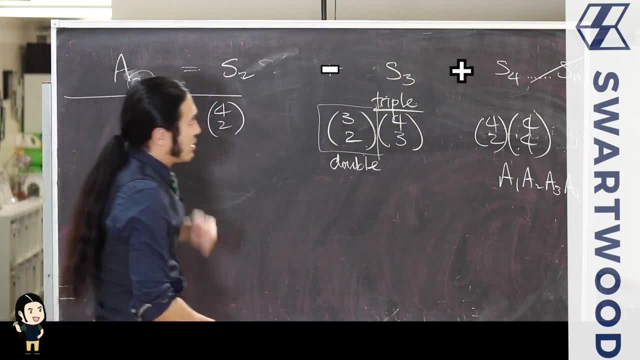 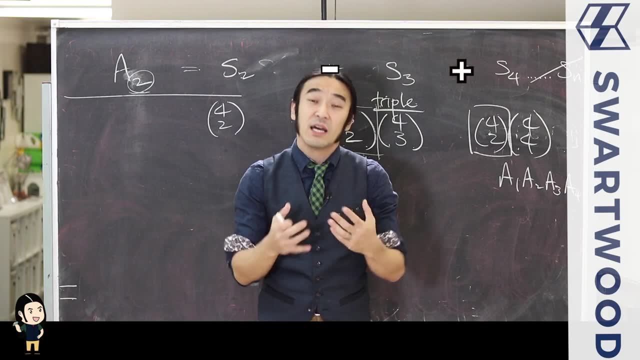 et cetera. Okay, That's the idea, All right. So now. and, by the way, these are actually the coefficients. so that's the inspiration. So the way you should view it is, those coefficients come from this idea of let's count all the double. 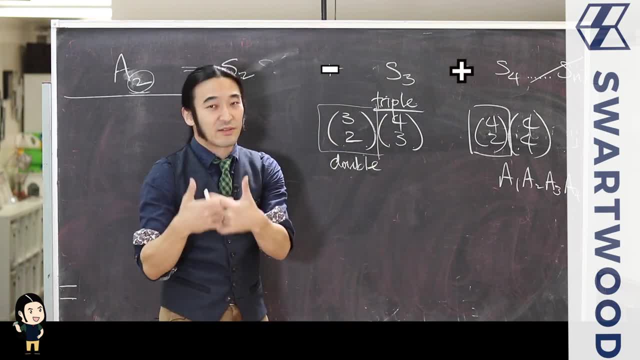 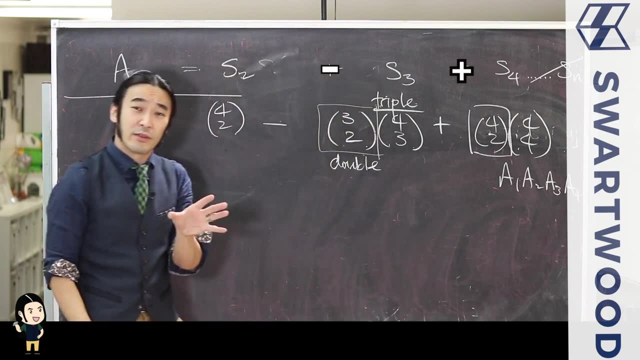 intersections, that alpha sits in, because that's what we care about. We're just going to do it different ways, Okay. But then you're thinking it might be okay. well, you know, we do the whole thing: subtract and add and so on, right, How do we know then that? 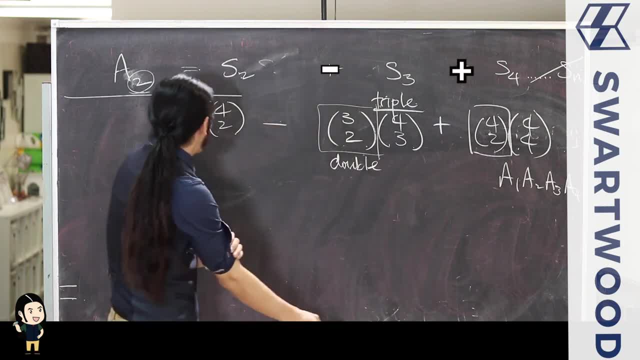 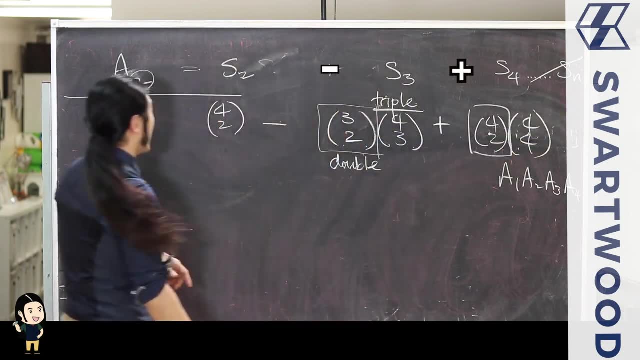 this is going to count it right, because my claim is it All right? Well, let's say this: If alpha only sits in a double intersection, then it wouldn't be in a triple quadruple. so all of these would be gone, right, It would be in one double. 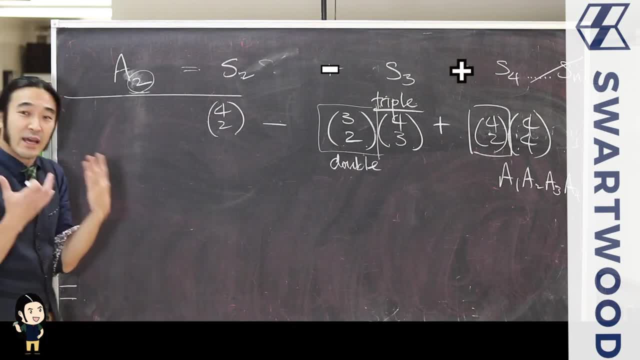 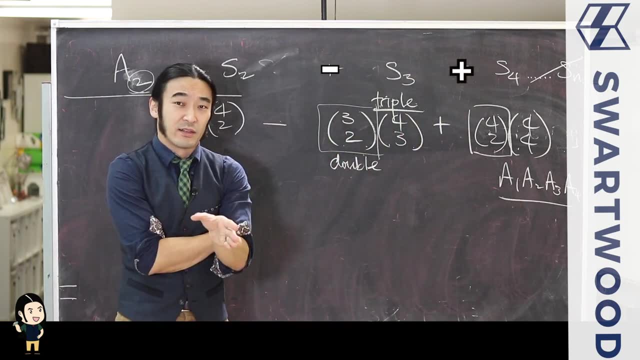 intersection. so you count it one time, and of course it would be counted once here, because it would be an element that only belongs to two sets. Okay, All right, But now, like in this hypothetical case, alpha belongs to four, So should that count on the? 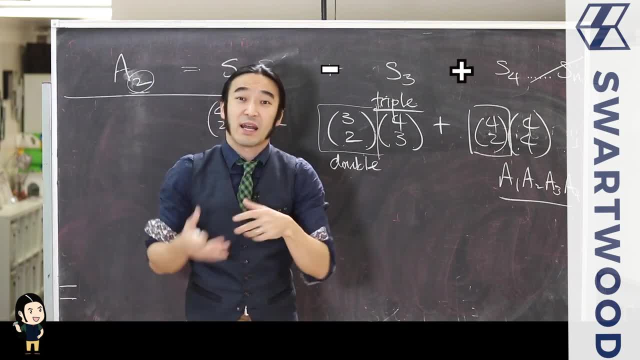 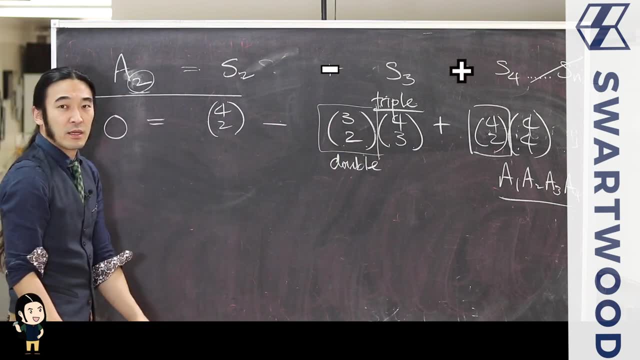 left. No, because the left counts only the guys that sit in double intersections. But alpha actually sits in a quadruple intersection Right. So on the left alpha should be in a quadruple intersection. It should be counted zero times, But of course if you sit in 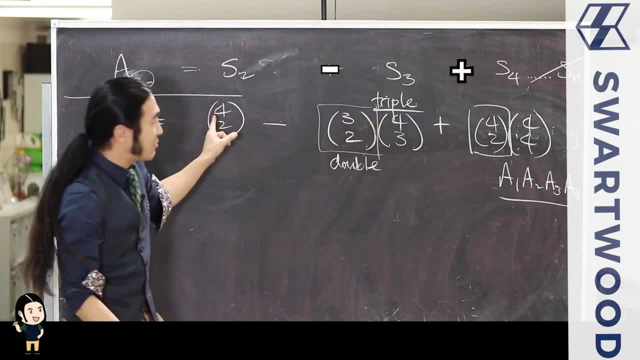 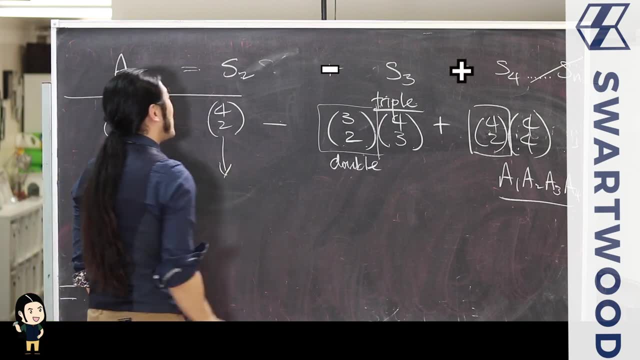 a quadruple intersection. you also sit in double intersections, So what we're doing is we're counting those guys up and we're hoping that when we count it, everything will go to zero. Okay, So let's see that First. this is actually the 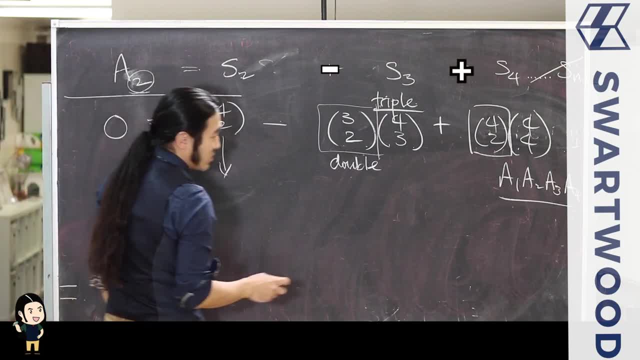 number of double intersections that alpha sits in. That is actually the correct number And if you imagine these guys like, let's do that, A1, A2, A1, A3, A1, A4, A2, A3, A2, A3, A4, A5, A6, A7,. A8,, A9,, A10,, A11, A11,, A12,, A13,, A14,, A15,, A16,, A17,, A18,, A19,, A20,, A21,, A22,, A23, A24,. A23,, A24, A24,, A23,, A24,, A24,, A23,, A24,, A24,, A24,, A23,, A24,, A23,, A24,, A24,, A24,, A24,, A24,. 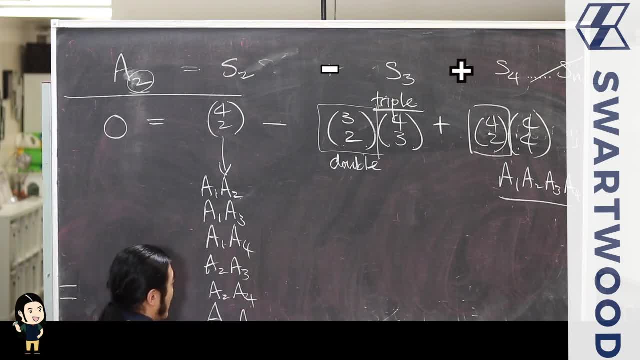 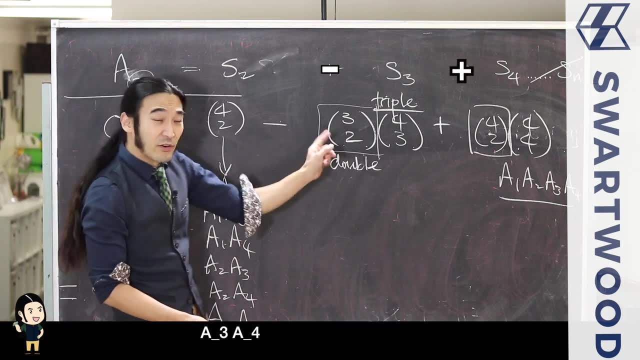 A23, A4.. If we did it right, there should be six of them. Yeah, These are all the double intersections. that alpha sits in And that's the correct number. Okay, But now over here. Over here, we looked at the. 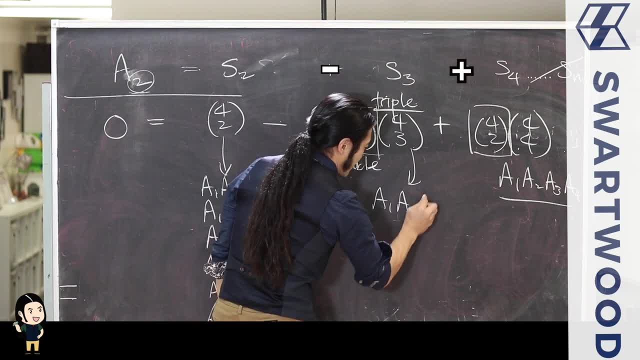 triple intersection, So that could be A1, A2, A3.. It could be A1, A3, A4.. It could be A2.. Oh Shoot, My bad, I forgot the video is truncated here, So I'm going to go ahead and do. 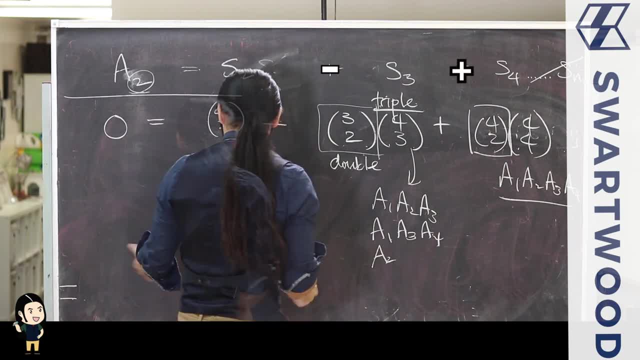 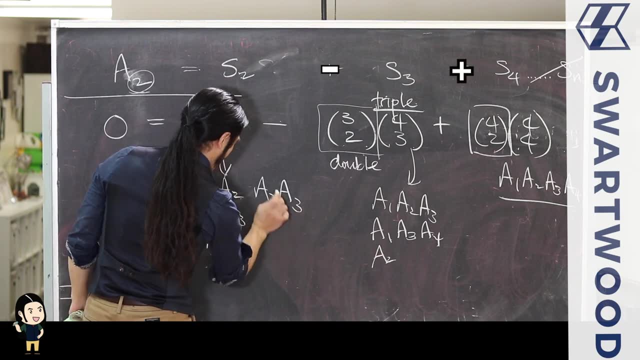 it like this, so you can see everything. Okay, Anyway, hopefully that's the same. I said it correctly. It's just you probably couldn't see it on the screen. So there you go. All right, So let's go for this. A1, A2,, A13,, A14,, A15,, A16,, A17,, A18,, A19,, A20,, A21,, A22,, A23,, A23,, A24,, A25,, A26,, A27, A28,. A29, A29, A30,, A31,, A32,, A33,, A33, A33,, A34,, A34,, A35,, A36, A35, A36, A47,, A38,, A39,, A40,, A41,, A42,, A43,, A43,, A44,, A45,, A45, A41, A43,. A45, A46, A46,, A48,, A47, A47,, A42,, A43,, A14,, A47,, A48,, A48,, A14, A45, A14,, A43,, A43,, A14, A43,. 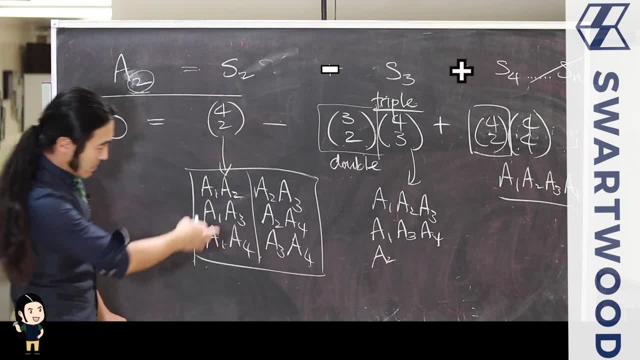 A14, A48, A14, A43, A41, A43.. So let's go for this: A1, A2, A4.. So my apologies if I miscounted, but I think these should be all the triple. 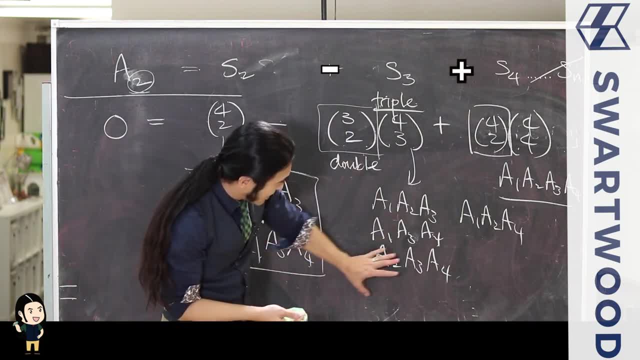 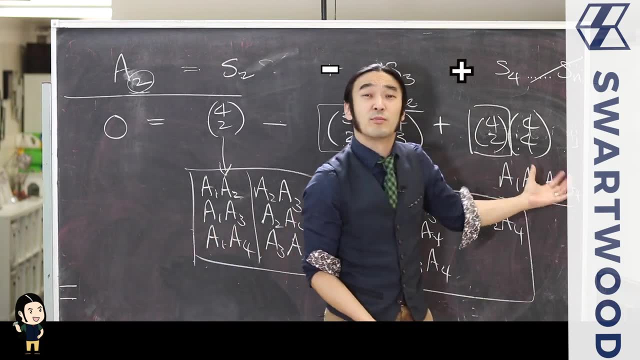 intersections we can pull out. Okay, All right. Now it stands to reason that if you take all four and you pull all the doubles from All right Now it stands to reason that if you take all four and you pull all the doubles from them, 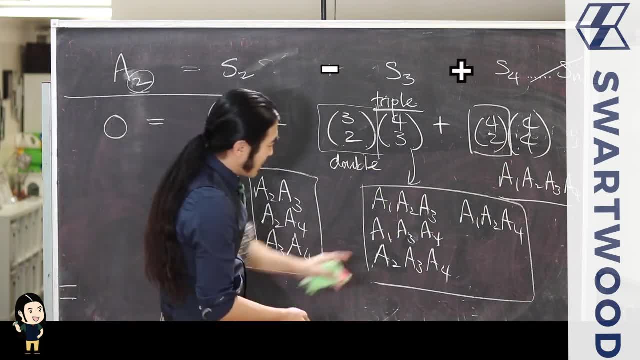 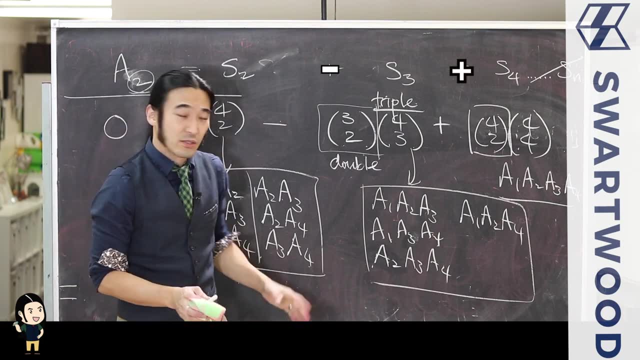 we're going to get exactly the same guys over here, But anyway, the main argument's going to be from this. So how's this going to work? These are the number of double intersections. alpha sits in, So this is the right number. 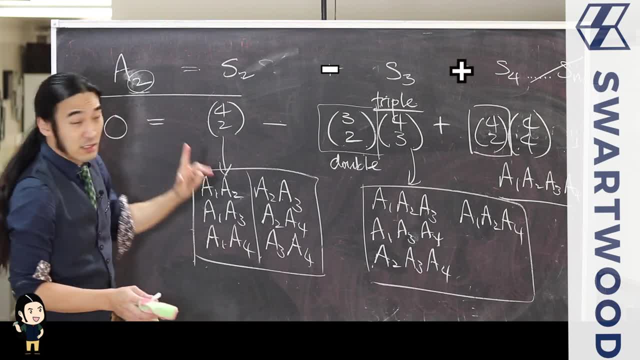 So if we count this up and we subtract it out, then we should get 0, and that's what we want, Obviously, when we're counting here, we're going to see in a second we can overcount. Now we could write all this crud out, but that's a pain. 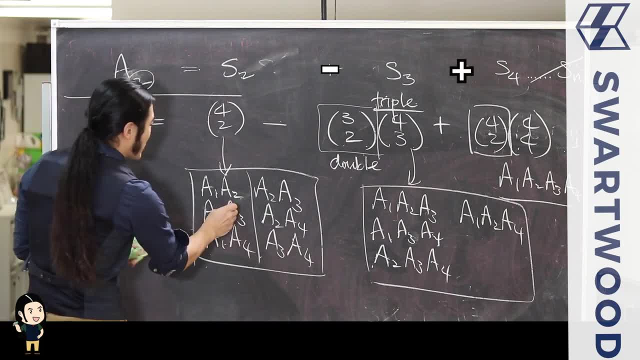 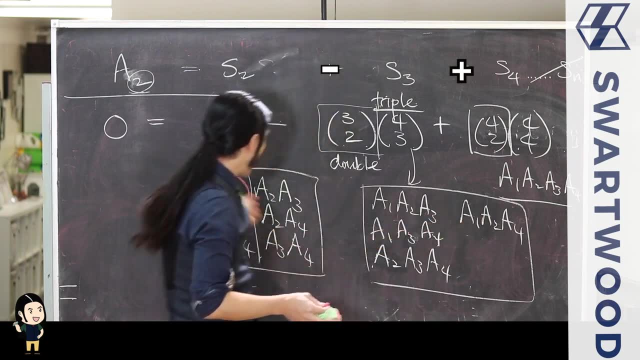 So what I want to do is I want to focus on what happens with each individual guy. Let's focus on this guy. Well, first, do you guys agree From these triples? when you pull doubles from them, you're going to get every single one of these. 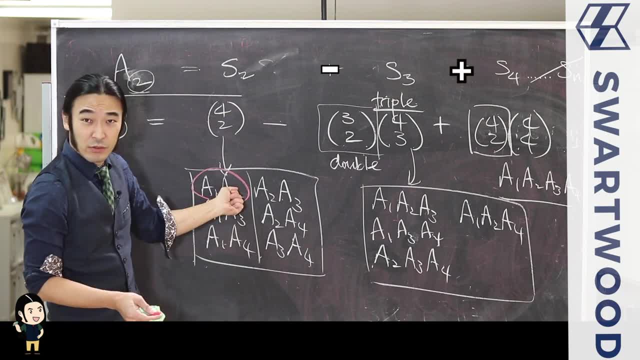 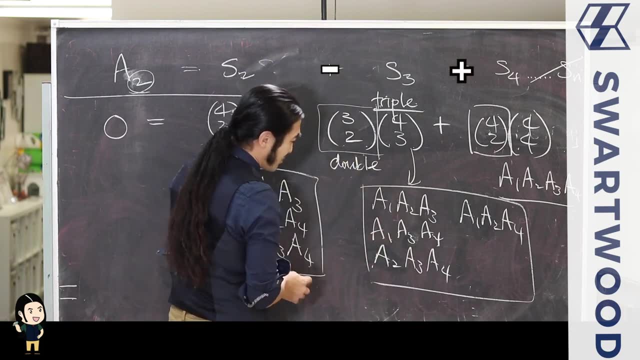 That's not the problem. We've overcounted because sometimes guys over here- like A1, A2, will count multiple times on the right. So how can this happen? How many ways are we going to overcount? For example, if we look at this guy, A1, A2.. 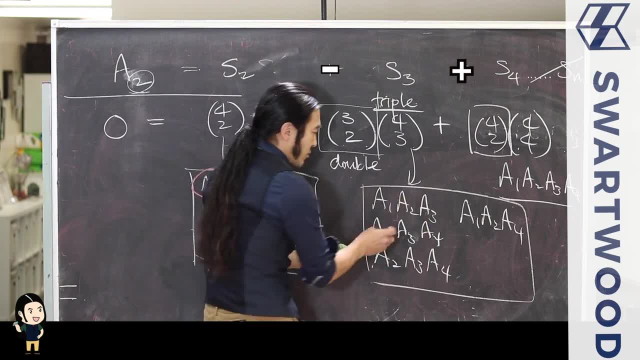 Well, if you're pulling doubles from these guys in order to get A1, A2, you have to contain A1, A2. So that one works. This one does not, Because you can't get A2 anywhere from this. 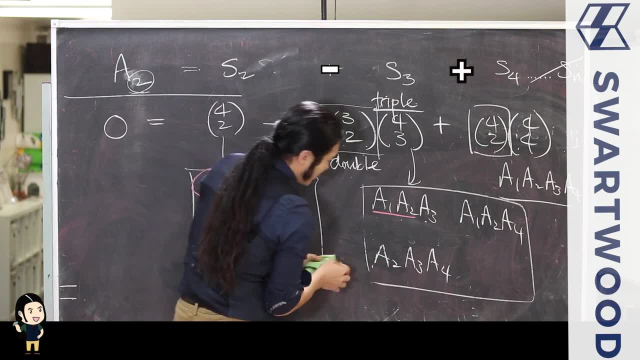 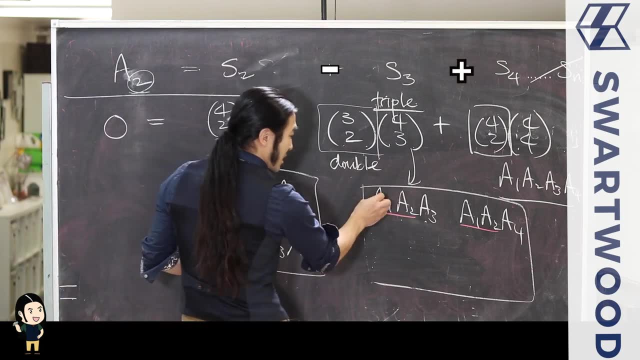 So we're going to ignore him for the moment. Let's see: Over here nope, Over here yes, And then when we compute the doubles we can pull from this we're going to end up getting. So from this, we can definitely get A1, A2.. 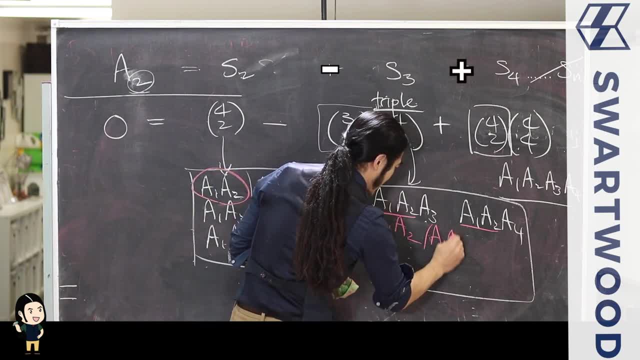 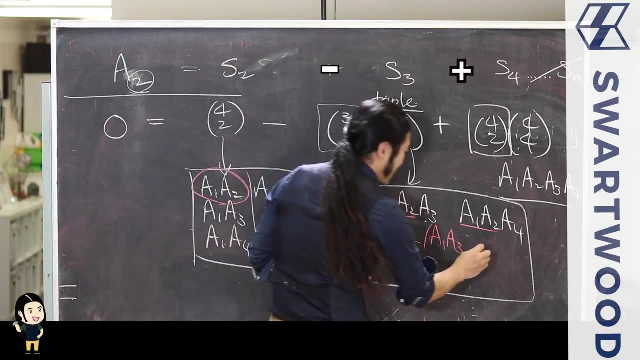 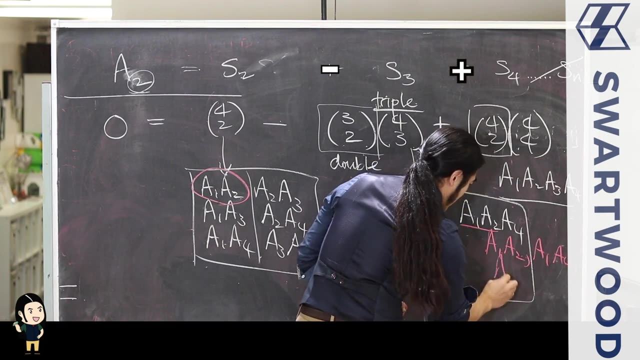 We can also get- let's see A1, A3, and A2, A3.. All right, Over here, what can we get? We can end up getting A1, A2.. A1, A4.. And A2, A4.. 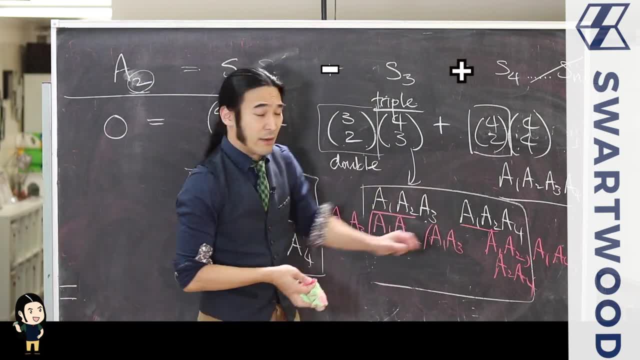 OK, All right, Does everybody agree? these are the guys that we can pull? OK, But my argument is going to be: and so clearly, we're going to get everybody but we're going to overcount. I want to focus on this guy, how we're overcounting this guy. 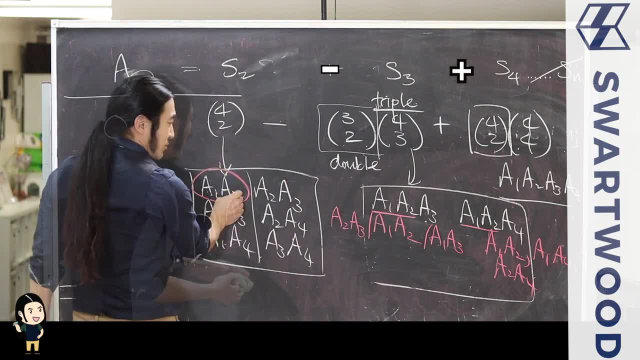 Because this argument will hold up for any of these double intersections. OK, Let's look at A1, A2.. We see it here and here, So we're going to overcount twice. We're looking for a general pattern, so let's actually count. 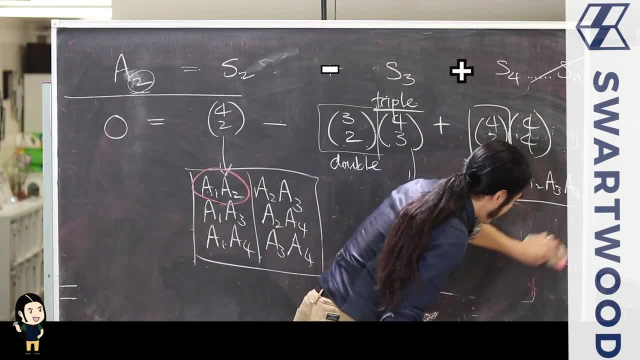 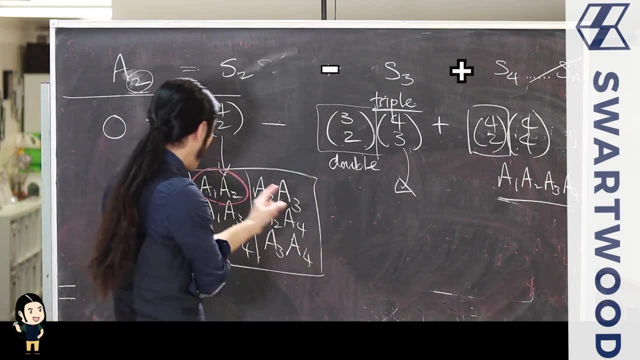 Let's count this out. So the thing is is that Over when we look at the triples, it could be the case that different triples will generate A1, A2.. From a given triple, we're not going to generate A1, A2. 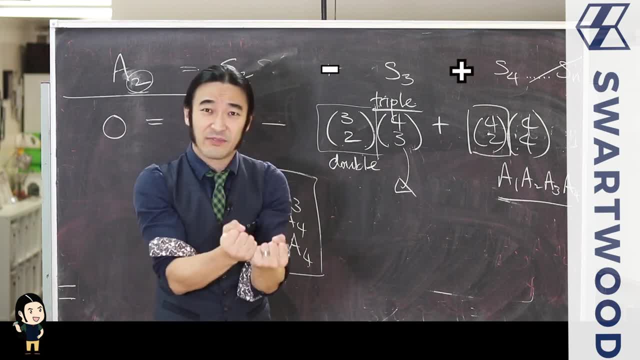 more than once. right, If you have three guys and you're pulling two like A1, A2 specifically, there's only one way to do that, But you may have different triples- that when we pull pairs from them, we're going to end up with the same guy. 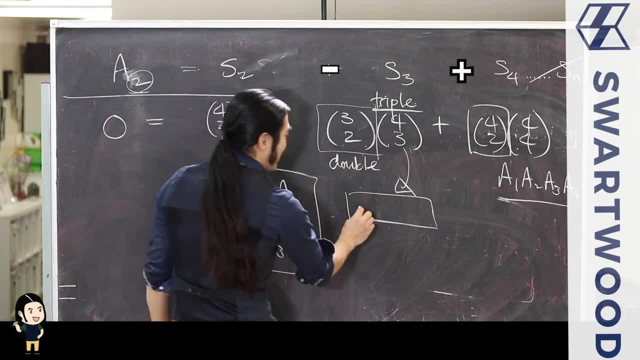 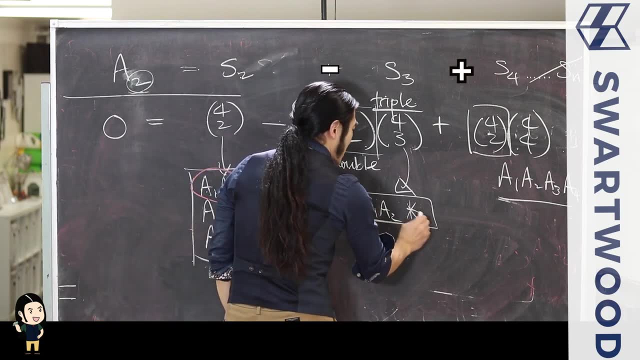 And that's overcounting. But in order in general to have a triple that's going to end up giving us this pair A1, A2, you have to have A1, A2 in that triple right. But that means that the thing in the third position 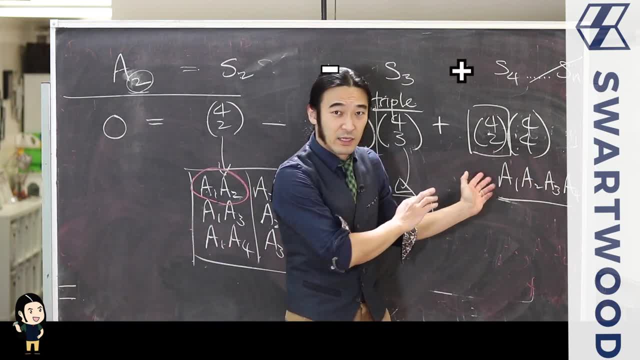 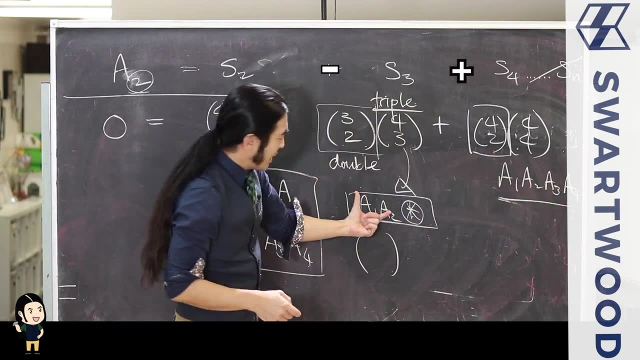 could be anything right, Anything that's legal, any of these sets that contains alpha. So how many ways are there of doing this? Well, let's see. All right, We have four guys out there that contain alpha. A1, A2 are fixed. 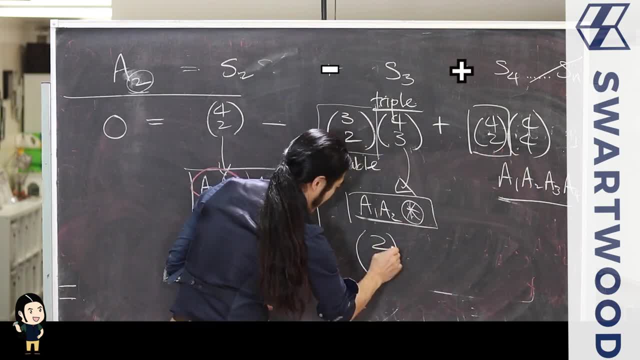 We don't have a choice about that. So if you pull out A1, A2, there are two guys left. OK, Of those two guys you can pull one or put one in that position. So it's two, choose one, OK. 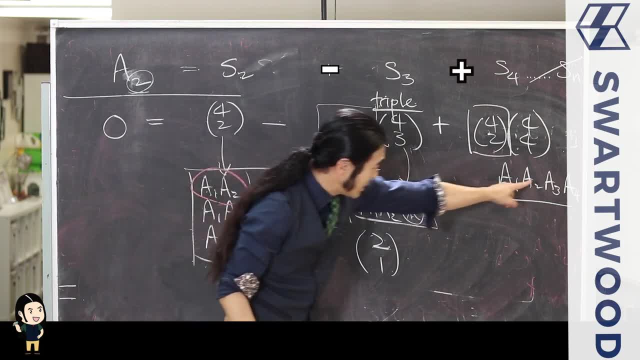 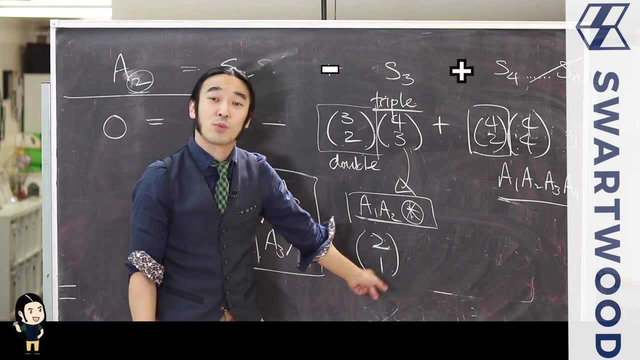 And it's clear, if you just count this out, This is A1, A2, and A3, or A1, A2, and A4.. OK, So that's it. So it looks like for A1, A2, we've overcounted two. choose one. 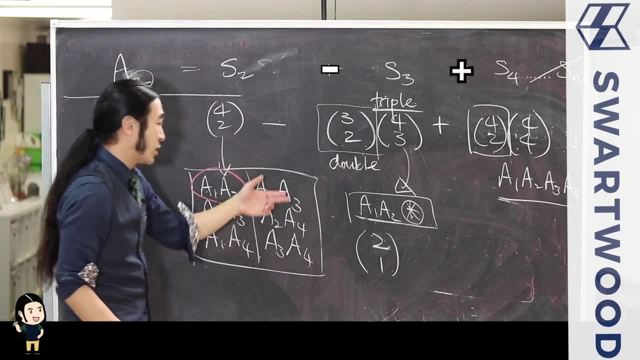 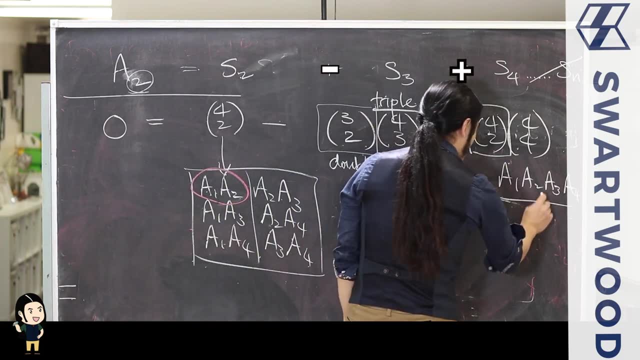 times, But that holds up, if you think about it for a sec. for every one of these, OK. So this guy is overcounted. two choose one times, OK, All right. but now what about over here? Let's try to do the same thing. 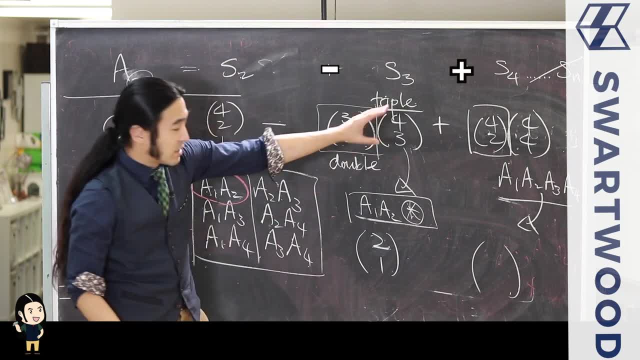 Well, this one's going to be pretty mellow. What ends up happening is we take a quadruple guy there, right, And we want to know. well, in this case it doesn't really matter, because it's only one quadruple thing. 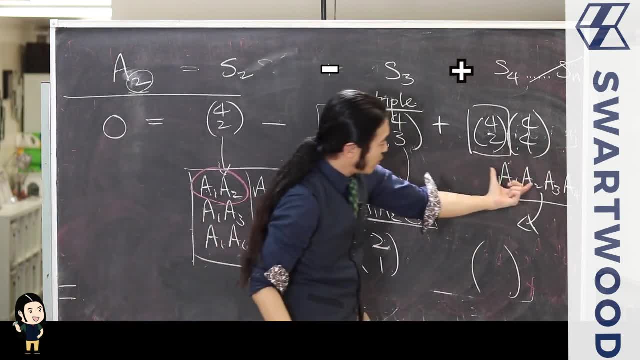 But let's just think it out In case. if you had a quadruple guy and you want to pull two of them, right, What is the requirement? Well, in order to contain- let's do the same- argument A1 and A2.. 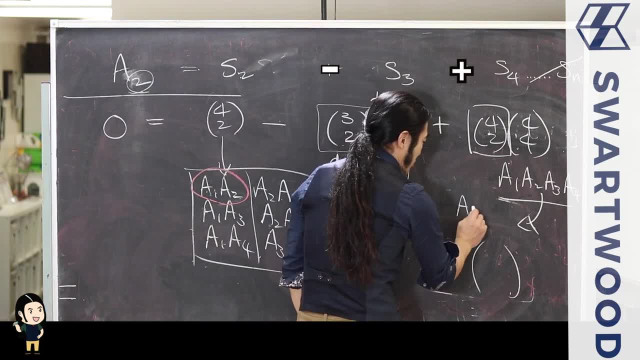 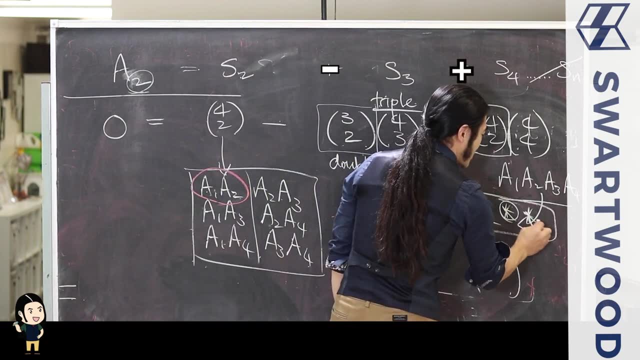 We're going to focus on that, Then that means we have to include in our quadruple A1 and A2, OK, So those guys remain fixed And now we need to fill in two slots. OK, so if you pick A1 and A2, that only leaves A3 and A4. 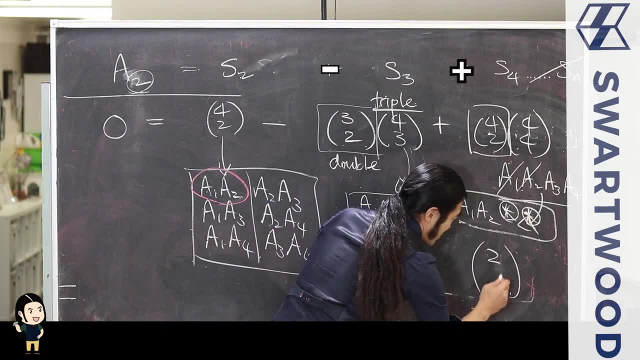 in the running, But you need to choose two guys to put in there. So out of the two options, you've got to choose two, And that, of course, is going to leave you to one, but you know that because there's only one. 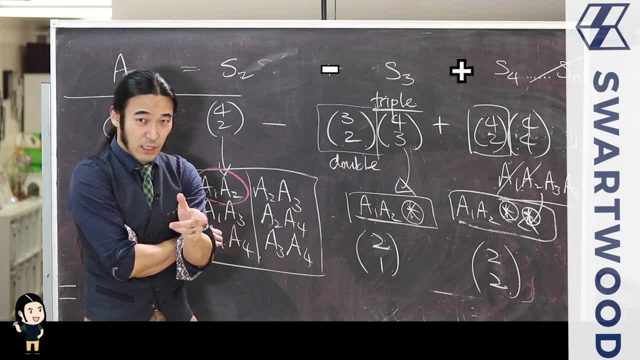 quadruple out there in this case, But you see how the pattern will hold up in general. OK, so let me get this straight. Oh, and how about over here? Well, over here, we know we're going to count it correctly one time. 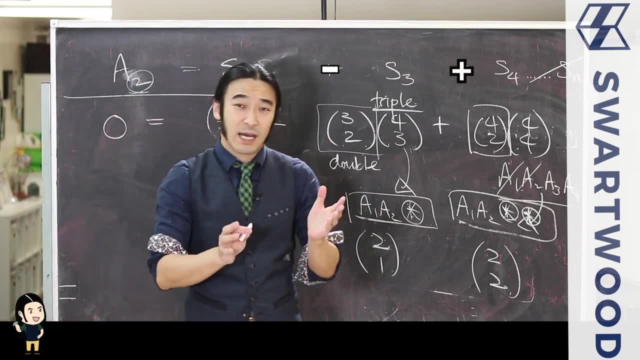 So you can think of it like this: Here it's definitely going to be one time. You count that double one time, correctly. But to keep the pattern up, you can think of it like this: You pull that double A1, A2.. 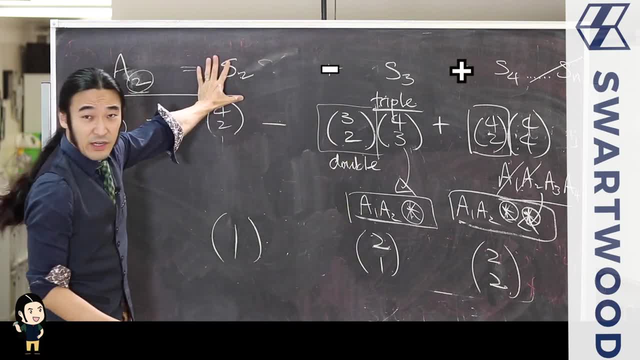 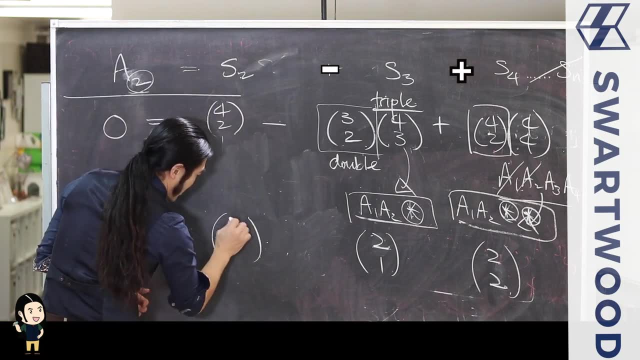 OK, how many more do you need to fill in? Well, you're only looking at doubles over here, So you're done. So if you pull out A1 and A2 to be in your double, how many guys are left? There's still two guys: A3, A4. 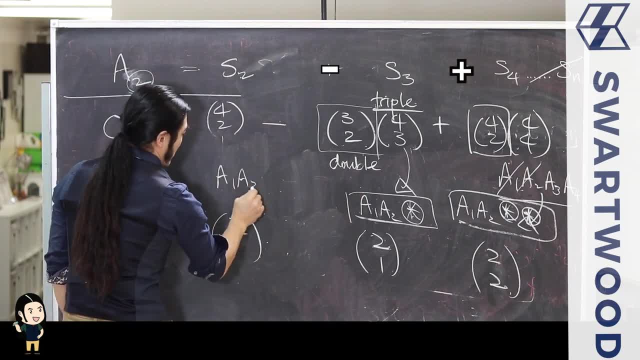 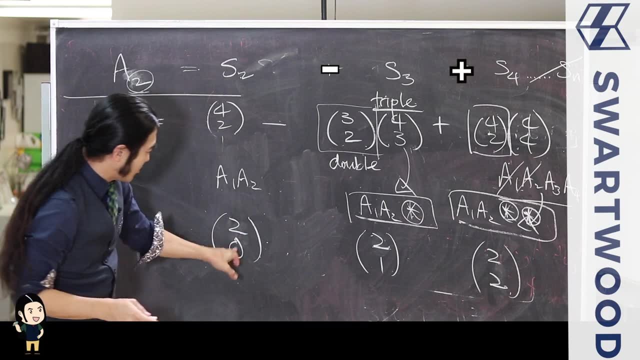 But how many of them do you need for that double? You need nothing, It's going to be 0. Does everybody see that? It's like if you have A1 and A2, there are two guys left- A3 and A4, but you're going to pull none from there. 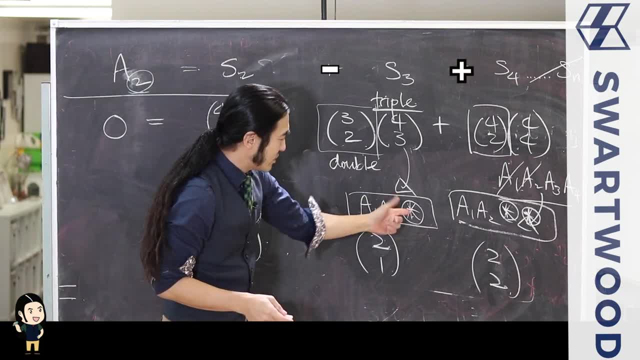 because you've got your pair. But for triples you put down A1 and A2, there are two guys left and you're going to pull what. You're going to pull one more to finish the triple And over here you have what. 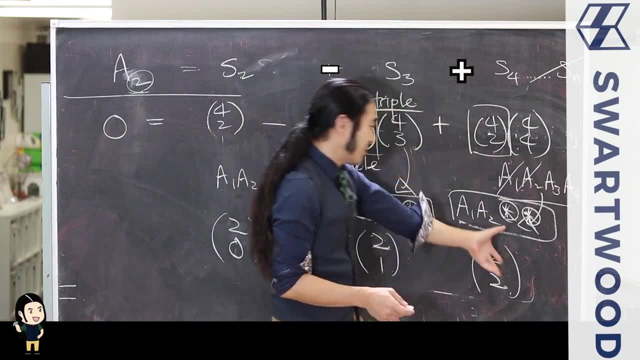 A1, A2, right, Two guys out there and you're going to pull both of them to finish that quadruple. OK, All right, it doesn't look so bad, So I think we're going to be able to finish here. 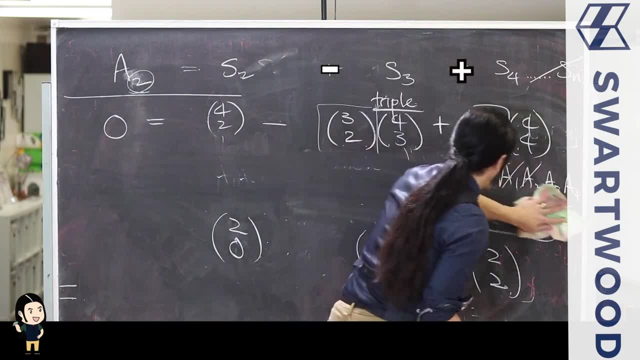 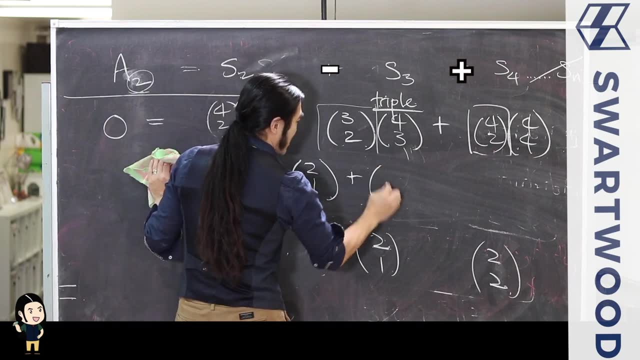 So let me clean this up One more line. So really the argument becomes so: 2 choose 0 minus 2 choose 1 plus 2 choose 2.. And now we use what we did in the previous proof, the general. 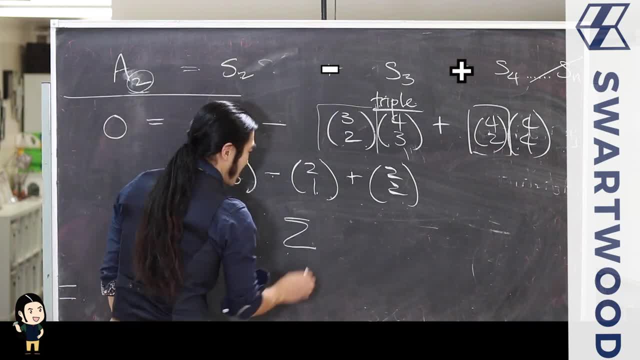 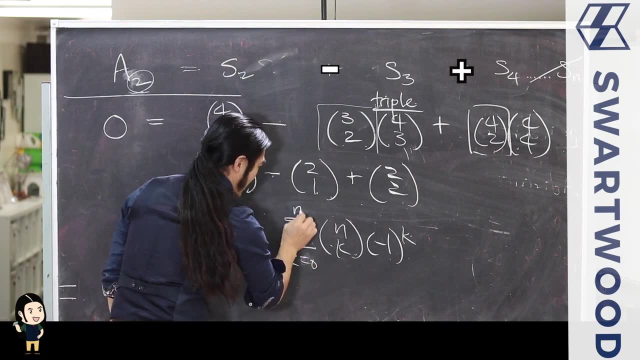 proof of pi. Remember the general proof of pi. if you sum some guy from n, choose k, negative 1 to the k 0, up to n- We did this already- That's going to be 0. And that's exactly this pattern. 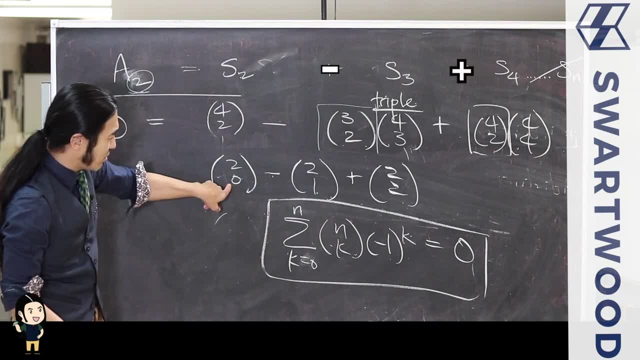 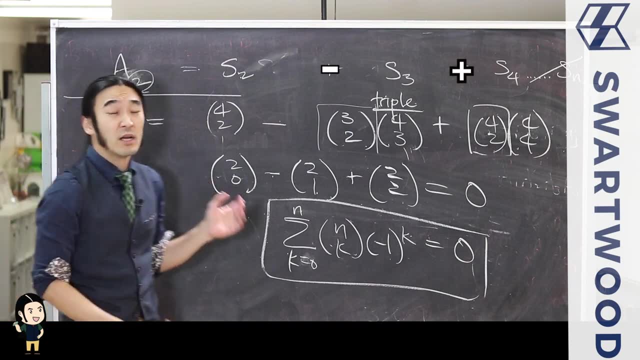 So we have the top fix of 2, and we run them from a positive with 0 up to negative 1, positive 2, like that, This will definitely sum to 0.. So the right-hand side counts 0, the left-hand side counts 0.. 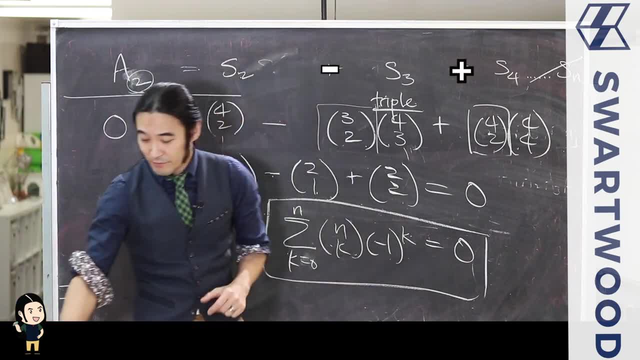 We know we're good, Does everybody buy that? So now we're going to do the same thing Now. it's just now that we have the idea and we have the inspiration. that was the key point of this. Where did these guys come from? 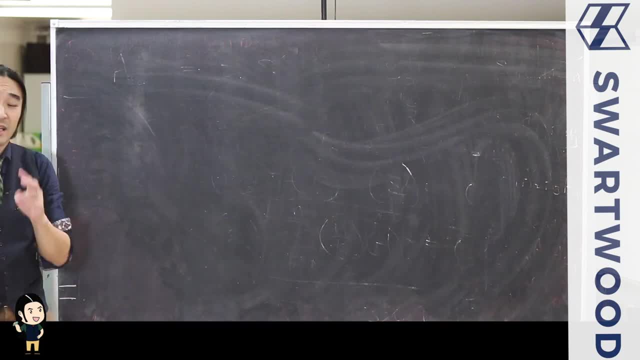 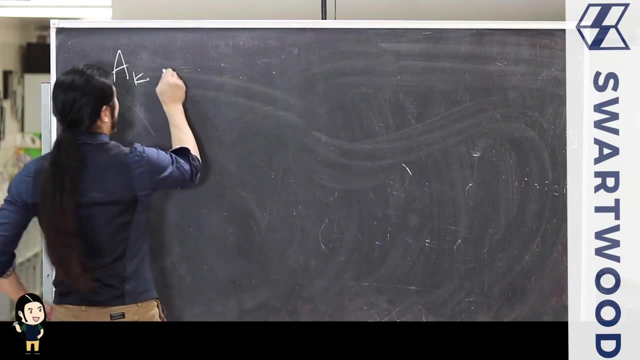 It's not that bad to do it in general, And I'm going to say this in words. So now we're looking at, let's say, there are n sets involved and we want the number in exactly k intersections. So if that's the case, where should you start? 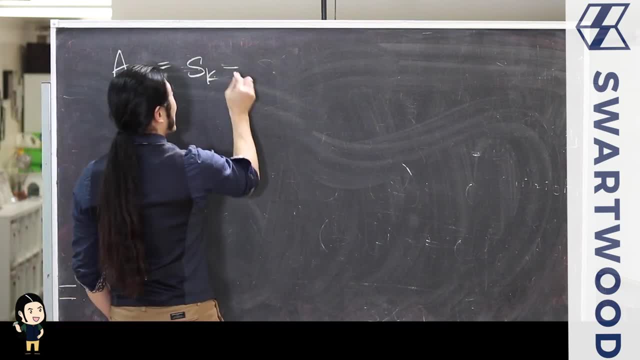 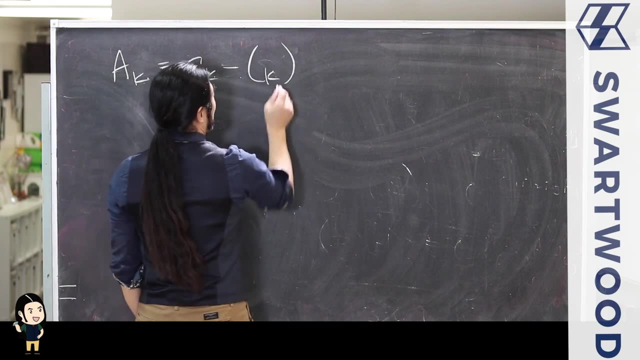 You should start at sk And these just subtract off. but now we're going to count now instead of in pairs or double intersections, we're going to count in k intersections. So we want the k intersections. The next guy up are k plus 1 intersections, right? 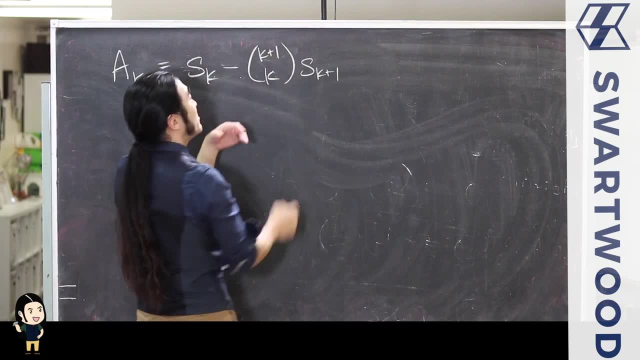 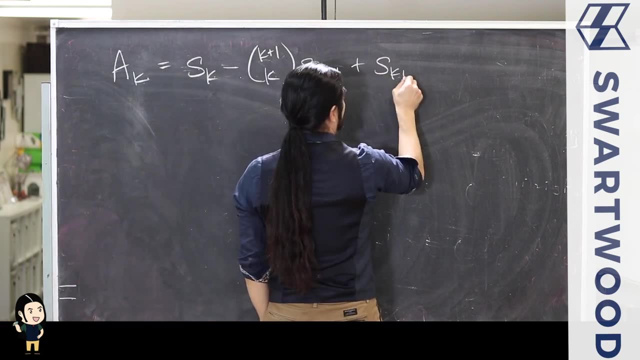 So you're looking at, out of the k plus 1 guys, you can choose k of them to be a k intersection. Does that make sense? If you look, this totally matches what we did before And now we're going to add. so let's say it's sk plus 2.. 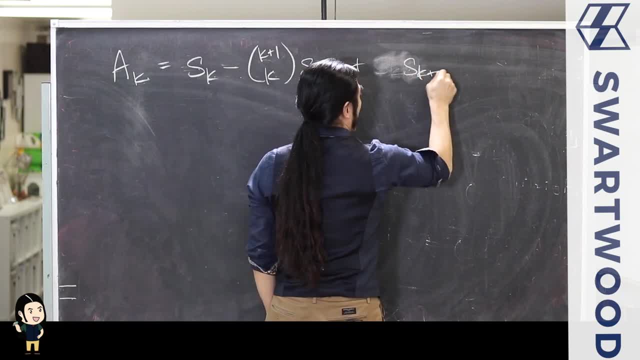 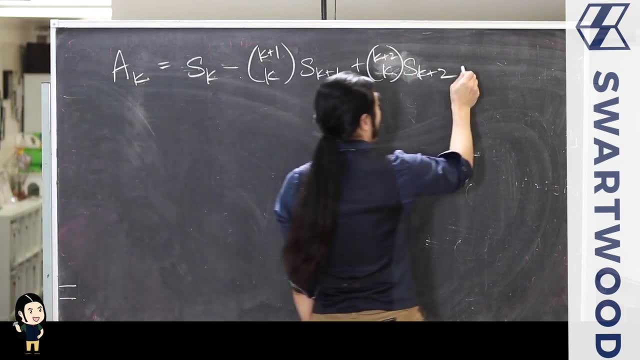 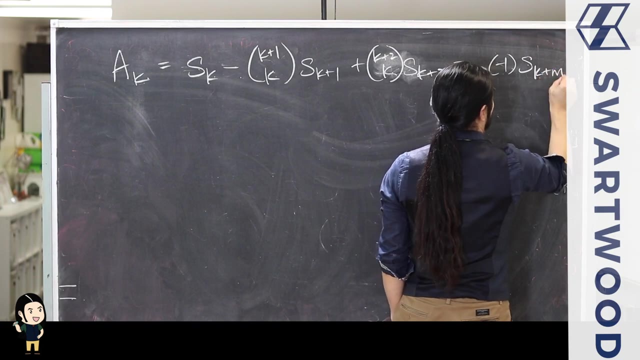 Oops, need room. There are k plus 2 guys. We're going to choose k of them for those k intersections And then we're going to go all the way up. So let's do the generic one. So, whatever the sign might be here- sk plus, let's say m. 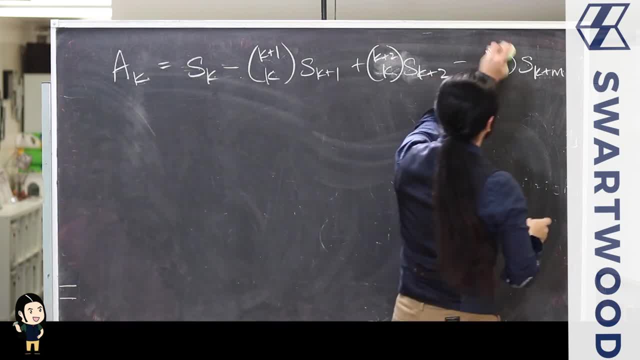 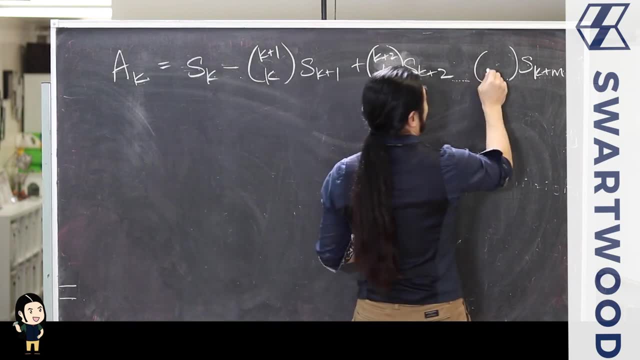 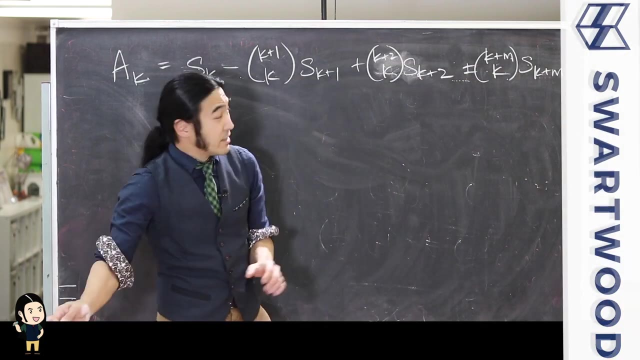 And then we're going to have over here. let's see, sorry, somewhere along the chain, here we're going to have. OK, Let's say k plus m. We want to choose k of them. right, It's going to have this pattern. 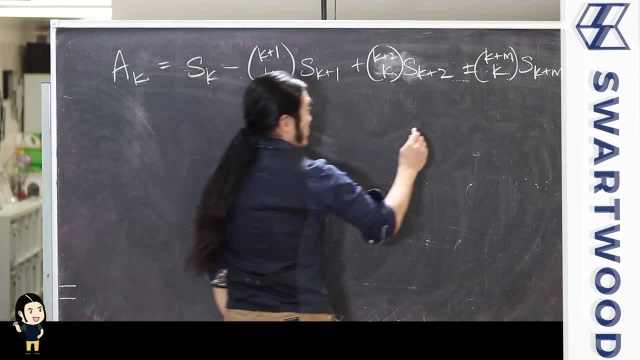 We'll figure out this sign in a second. It's not a big deal. And then we keep going. What's the final term going to look like? We're going to go all the way up to sn, even though we might not need to use it. 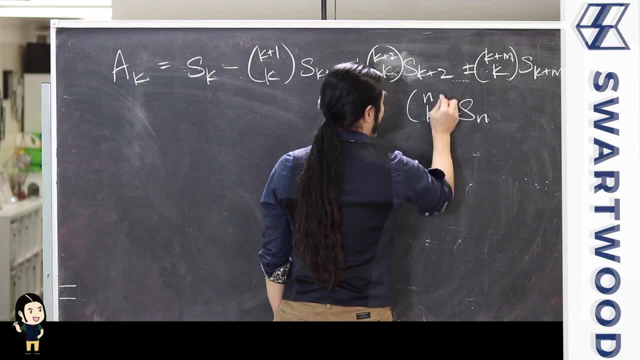 So we're going to look at this guy And it's going to be n guys. We're going to choose k of them again. OK, so what about this negative 1?? That's more like bookkeeping. The main idea was getting those coefficients. 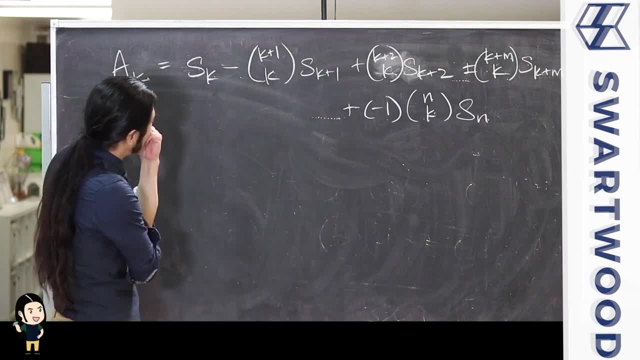 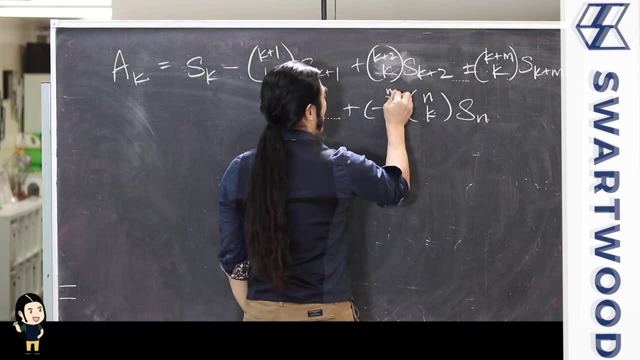 but we could do it now, Let's see. So if n were actually k, Then you want the guy to be positive. So I think maybe let's try this. Let's try n minus k. We could talk about where this comes from. 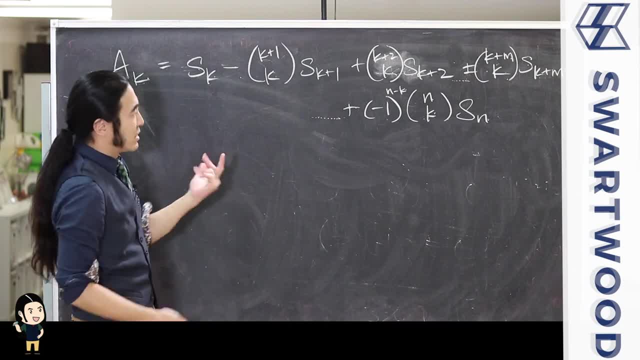 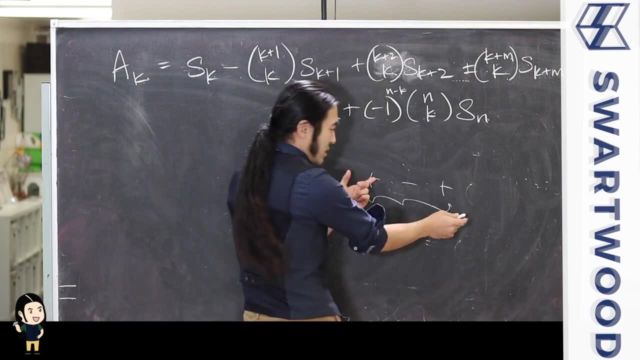 but this is just playing with flipping the signs. It's not the main point of this. But let's just test this idea. If n were say, because what's happening is you're alternating positive, negative, positive, like this, And whether you stop here or you keep going. 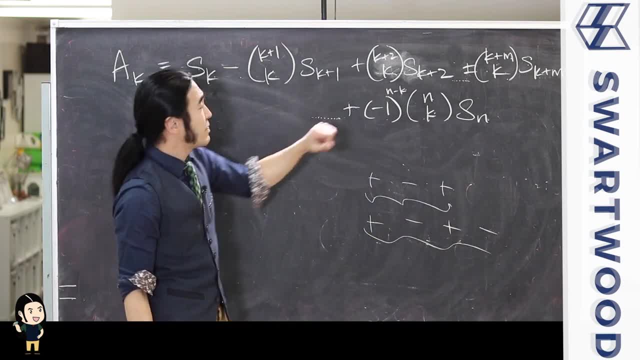 depends on how many terms there are. So now take the difference to get the number of terms. But now, if n were actually k- that's all we're doing- then it would be negative 1 to the k minus k. OK, 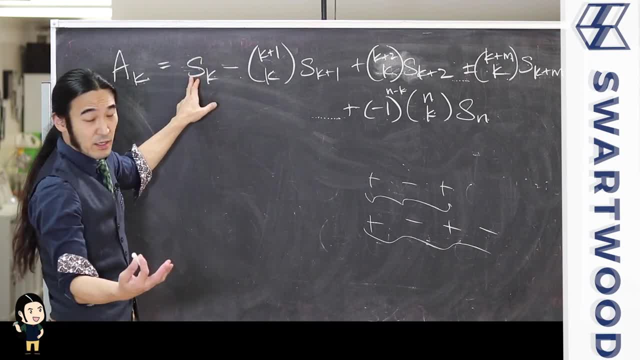 But then that would end up being what? Negative 1 to 0, which is positive 1.. That works. What if we ended up going to here? Then it would be well, n is k plus 1. And you're going to subtract off k. 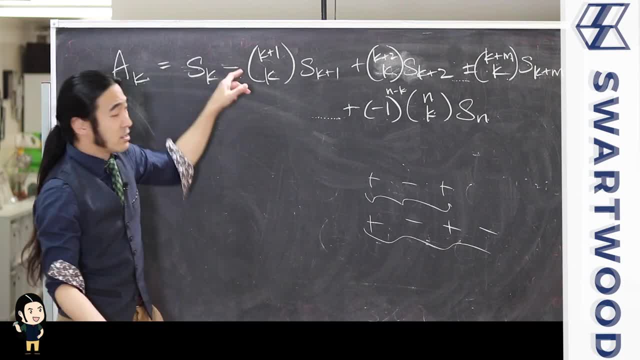 That would give you 1.. Negative: 1 to the 1 is going to be a negative And that works too. So this power right here totally works out. Let me know in the comments if you want to talk more about that. But again, that's kind of peripheral to what. 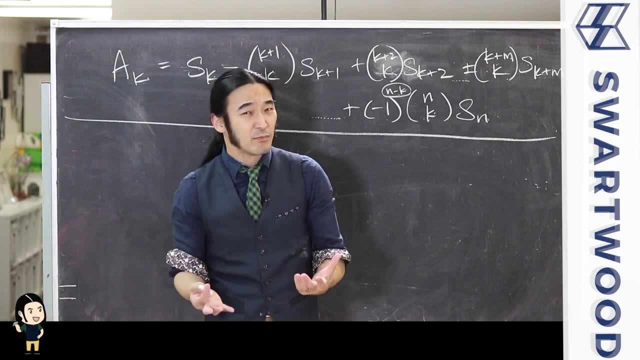 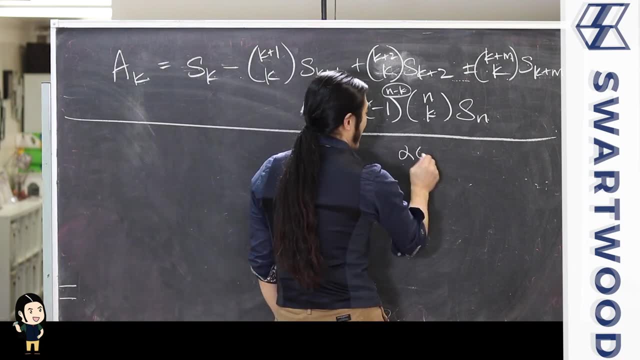 we're really going for. So I want to go for this pattern. So here's our basically complete proof: just a little bit mellow and kind of informal, But the same idea. You look at an element, alpha- An alpha might be an intersection of, let's say, 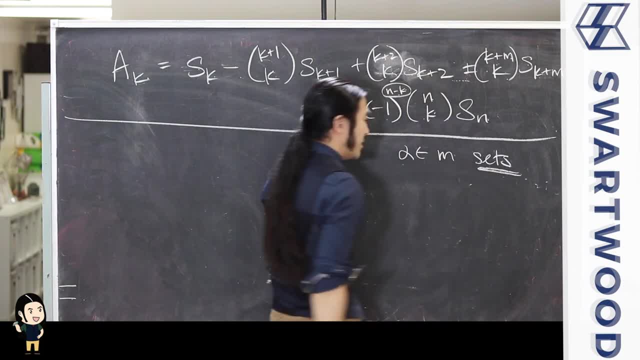 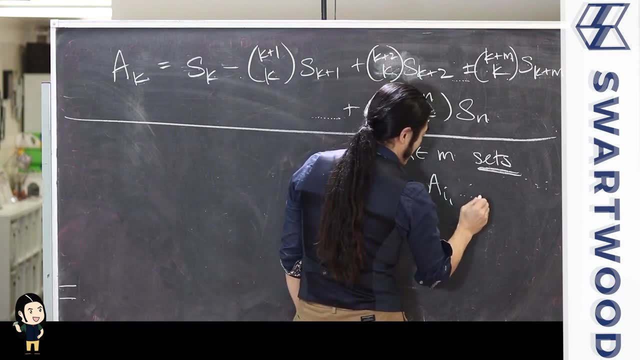 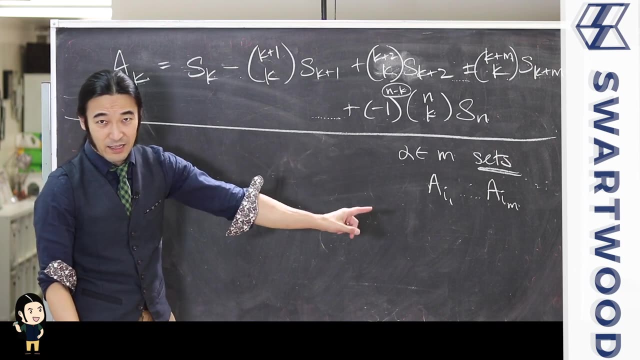 m sets OK, And you could designate them. For example, you might designate them alpha i. This is where it gets really tedious. a, i 1 up to a. i m assuming that your sets are labeled. say a 1 to a n. 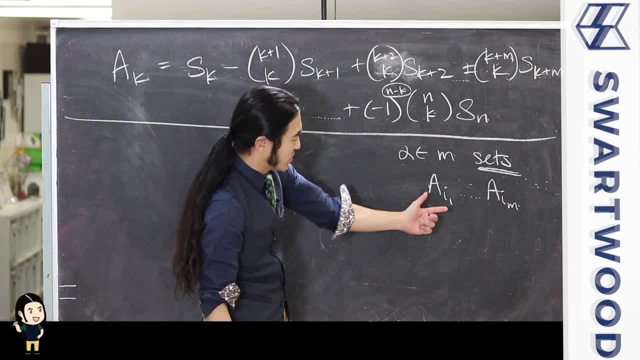 The reason why I'm putting the i here is it doesn't have to be a 1.. It might be a 2. But we're saying there's m of them. Again, that's not so important. The main point to pick up here is that alpha is: 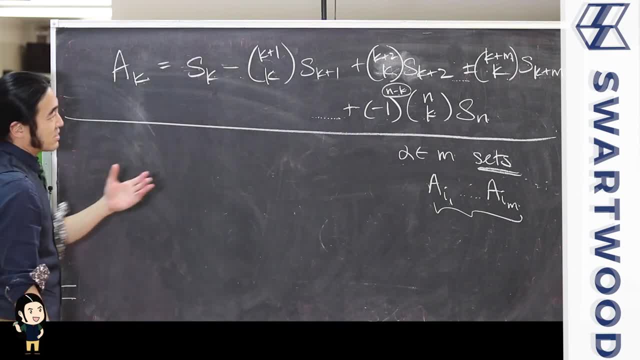 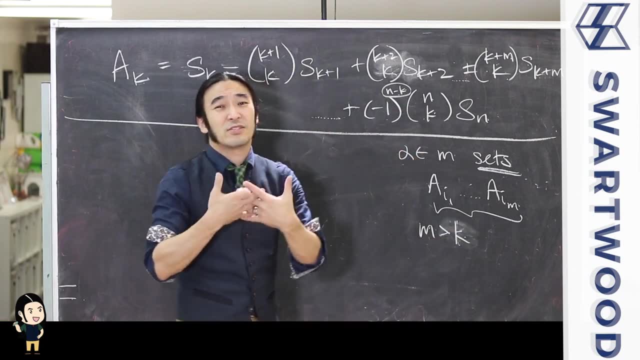 in m sets exactly. Well, if an alpha is in m sets- and of course I'm going to assume m is greater than k, If m is equal to k, then it's in the intersection of exactly k sets. It's kind of once here. 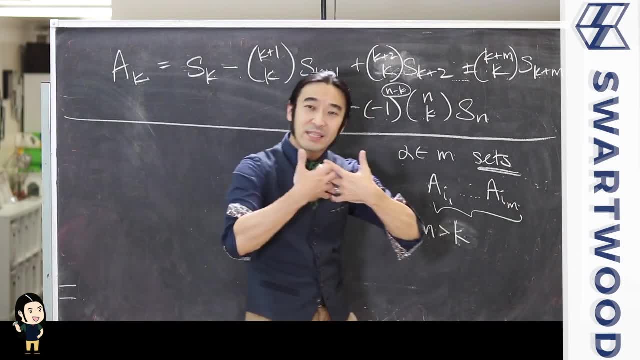 It should be kind of once there, And then these other terms even apply, because it's in k sets, not k plus 1 or k plus 2 or k plus 10.. The only issue is when you're out there and this guy is greater. 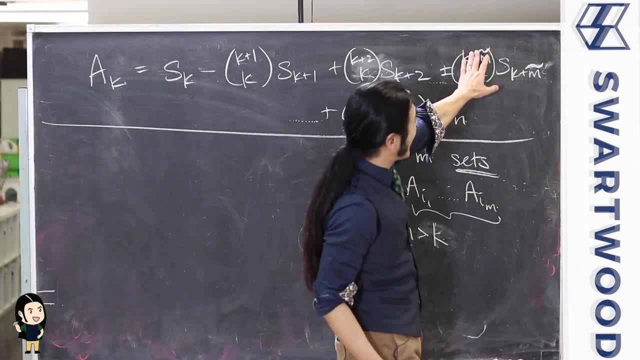 than k. OK, Oh, my bad, I don't want to confuse anyone. I don't mean that that m is the same as this m. I just want to give some arbitrary guy here And I thought m was a good letter. 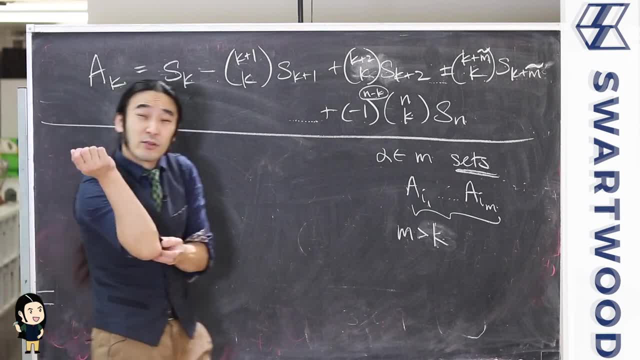 OK, So let's go with that. OK, All right, My bad. We can always come back and do it more cleanly if you want, But I think the main point is just to get this idea out there. OK, So we have this set up here. 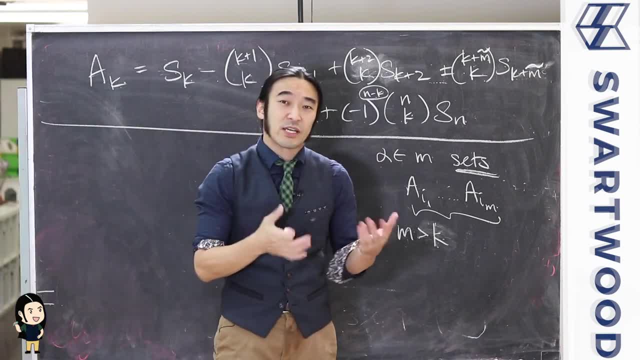 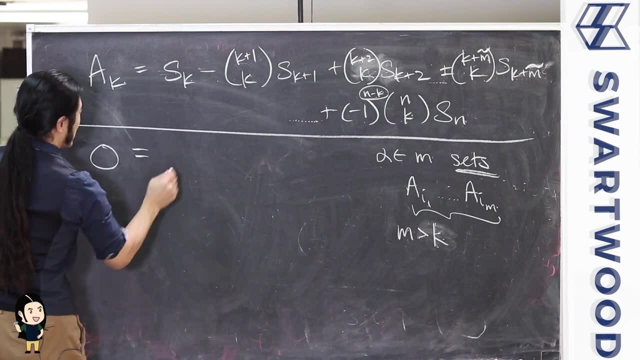 Now if m is greater than k, that means it's in the intersection of m sets, So it's not in exactly k sets, So it doesn't belong. So on the left-hand side it would be counted 0 times. Now the question is how many times? 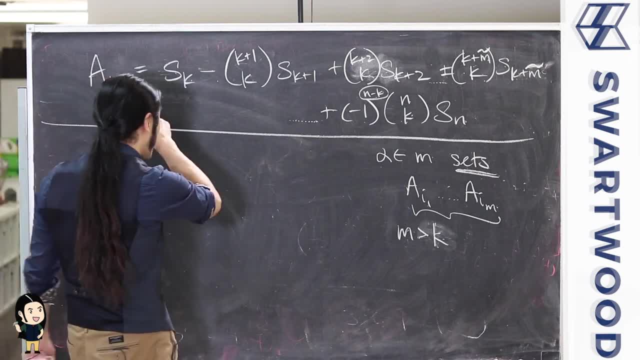 would it be counted on the right? Hopefully it's going to be 0.. OK, All right, But in the k guys here, right in the k intersections, well, if you're going to get a k, you're in exactly m sets right, then it's a fact. 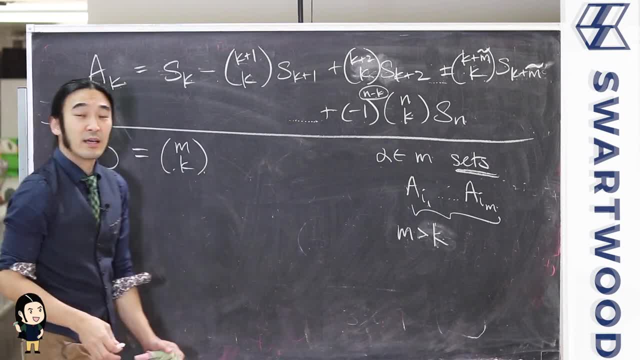 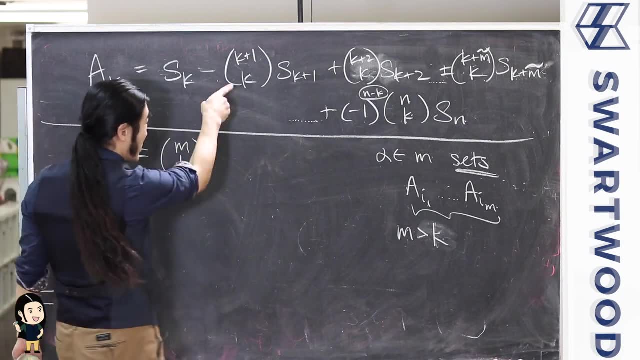 that you'll be in. m choose k, k intersections, Because that's how we get all the k intersections that contain this guy alpha. It's literally: you take your m guys and you pull out k of them. OK, Now let's go to here. 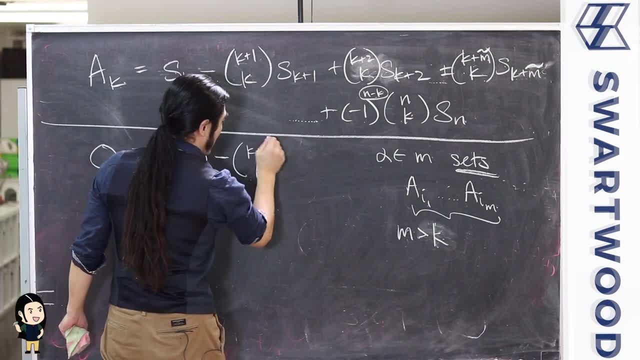 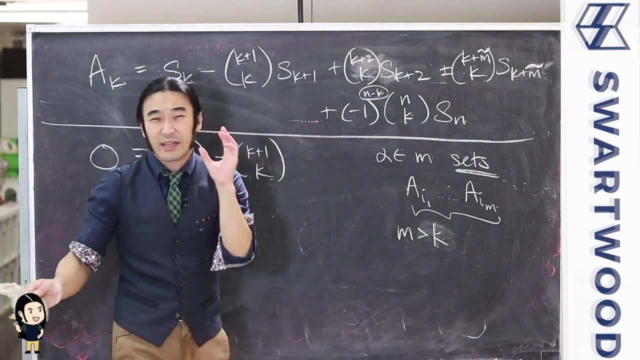 Now we're actually going to put in this coefficient we've artificially constructed, OK. So now, what about k plus 1?? Well, again, what's going on? If you look at the k plus 1 intersections that contain alpha, how many of them are there out there? 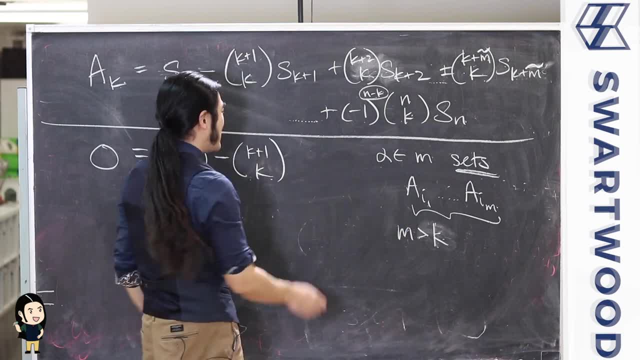 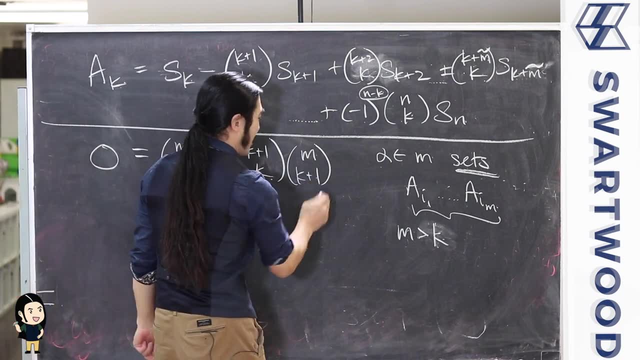 Well, Alpha sits in m guys, right. So alpha sits in m sets, And so you're generating all the k plus 1 intersections by taking k plus 1 guys from that m. So this is just like before, when we're doing the whole triple. 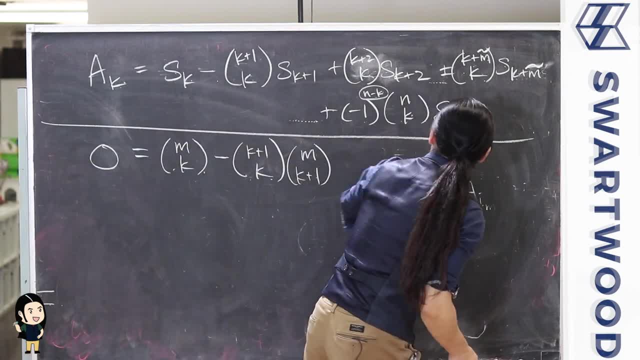 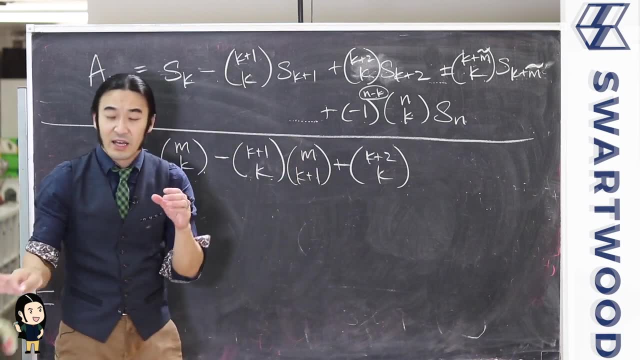 intersections. right? How many doubles do you get from that 3 choose 2.. Let's do a couple more to make sure we're good. So I'm just copying down this coefficient And I think about this: If you have k plus 2, how many k plus 2 intersections? 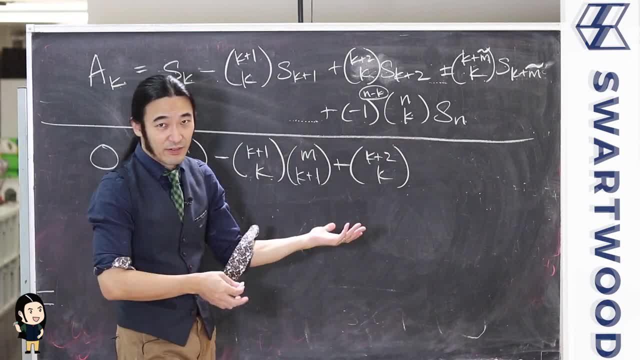 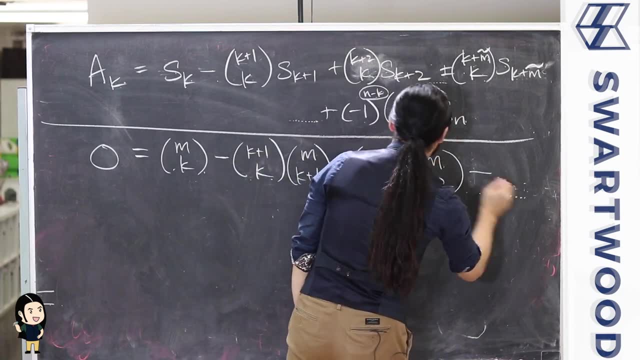 can you get from the m sets right or the m sets? OK, If you contain alpha, there will be m. choose k plus 2, OK, And this procedure keeps going all the way up to the. well, we don't have to go all the way to n. 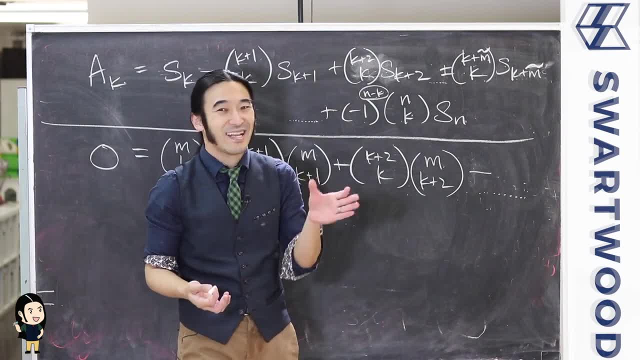 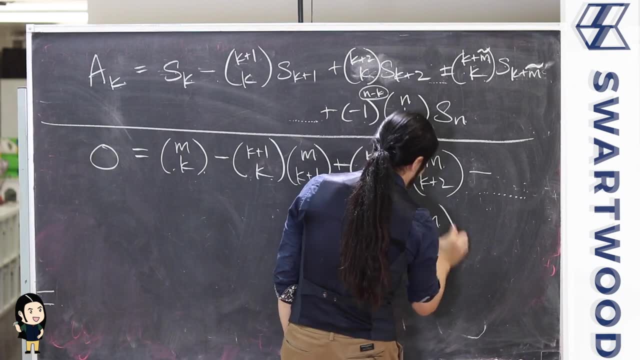 because the biggest intersection alpha sits in is an m intersection, not n. So that means we're going to go up to this guy: m choose k. right, And this is going to be: m choose all m like this, OK, And the sign here is going to follow the same pattern. 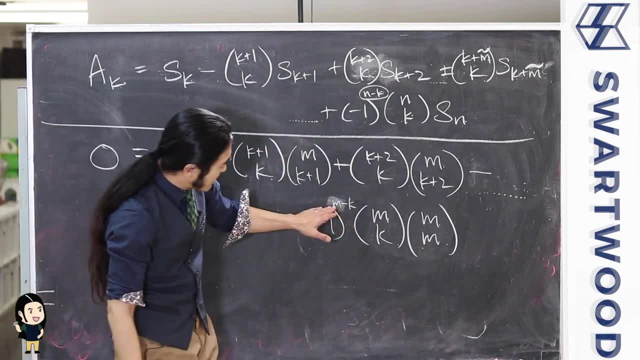 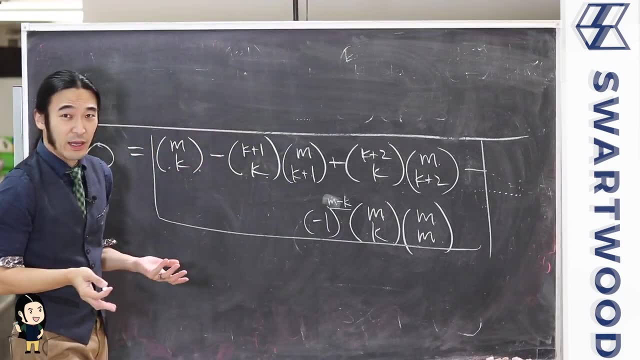 It's going to be again. this is going to be m minus k. This sign is flip-flop and it lands on the right thing. OK, so if someone actually gave you this identity, you could actually argue it this way: 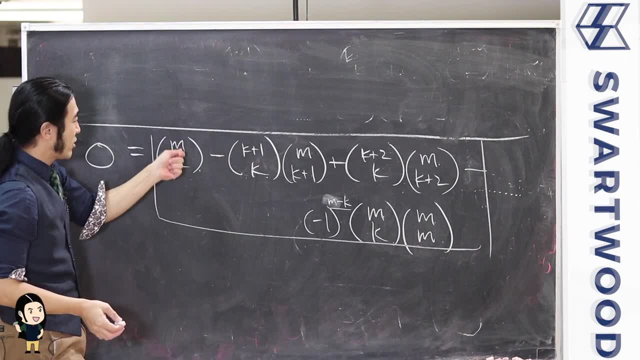 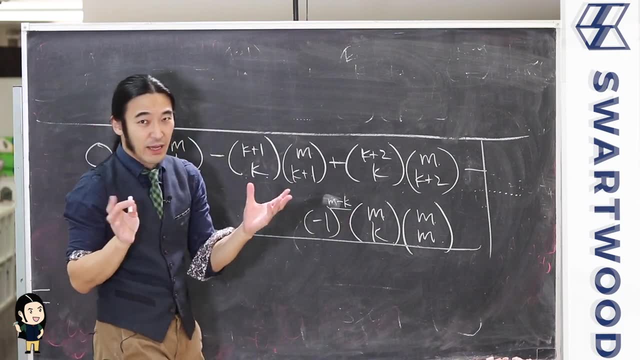 So we can imagine that this guy counts basically of m sets, right, and we're looking at the k intersections. OK, So you've got m sets and you're looking at the number of k intersections and then to contain a certain guy, 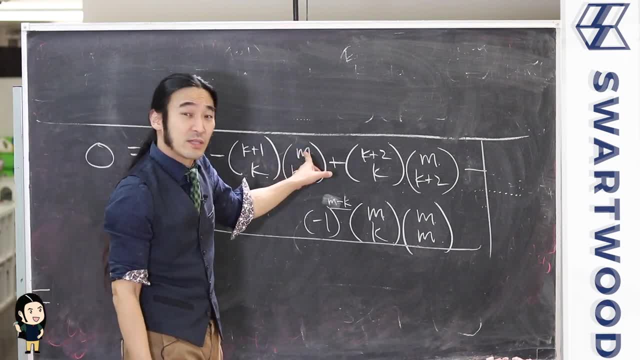 And then over here what's happening. Well then, you're looking at- we're going to do the same thing- We're going to look at those m sets and pull out how many k plus 1 intersections we have, And from those k plus 1 intersections, 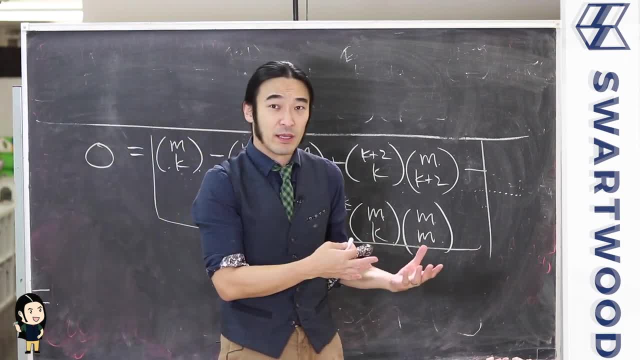 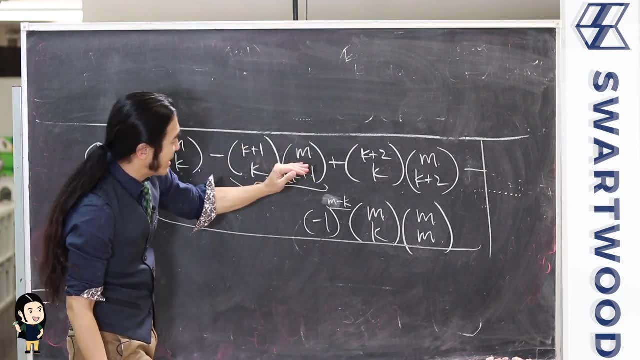 we'll see how many k intersections can be generated from them. So when you multiply these two guys together, this is counting the number of k intersections that we can get when we first pull out the k plus 1 guys and then generate for them the k intersections. 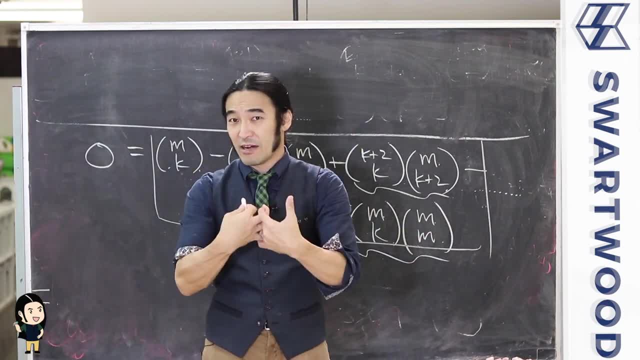 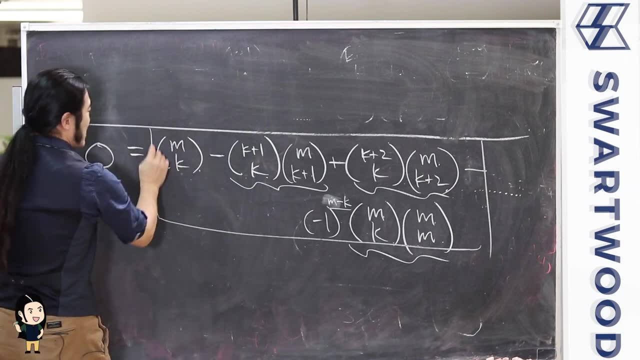 Same argument here. same argument here. only looking at the guys that contain alpha. OK, All right, so what's going to happen here? Well, let's count up the difference here. Let's say: this number counts what we want, correctly. 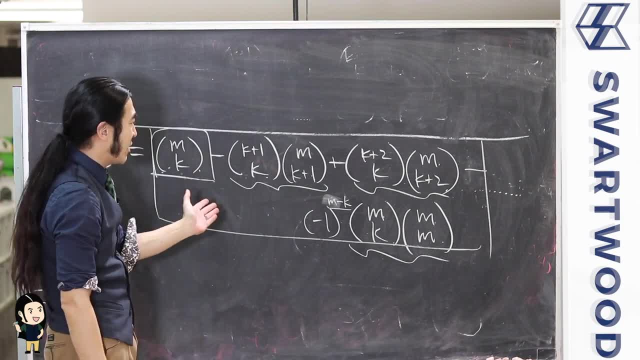 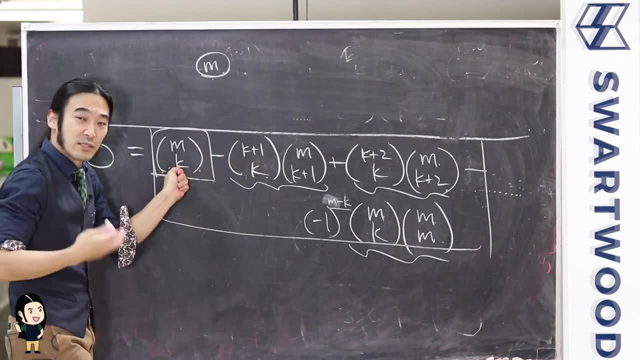 Then over here we're going to overcount. But how many ways can you overcount? Because first you want to look at the number of k guys. So they're m guys alpha There, OK, so we want to see if there's repetition. 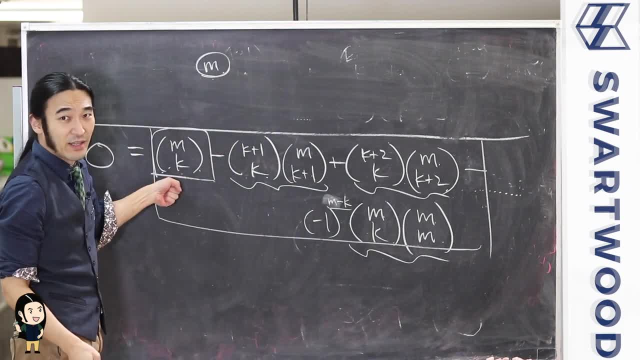 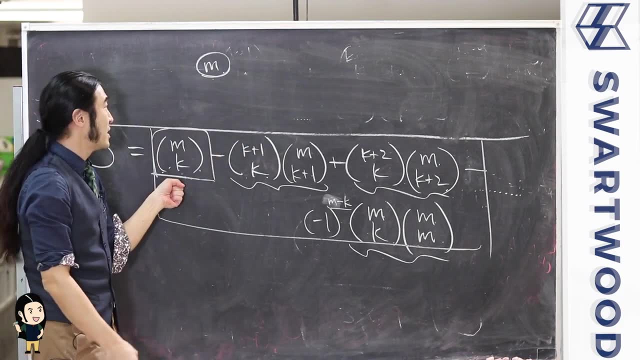 So for any given k intersection or a collection of k guys, you can think of it that way- how many guys that are k plus 1 can generate the same k guy over here? So how do you do that? You go back up here. 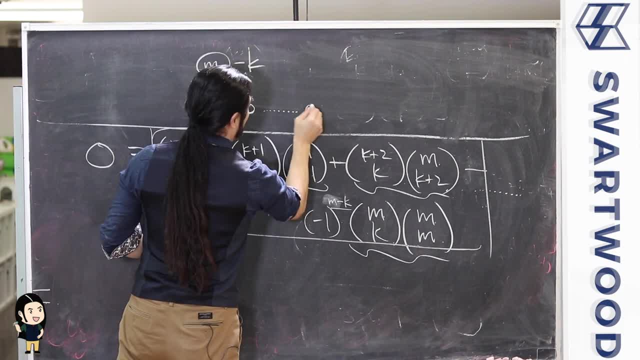 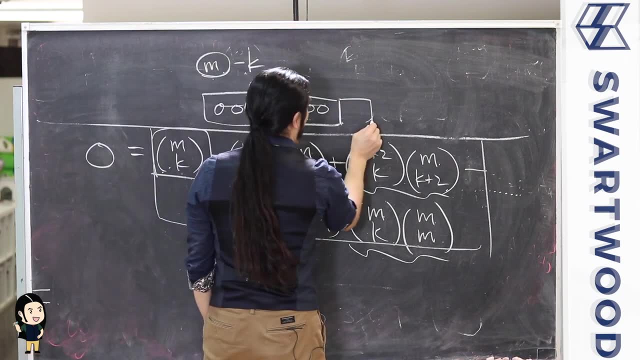 We need to first put our k guys, whatever they are, place them down. But now we're looking at what We have our k guys right, And then we want to look at: so these are our k guys. We want to look at this extra one right here, right. 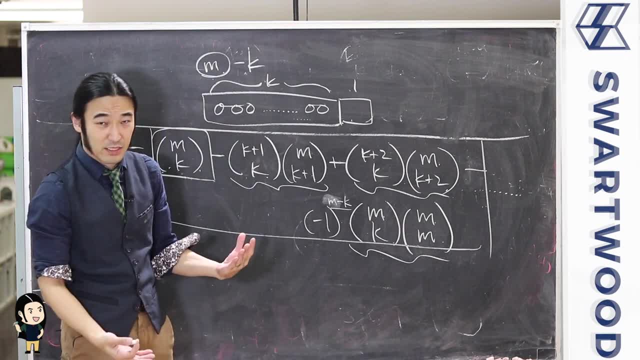 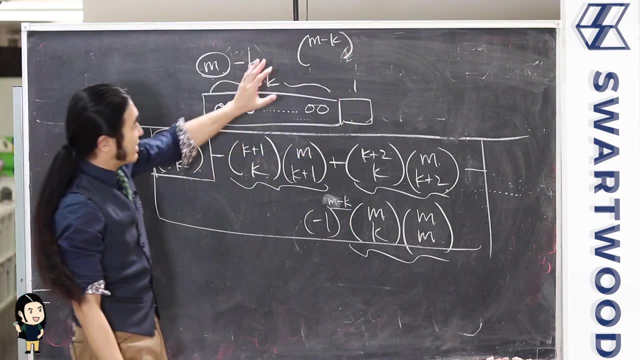 Because we're looking at all the k plus 1 sets. So this combined will generate the k plus 1 sets. So how many ways can that be done? Well, there are m minus k guys out there, right, OK? and of the m minus k guys out there, how many are we going to pick out? 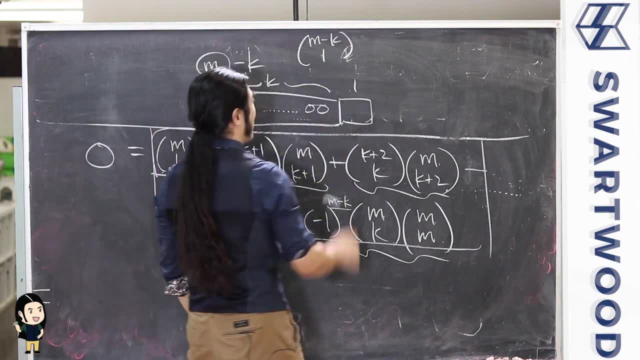 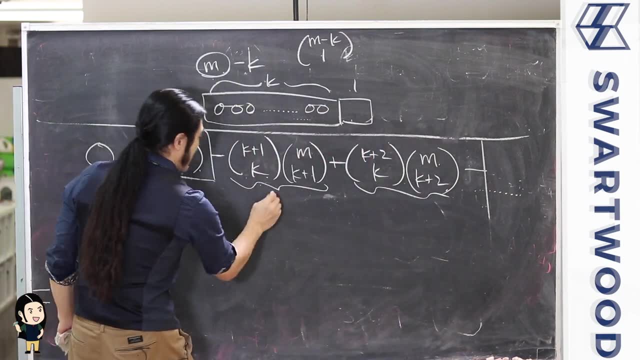 to push this k set up here to k plus 1 set up. We're going to choose 1, OK, So the number of overcounts here- let me erase this, so you get the idea- For this thing it's going to be m minus k. 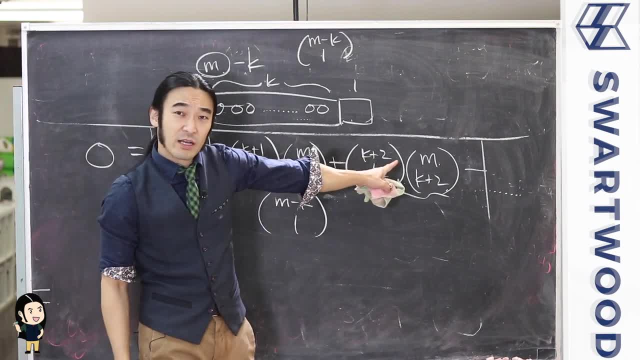 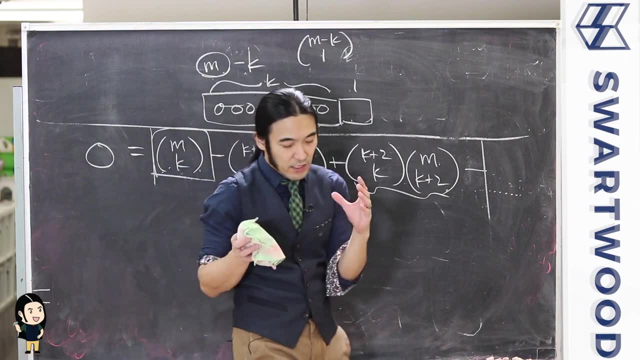 M minus k, choose 1.. Now over here, the same thing. So what you do is you pull out the k plus 2 guys, right, And then we generate from them the k guys. OK, So then, how many ways can this be done? 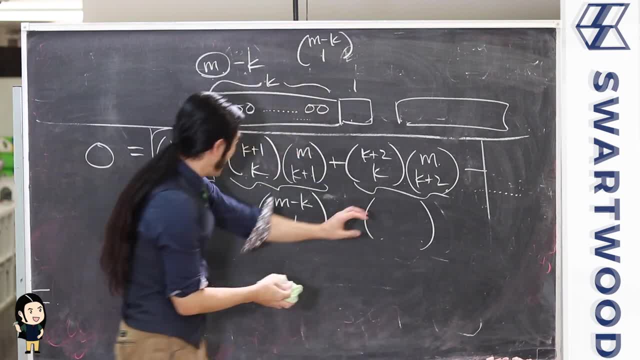 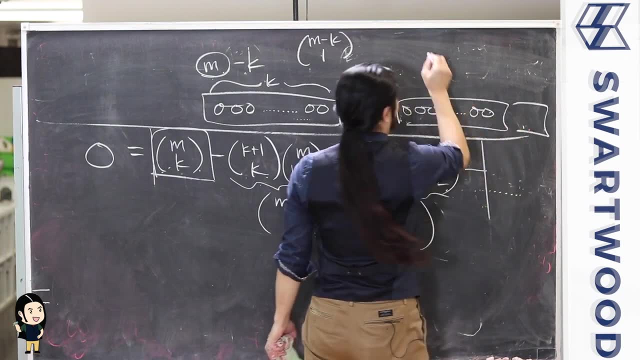 Same argument, All right, so same thing here. So we want to have our k guys because we're aiming to see redundancy on a specific given k intersection. So here's our guy. OK, And again, if you remove k of them, you have m minus k out there. 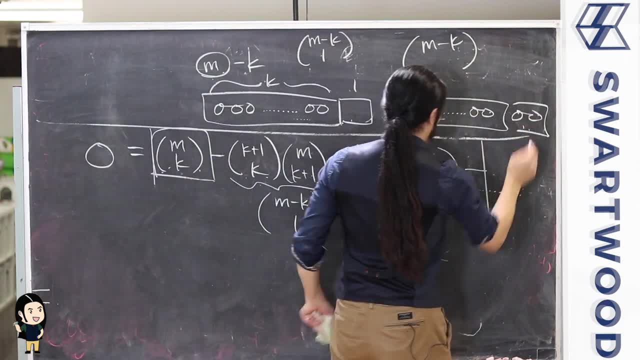 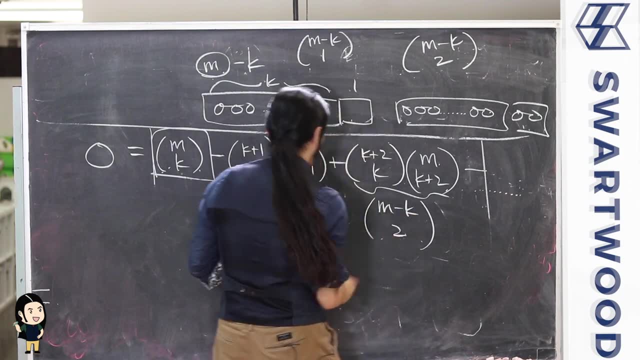 How many do we need to pick out? to finish this up, We need to pick out 2. To get our k plus 2 guy right, OK, so if we do that, it's going to be m minus k, choose 2.. 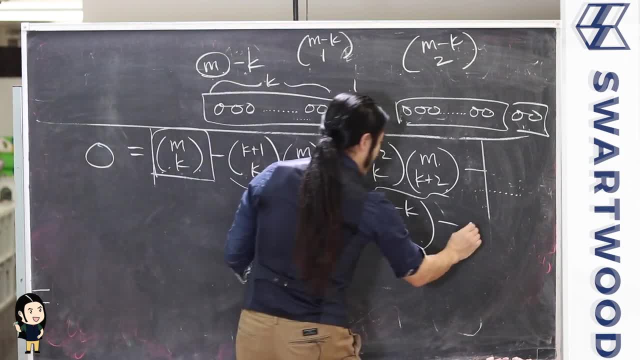 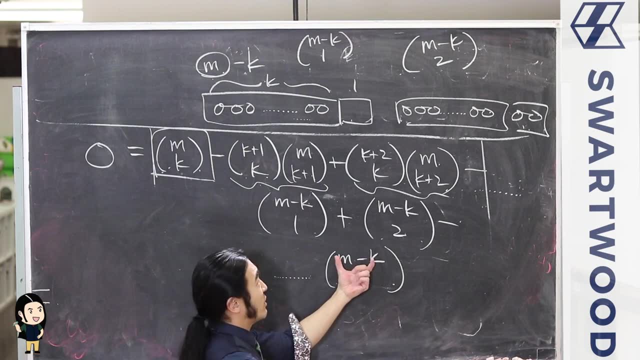 And here it's going to be a plus, OK, OK, Et cetera. So you can see the argument holds all the way up. When we get to the final one, it's m minus k. guys here, right Again, starting off the same way. 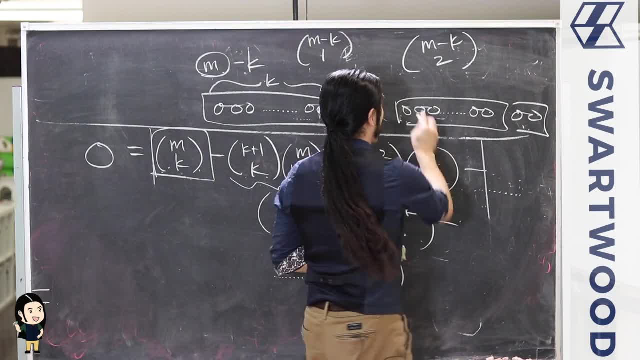 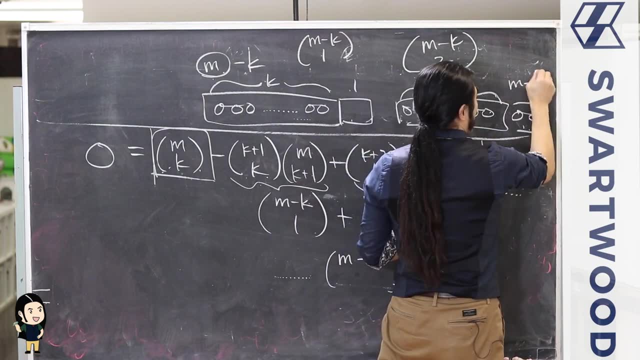 But now you need to finish up, You need to flush it all the way out. So we've chosen k guys here, and we're going all the way up to m. If the whole thing should be m and this is k, then this is m minus k. 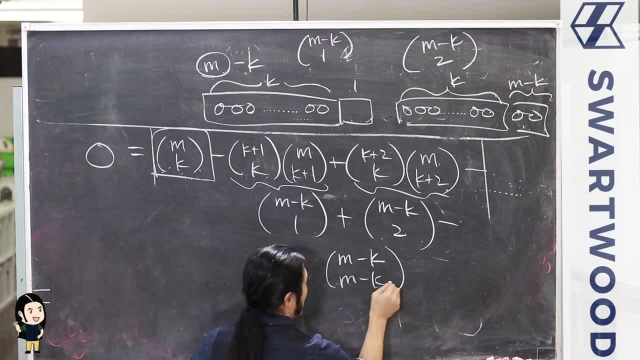 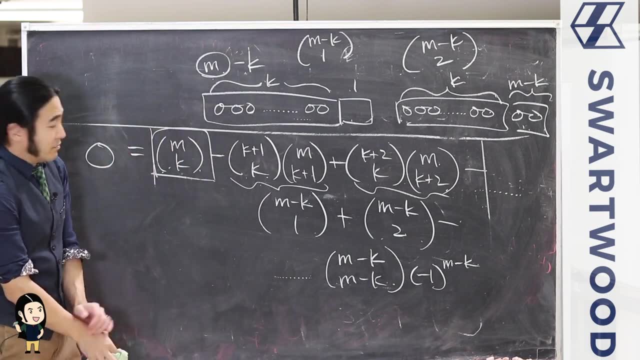 So this is actually going to be m minus k, OK, And of course put the negative 1 to the m minus k. OK. All right, not a big deal. So again, if it bugs you, we can talk about what this thing means. 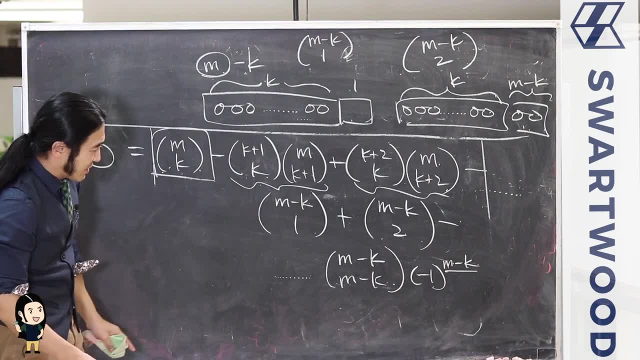 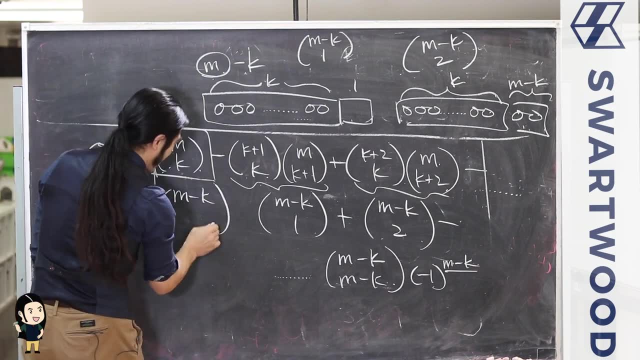 But that's just a mellow trick, All right, so now are we done with this. Well, don't forget this term. We've got to put this back here Now. you could write it as 1.. But you can also think that: well, if you're looking at a k set, 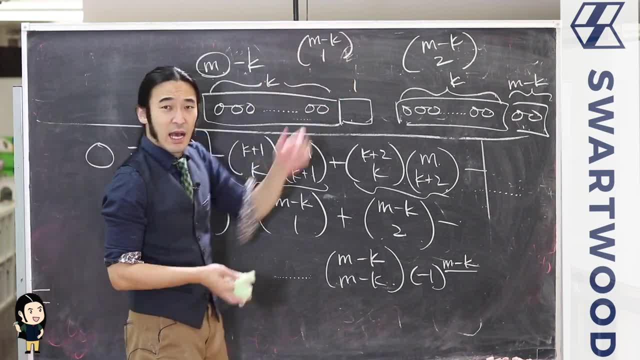 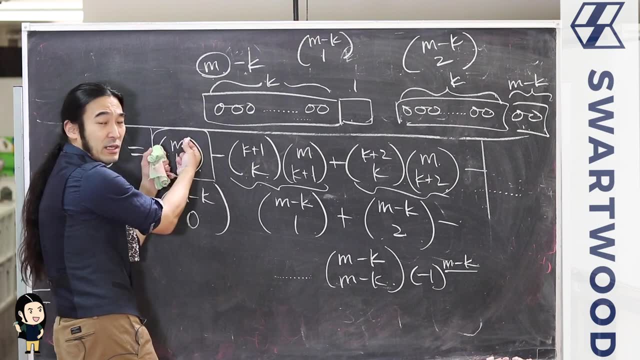 and we've chosen k guys. how many are left over m minus k? How many are we going to pick? None of them, That's equivalent to 1, though right, OK, because remember, the guys that are counted here are counted properly. 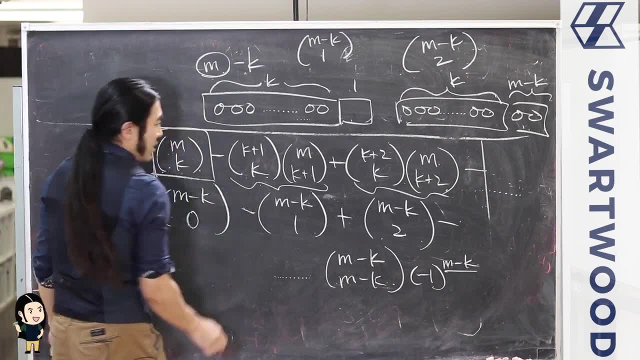 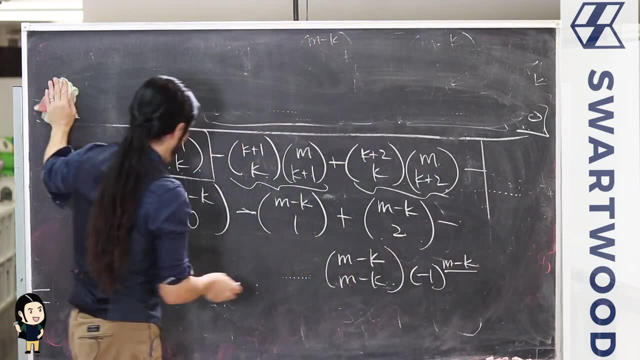 So for any given guy, you're counting him once properly. OK, But then what does this boil down to? Well, m minus k doesn't change, It's a fixed number, right? All right, so we're basically done. We want to know what does this sum to? 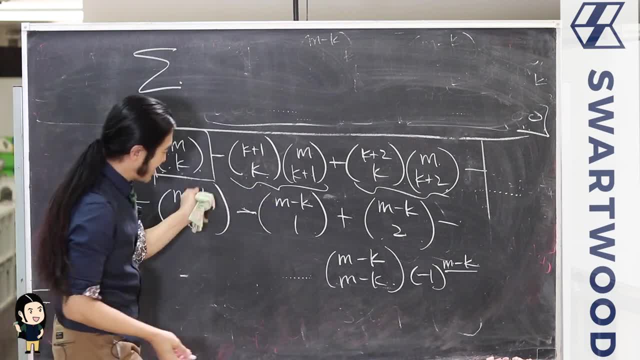 So let's rewrite this So you can definitely see. it's the same pattern, It's a fixed guy and we're letting the bottom go from 0 to 1, and we're altering the signs all the way up to m minus k. 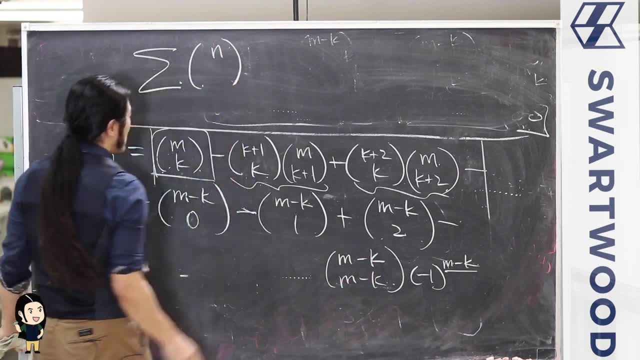 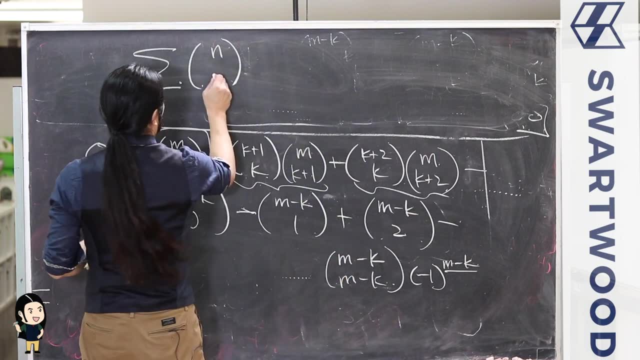 So I think we're good, But let's write it right. Let's write it like this: n choose. typically we use k, but since k is already taken, let's use a different letter. Let's use like phi. Why not? OK? 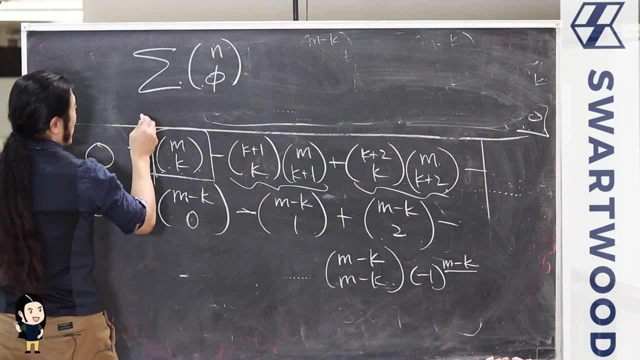 Phi or phi, depending on how you want to pronounce it. So we're going to use this guy, OK, so now, where is this guy going to go? Well, this part's easy. It's going to go from 0 up to m minus k. 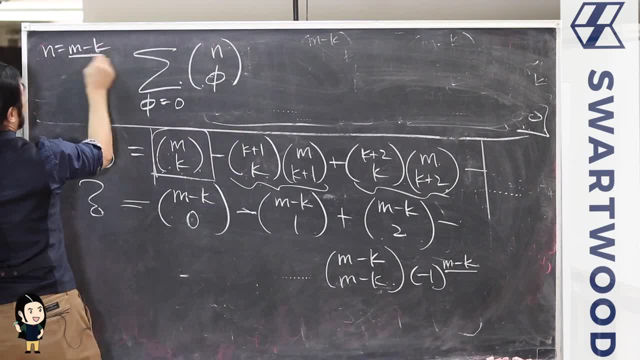 But we're going to let n equal m minus k. You don't need to do that. You could put m minus k, It's totally fine. But it's just a fixed number, It doesn't change, And you're going to go from 0 up to that number, right? 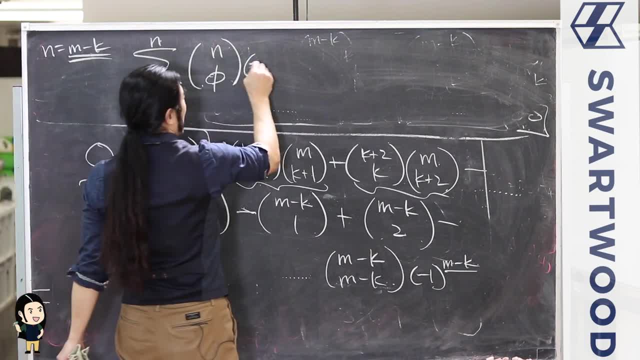 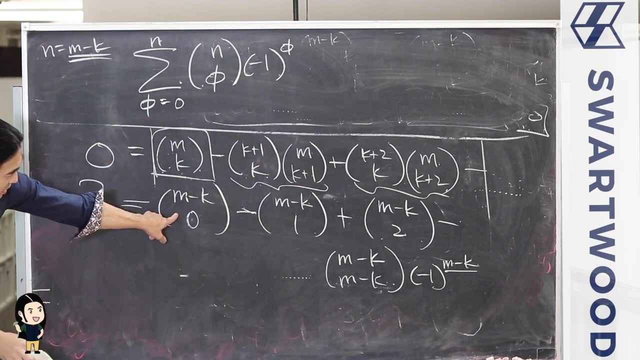 So it's going to go from 0 up to n- OK, And we know it's going to alternate. It's going to alternate from what? OK, Because it's going to start at 0 and then go to 1,, 2.. 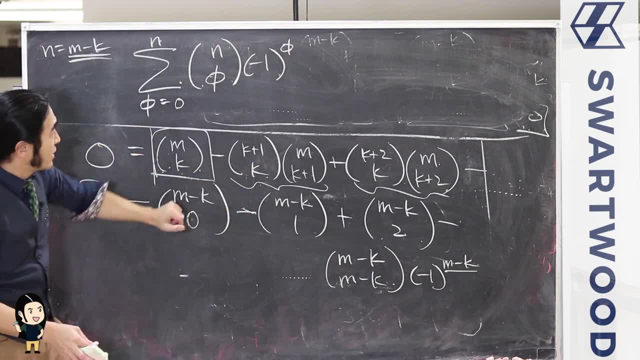 This works right, Because negative 1 to the 0 is 1.. And then negative 1 to the 1 is negative 1, et cetera. Positive 1, negative 1,, all the way down, OK. 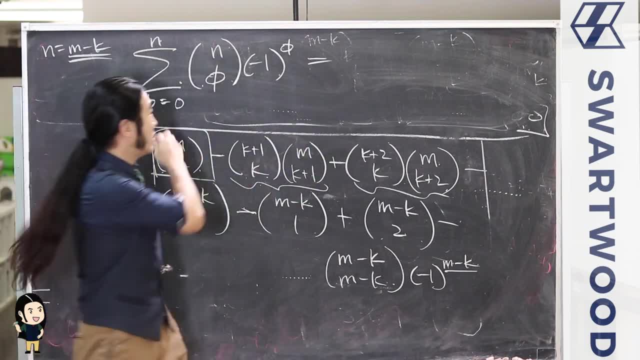 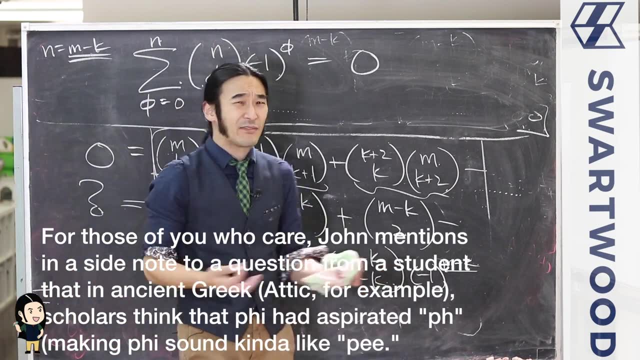 And this guy we know from before, right From the general pi thing. We know that identity is definitely 0. So we know it works out. So that formula we had up there actually counts it correctly. Now, if you ever have to bring this back up on command, 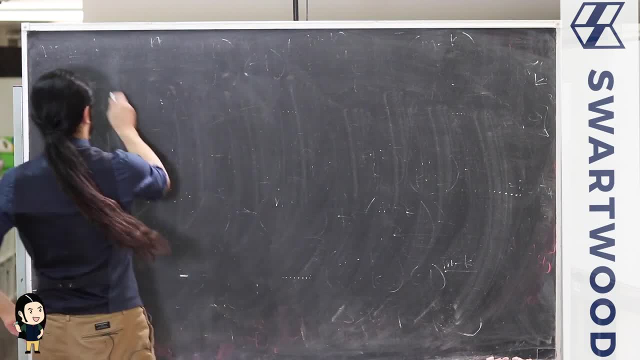 that's why I like thinking of it this way. It's very mellow, You don't really have to memorize it Because, again, if you're looking at k sets right, You know we're going to start at sk, sk plus 1.. 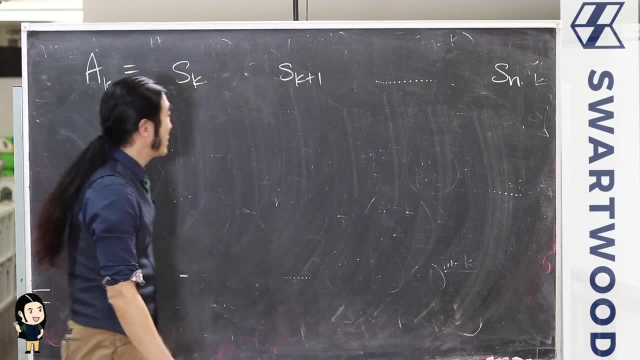 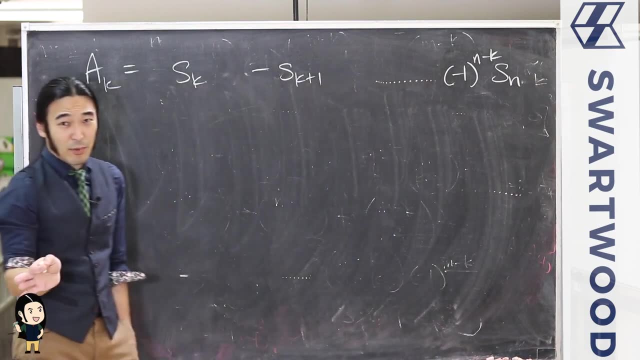 And you know we're going to go all the way up to sn. OK, We know the signs are going to alternate And then we'll talk about this later, if you want. This is going to become n minus k. OK, I get that part. 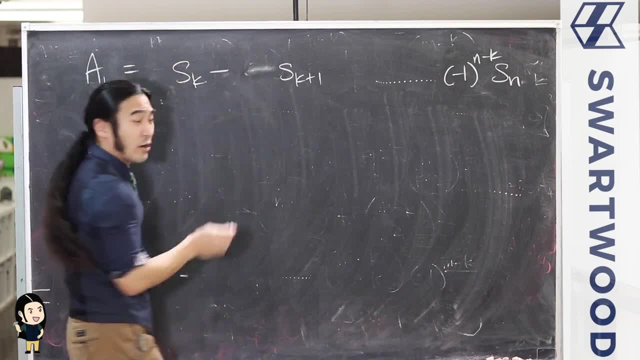 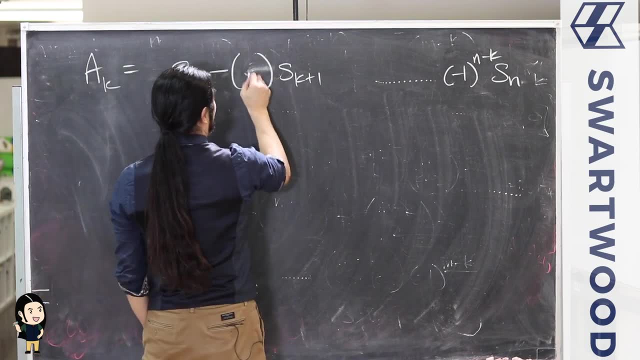 The tricky part is: what about the coefficients? But remember how we argued this. right, We're actually looking. We're looking at or counting the what, I guess the k intersections. So you want to pick out k guys here? You want to pick out k guys here? 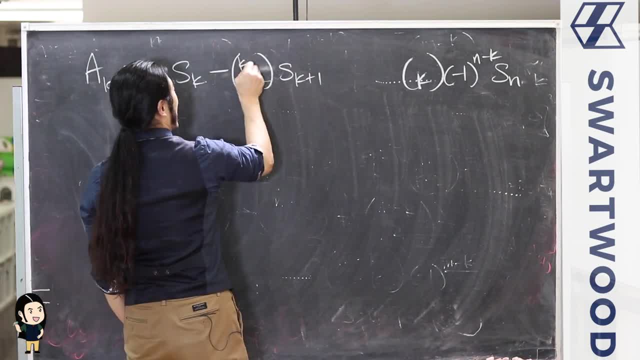 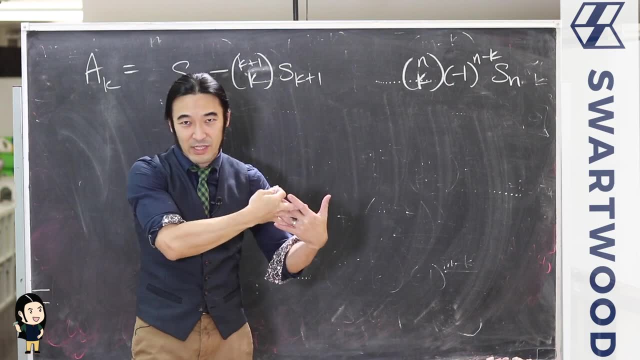 But from what? From over here, the k plus 1 intersections. So from the k plus 1 intersections And from here from the n intersections? OK, Meaning the intersections where n guys are intersecting. Does that make sense? 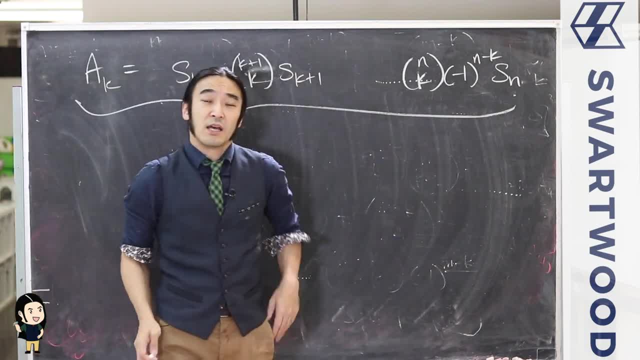 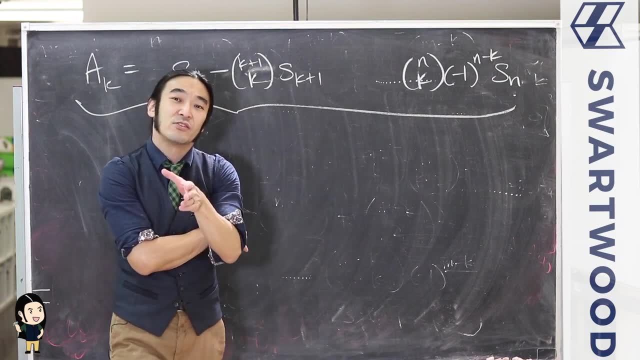 OK, So this totally works. There is another one that doesn't count exactly the number of elements in k intersections. It actually counts the number of guys, It counts the number of k intersections or more. OK, And that one is actually the true general form of pi. 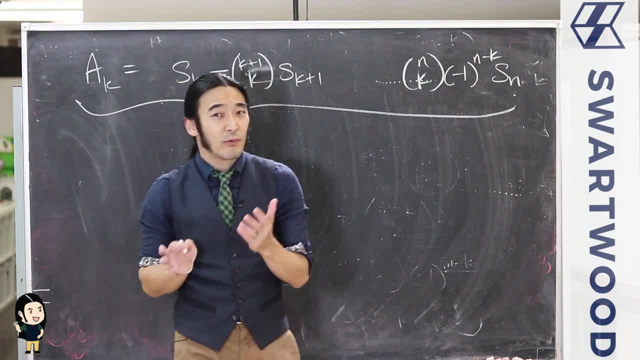 Because when you set that k value to be 1, you get pi back. So if you want, we can do that. There is a way of seeing that that's similar to this, Like the way when I was thinking about it. 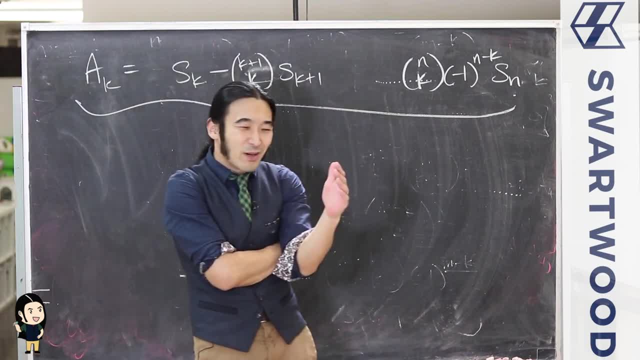 like, how can you put it together? You can't actually visualize it that way, But that one is kind of layered And it's OK. It's not bad if you want to do it, But I figure, if you convince yourself with this, 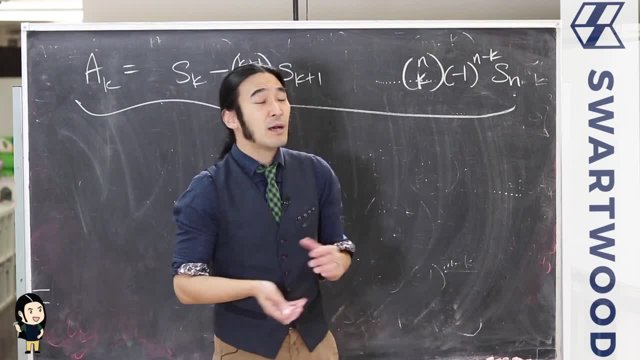 we can do a much smoother argument- Not super slick, because I want to give it some intuition, But there is one that's pretty good that will use this and basically solve and get the general case OK. So we can hopefully do that next time. Please let us know if you have any questions. 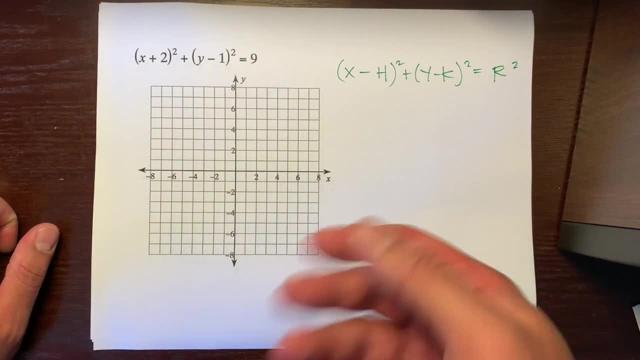 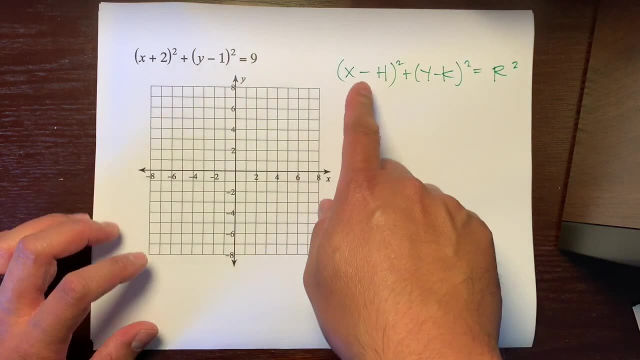 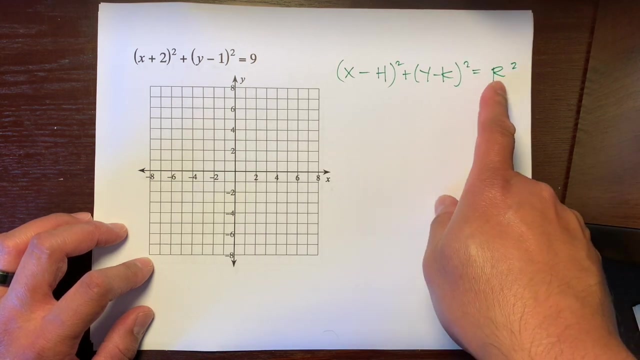 Hello, this is Mr Quinanola and I'm going to show you how to graph a circle given an equation. So in the previous video I showed you how to derive the formula for a circle. and here is the formula for the circle. This r represents the radius and, if you remember, the formula was: